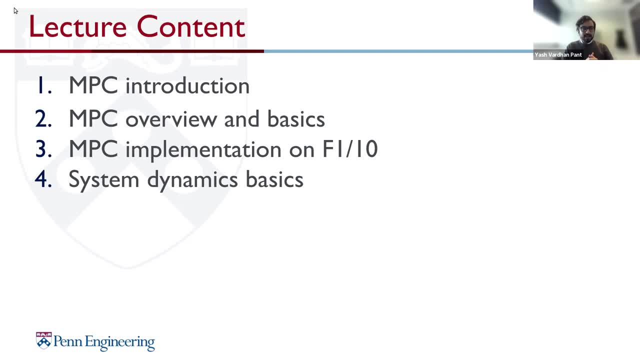 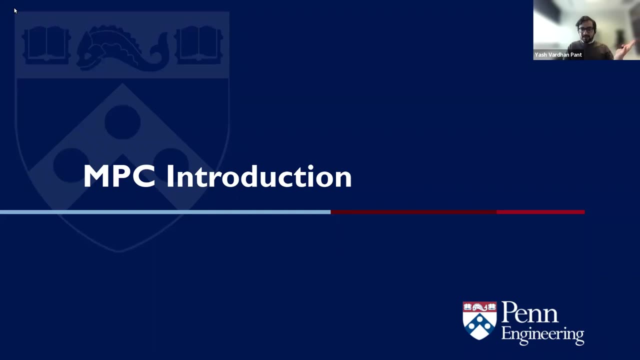 time we have, we'll also talk about some of the basics of system dynamics or the first principle, physics modeling of your race cars. that is useful for using model predictive control, Because the first alphabet in MPC is M for model. Alright, so MPC has a lot of applications, not just in racing, but I guess we'll focus. 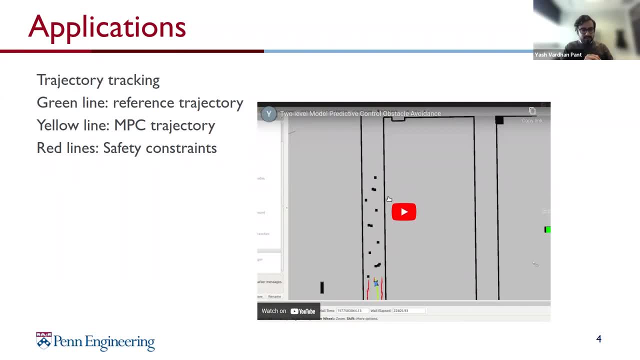 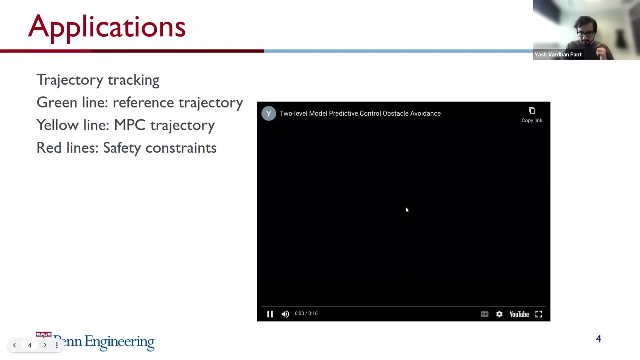 on applications in that particular domain. So we can use MPC for, for example, trajectory tracking. And here's an example of a hierarchical model predictive control algorithm. I'll just play this video. Oops, sorry, let's move on to the next slide. 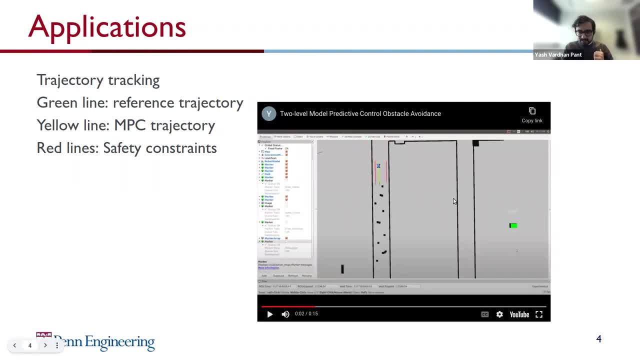 Okay, so you have this autonomous car with a trajectory that is in yellow. That is the actual trajectory that your vehicle is going to follow. In green you have a reference trajectory. Think of that as given by some high-level trajectory planner that tells you this is what the best. 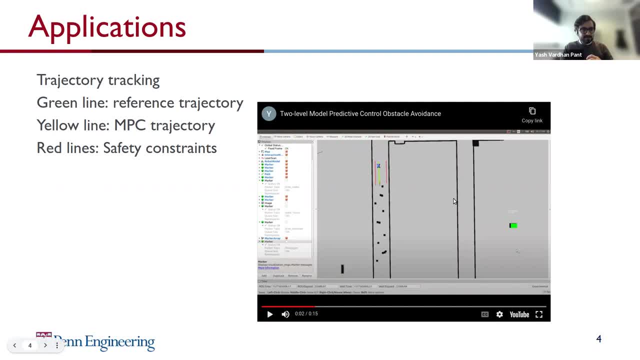 for example, the racing line would look like And the red lines over here are safety constraints generated again online through some algorithm. We'll talk about that towards the end of the lecture- And so the task of the safety constraints is to generate a safety constraint, And so the 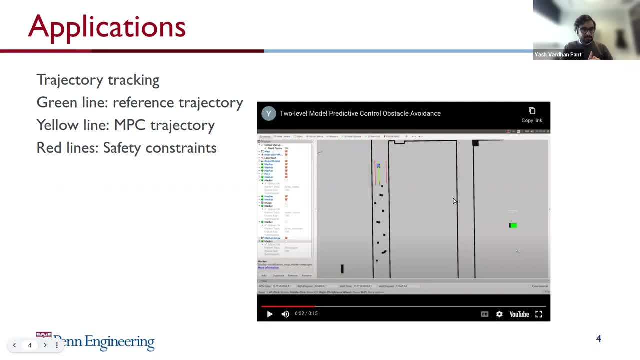 task of this car is to follow the green line, stay within the red lines, that is, avoid obstacles, And then, of course, compute your steering and throttle for the car such that it can do it. And this kind of a problem can be encoded to a model predictive control problem, As 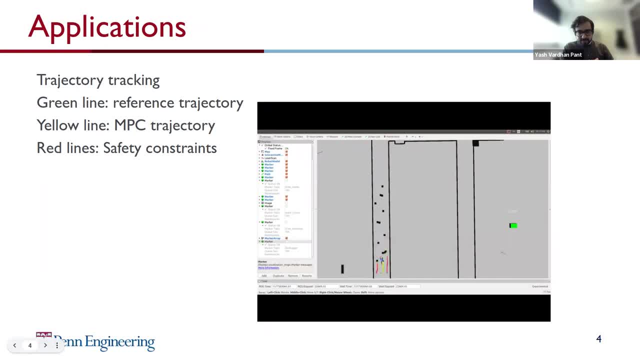 you can see over here, the car makes these drastic maneuvers to avoid these obstacles, makes it through And you have these different red lines which are candidate sets that you should stay within, And so you can use this for racing. I suppose this was being done. 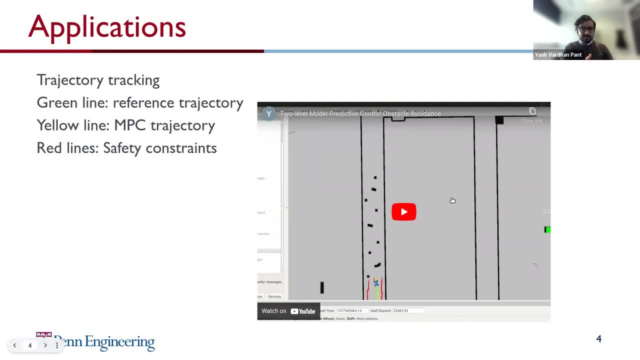 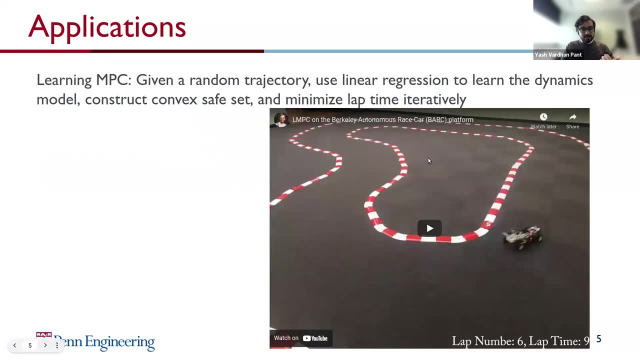 around the Levine corridor, it seems like So- right outside of Rahul's lab. That's one application, So it can be used for trajectory tracking, for example. But over there you need to know the model of the car or you need to know the physics of the car. Now, the modern-day MPC. 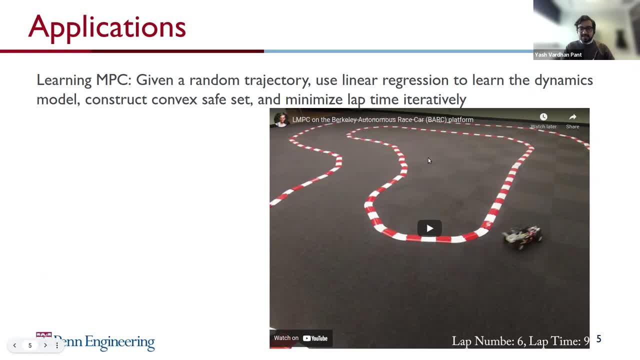 applications where you don't even need to know the model exactly. you can start off with some nominal trajectory, some simplified controller like a PID controller, to just follow a trajectory, And then you can learn over time what the model is and improve. So, for example, 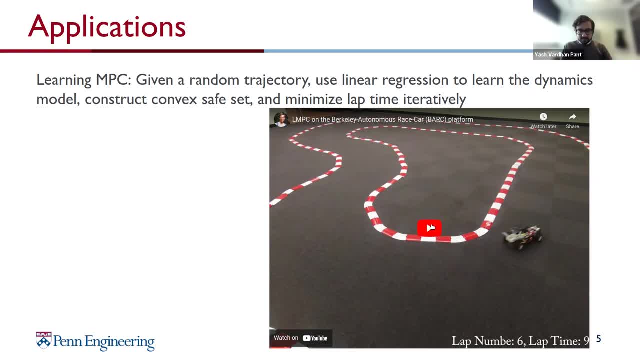 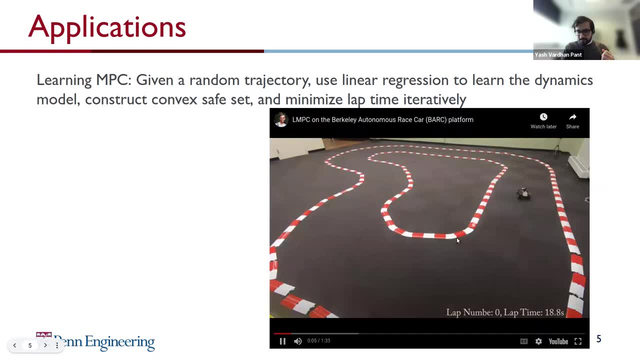 this is an application of learning MPC2 racing done on the Berkeley autonomous race car platform. So we have a car starting off with a very simple trajectory that's slowly going around the track. By the way, quick question: Is the sound being shared or is that something that's not happening? 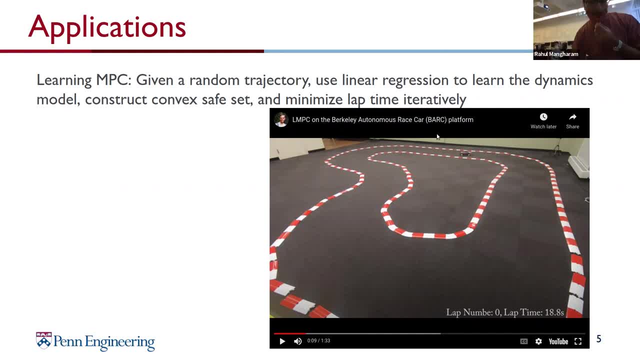 right now. No, there's no sound from the video. Okay, I will share sound because in one of the videos later on I will need sound. So let me know if you can hear this video. All right, So the car starts off slowly, you know, takes a few laps. It started off at about 18. 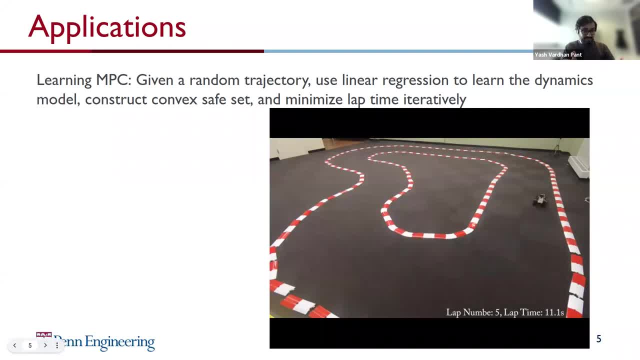 seconds. Now it's driving around. It's learning the track, That is, the constraints on the car. It's also learning the dynamics of the car And as the lap number goes up you can see that lap time comes down. So it's online learning and then using that to control the car to speed it up. 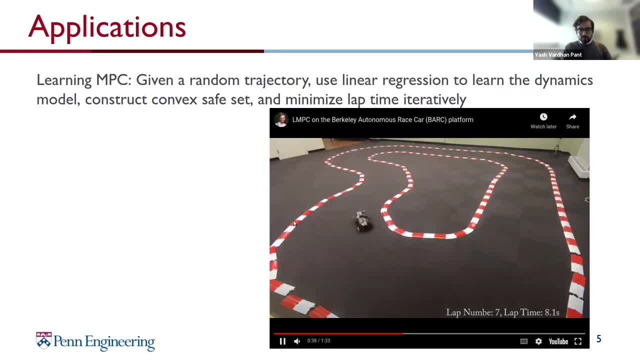 So yeah, this is another application of model predictive control for racing. won't be talking about learning MPC so much. we'll talk about the more classical versions of MPC, where you do know a model and you design the constraints as well, and you don't learn them. 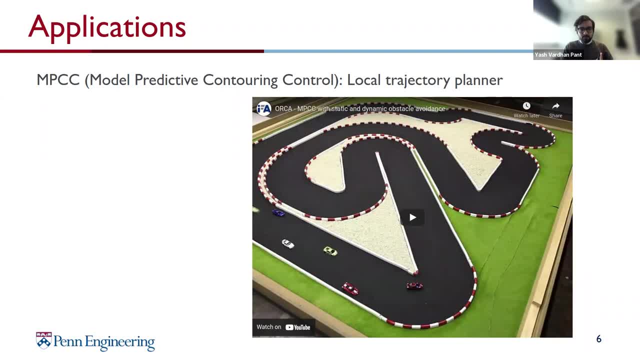 One thing that we will talk about towards the end of this lecture is model predictive contouring control, or using model predictive controller as both a local trajectory planner and a low-level controller combined. So in this case we have these 1 43rd scale race cars called 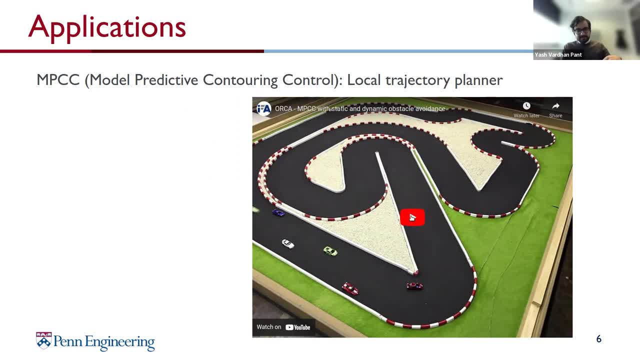 the Orca race car from ETF Zurich. So this is a track- these are RC cars- with the downward facing camera that gives you the position of these cars, also their orientation and velocities, and you have one car that is going to be operating over here in a track with other static obstacles. 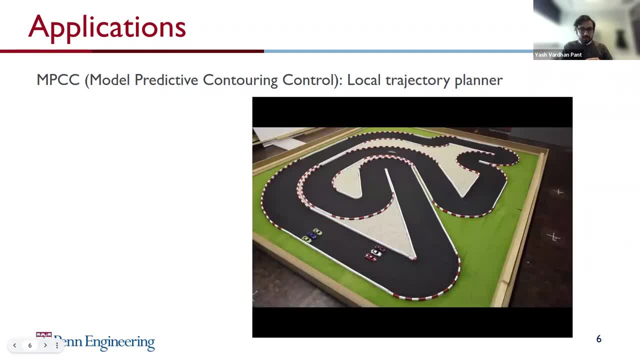 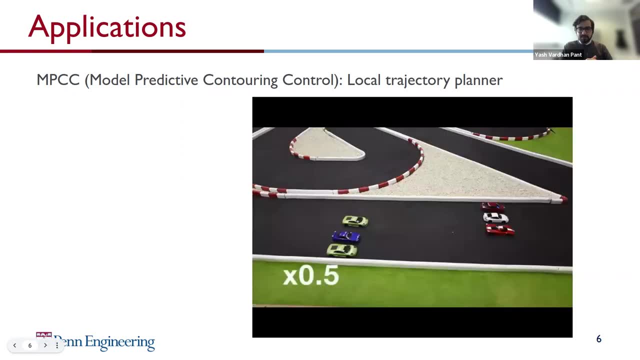 You can see, at these really high speeds they're actually running model predictive contouring control on the inside to generate local trajectories that the car can follow very closely, and it's doing that while avoiding the obstacles, staying within the track and so on. In fact, it's so fast that if you look at this slowed down version, it almost seems like the car. 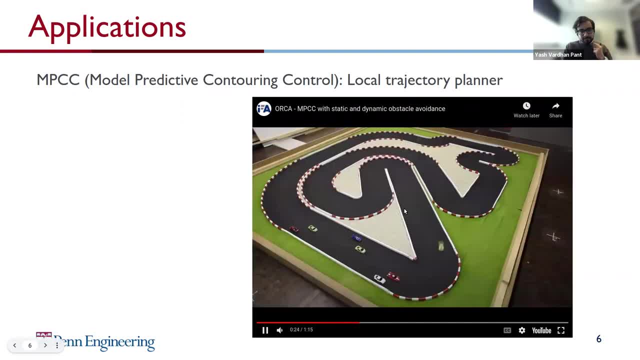 is bending. So, yeah, we'll talk about model predictive controlling, contouring control, at the end of the lecture. But again, this is one more thing that model predictive control can do for you. But if you've taken a controls class like, let's say, 406 or 504,- 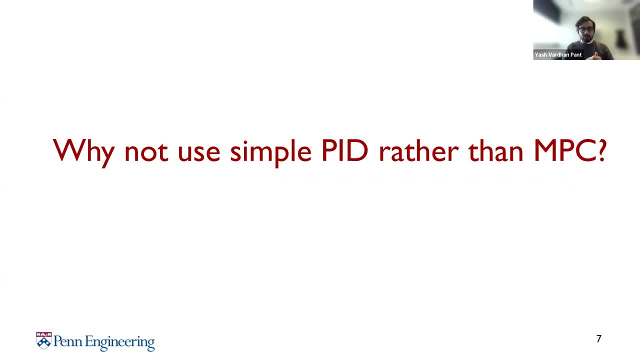 the question would be: we spent so much time talking about PID or lead lag controllers. why don't we just use that for control of the car? And so now we'll try to motivate what we're going to use for control of the car. And so now we'll try to motivate what 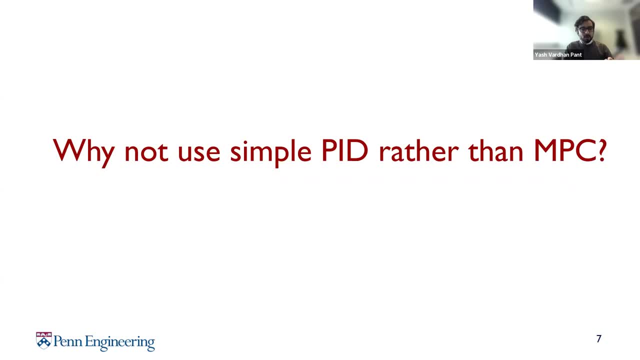 we're going to use for control of the car, And so now we'll try to motivate what you know. MPC, of course you saw it can do some cool things, but it can do things beyond what you could do with a simple PID. The first thing about PID control is that it's usually a single 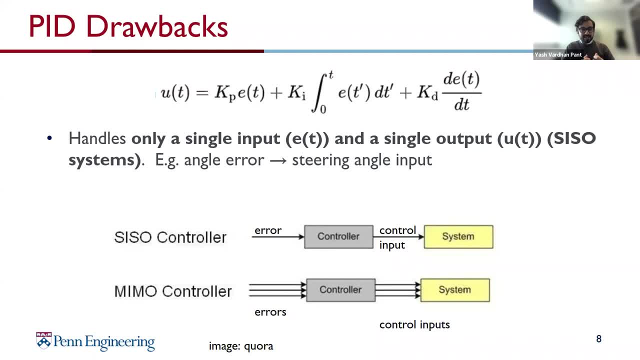 input single output controller. That is, it takes in a single error signal that tells you how far you are from a desired reference and maps it to a single control variable or a single output. For example, taking your heading angle error and mapping it to the steering angle. 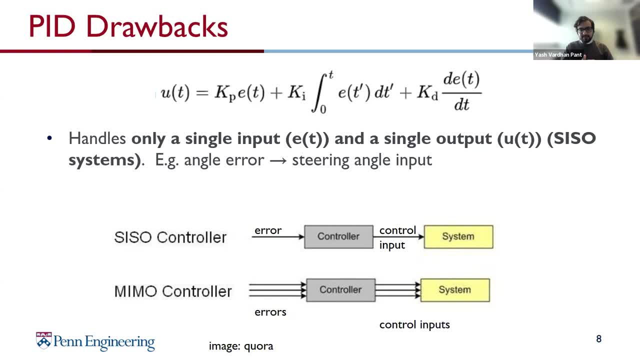 So that would be something that a PID can do for you. Shown on top over here is the control equation for a proportional integral derivative controller. If you have seen it, great. if not, I guess you don't have to worry about it too much in this class. 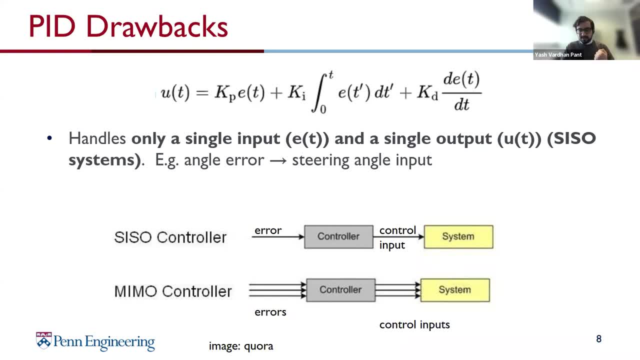 But the kind of systems that you're mostly going to be concerned with, for example, these cars are multi-input, multi-output systems. That is, you have multiple measurements coming from them. you have your angle, you have your velocities, you also have positions and you have to control. 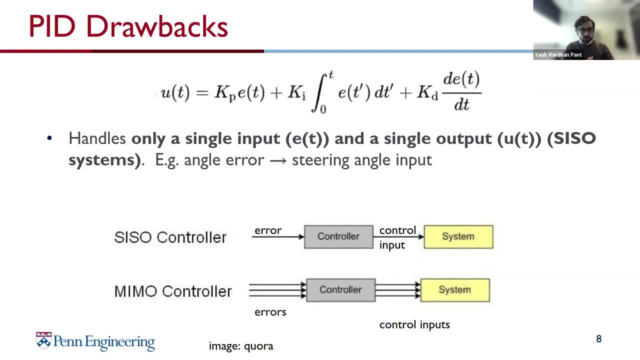 multiple signals. You're not just controlling steering. you're controlling both steering and throttle, and they have to be coordinated. You're not just controlling steering. you're controlling both steering and throttle and they have to be coordinated in the way they're going to act. 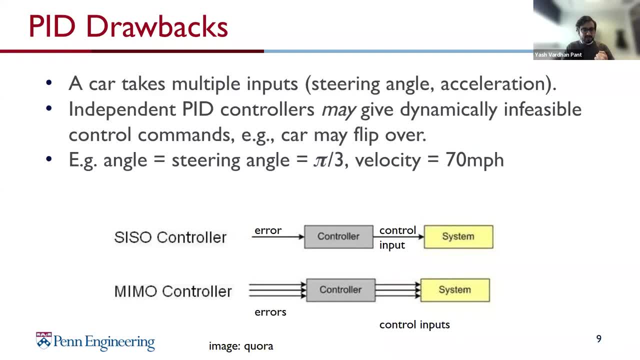 So for these kind of things, PID kind of is usually inadequate. For example, like I said, a car has multiple control inputs- steering angle, throttle, for example- and if you have independent PID controllers that are controlling these inputs without talking to each other, you could come up with the infeasible or bad commands. For example, you might just flip the car over. An example of 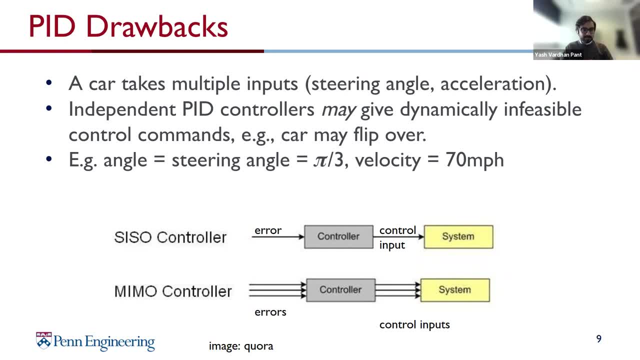 that could be. you're traveling at a high velocity and you give a really high steering angle. The center of gravity of your car is high. then it's going to roll over. So you want to avoid these kind of things and PID doesn't necessarily guarantee that you'll be able to do that. 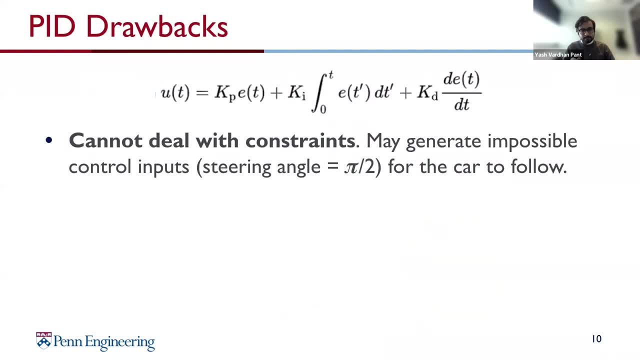 MPC, on the other hand, will try to give you some strong guarantees on what it can do. Speaking of what else MPC can do is that you can explicitly deal with constraints on the system. As we just saw, it was avoiding these static obstacles for staying within the boundaries. 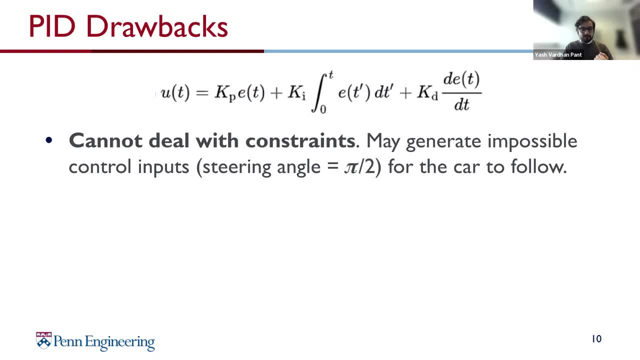 MPC is PID kind of struggles to do that and it could also generate again impossible control inputs- The reason why the equation shown over here. for a large enough error signal and how far away you are from your desired racing line, it could generate a huge steering angle like 90 degrees or even more. 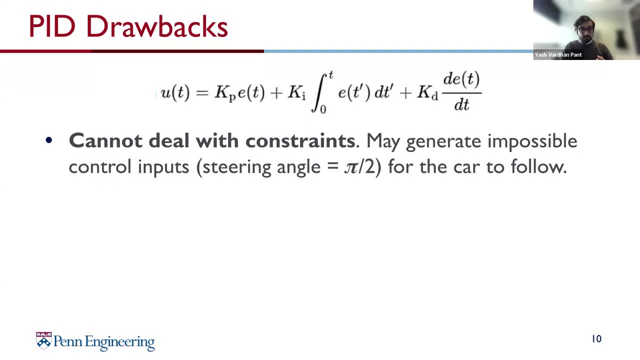 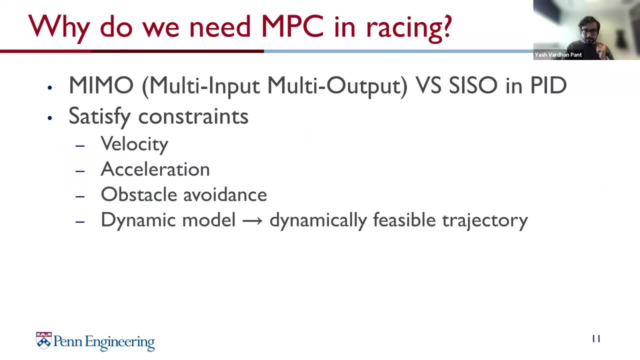 which is physically impossible for the car to do. So model predictive control, on the other hand, has a model, it has constraints and it knows not to do these kind of things. So you know, with that, just to summarize, model predictive control will allow you to deal with. 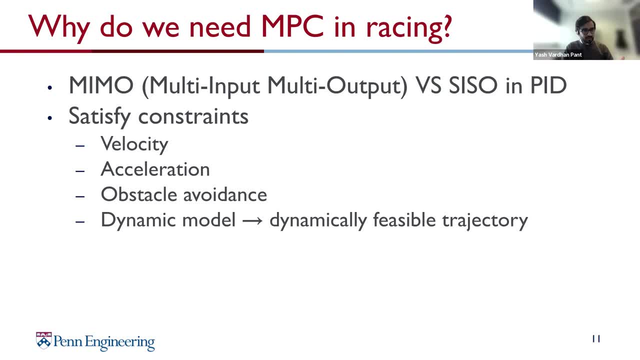 multi-input, multi-output systems in a natural manner, similar to, for example, that will be your race car versus in PID. you have to come up with a lot of hacks to make it work for multi-input, multi-output systems. MPC can also satisfy constraints. for example, you could: 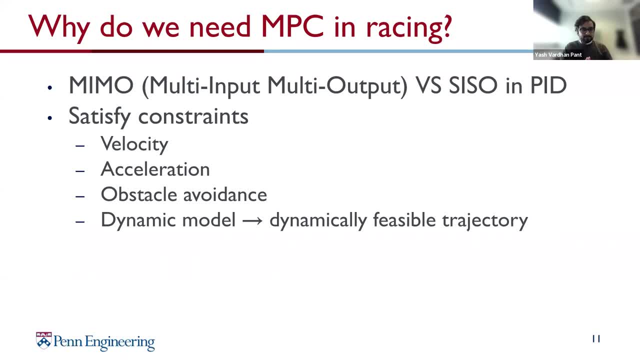 have some limits on velocity, like if you're in the pit lane, your car has physical acceleration bounds, there's obstacles that you want to avoid and, of course, you want to generate trajectories that your car can follow. MPC, as we'll see later on, will allow you to do all of that. 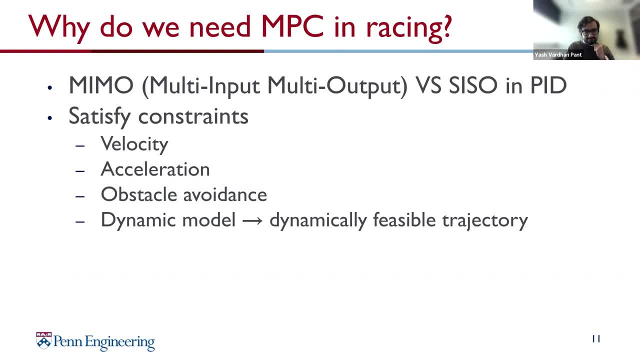 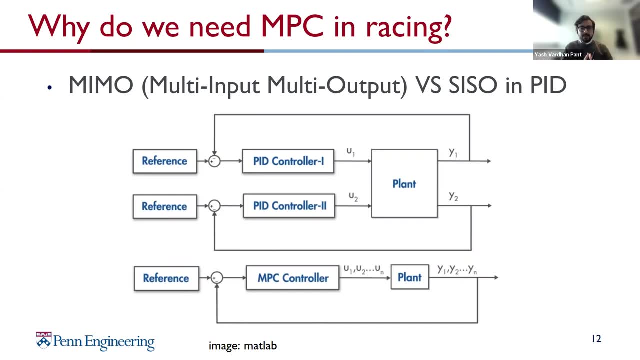 Okay, any questions? so far? I guess not, so let's continue. and right, just to take a look at a picture of what multi-input, multi-output with the PID would look like. you would have to stack up multiple PID controllers, feed them independent error signals for different references, and then you send. 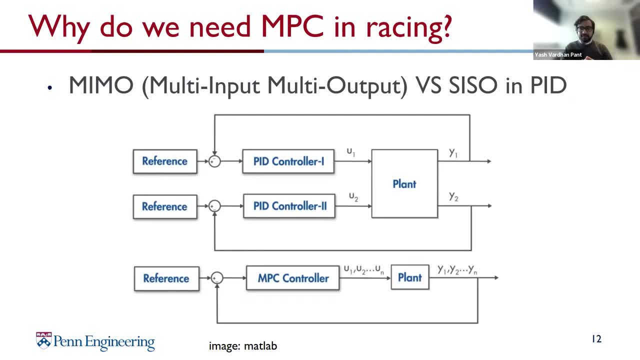 those control signals to your plant, whereby the plant over here we mean the dynamical system. So, for example, think of that as your steering and throttle for the car. you get your outputs and then you try to kind of make them independent in a way that your control PID controller works. 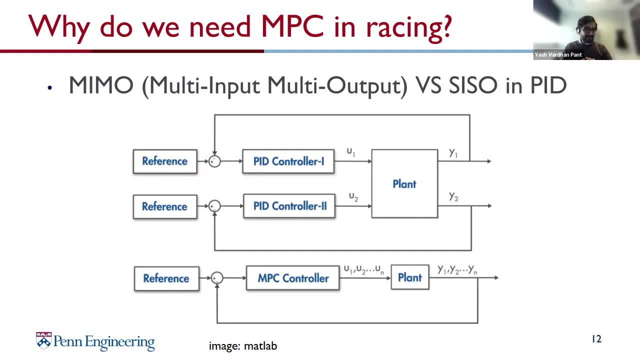 MPC, on the other hand, can take in your multiple outputs or a vector of outputs and also generate a vector of inputs or these multi-inputs to control your car, for example. So, again, this is something that MPC handles in a very natural manner, whereas with PID. 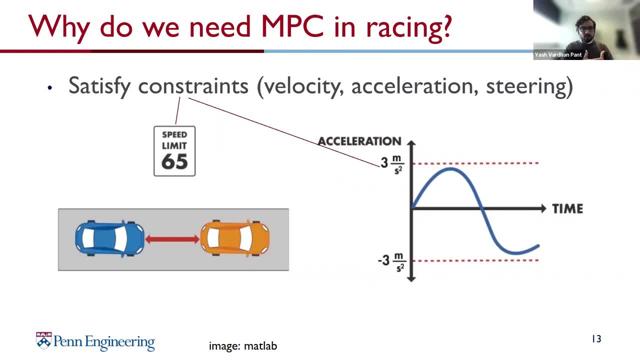 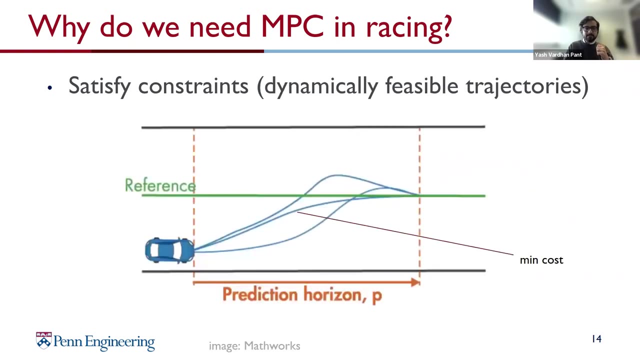 have to hack it. In terms of autonomous driving or racing, MPC is important because you do have a lot of constraints. for example, in driving, you have an explicit speed constraint that you want to respect, you have acceleration bounds, you also have steering constraints, So you can have a lot of. 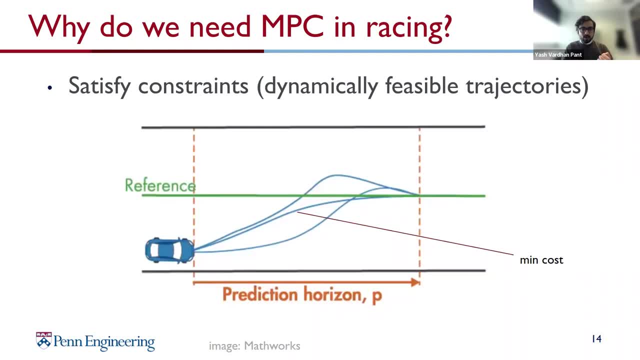 power steering limits on the car that you want to make sure are respected. You also want to generate trajectories. if you're using MPC as a low-level trajectory generator that can be followed by the car, so it can do that for you and, of course, not just generate dynamically feasible trajectories. 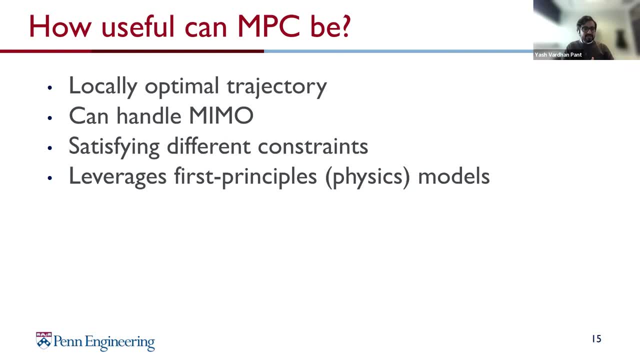 but also trajectories that don't go outside of the track bounds or crash into other obstacles- static obstacles. MPC can allow you to do all that, but as PID, would you need a bunch of hacks to make that happen? MPC gives you these nice properties It'll generate. 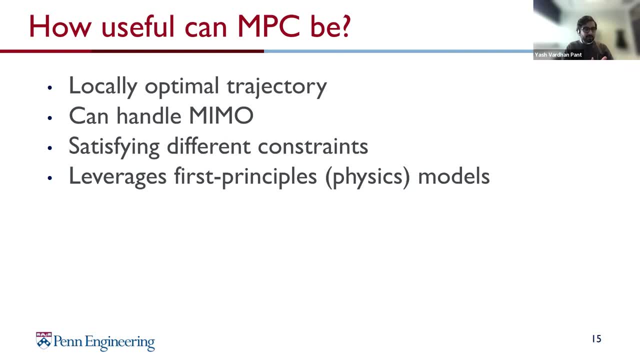 trajectories- if you're using it as a trajectory generator- that are locally optimal. We'll see what that means- optimal with respect to some objective, and we'll see what those objectives are later on. It can naturally handle multi-input, multi-output systems. It can satisfy a bunch of 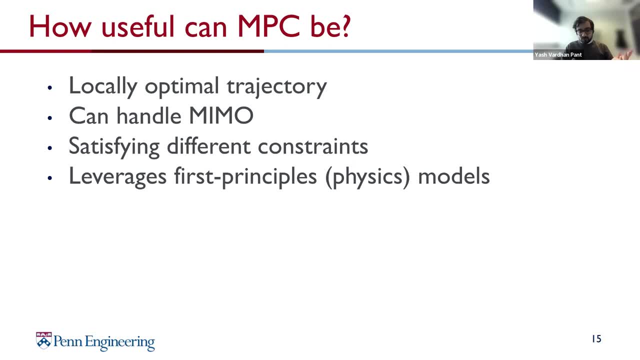 different type of constraints and as opposed to a PID, which is usually agnostic to what's happening inside your dynamical system, your MPC automatically leverages first principles, physics models, and a lot of effort has been put in into coming up with good computational models for cars, for example. 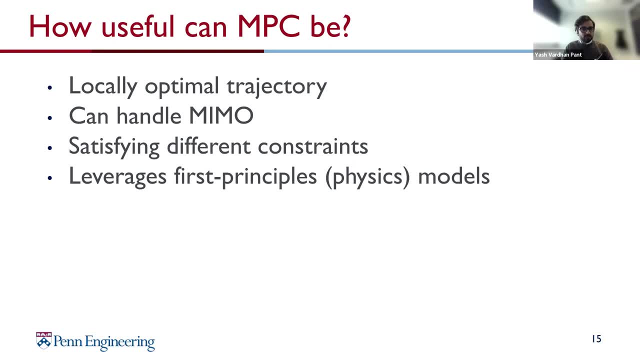 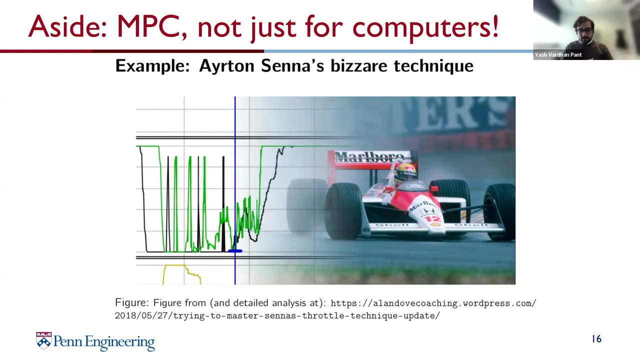 MPC allows you to leverage all that and use it in a way that your control signal is generated using these models to satisfy the constraints while being optimal. So, again, in context of this course, MPC can do these kind of things for you. Now MPC is implemented on. as you'll see, you'll be implementing on computers for autonomous cars. 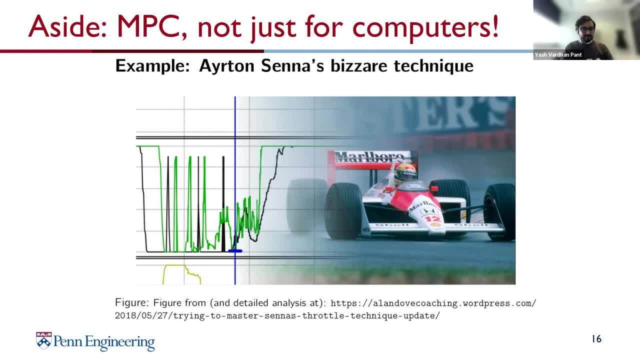 but it's not just for computers. Humans also work in a way very similar to the way model predictive control works, And an example of that from the racing domain is the way Ayrton Senna used to drive, especially his throttle technique, which was noticeably different from that of other drivers of his era. 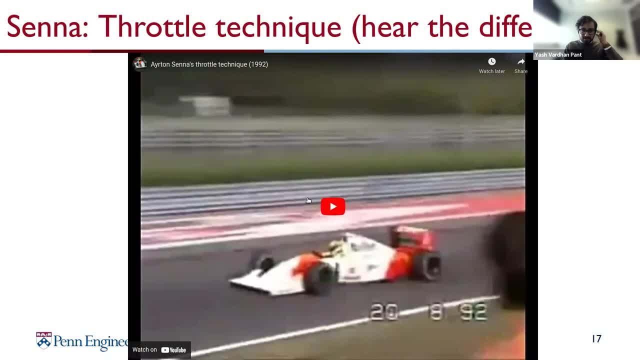 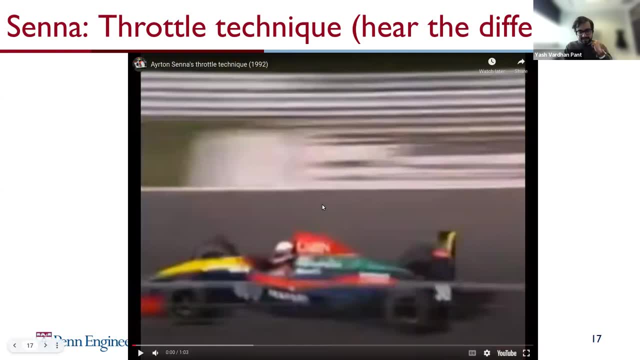 So I'm going to play a video and I'll ask you to pay close attention to the sound of the engine. All right, so first up we have- I think it's a LaRouche, so this is from 1992, so this is a. 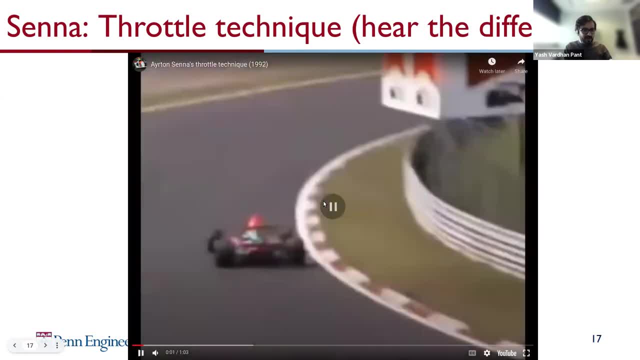 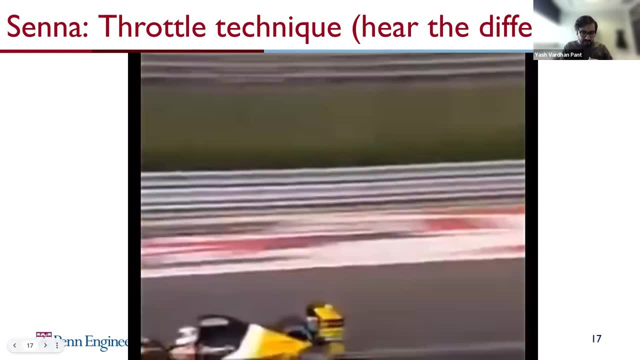 LaRouche, powered by a Lamborghini engine, and listen to how the car sounds. This is how the car goes through the curve and how it accelerates out of the curve. Similarly, we have a Minardi and a Ferrari coming in after that. 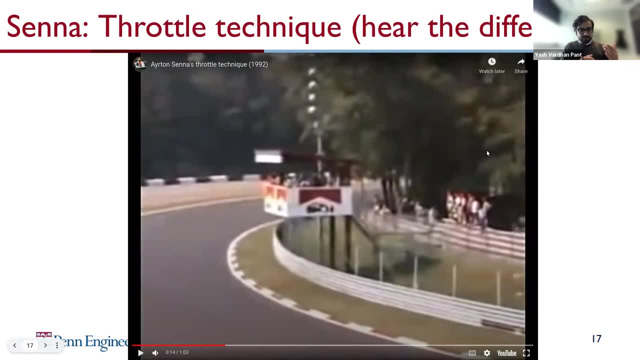 And so what you would have noted over here is that you see the throttle drop out a little bit as they enter the curve because they want to slow down, and then they gradually pick up in the throttle and accelerate out of the curve. So it's a very smooth sounding behavior from 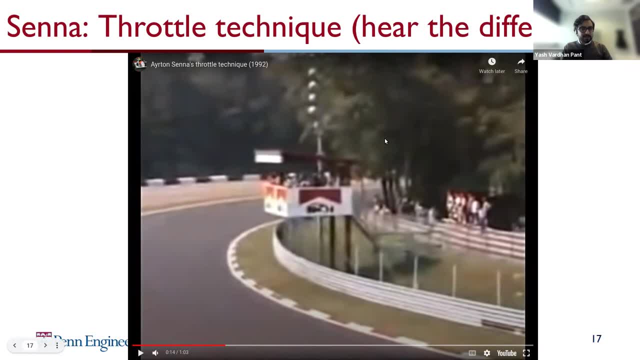 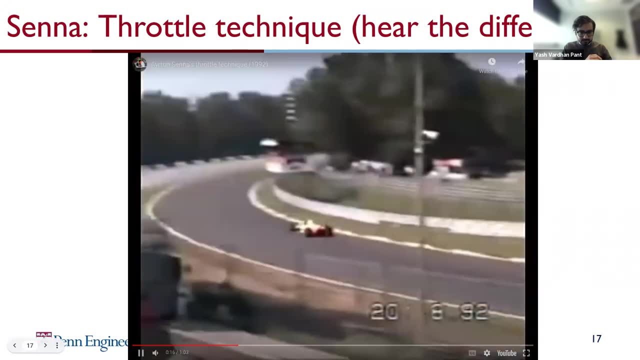 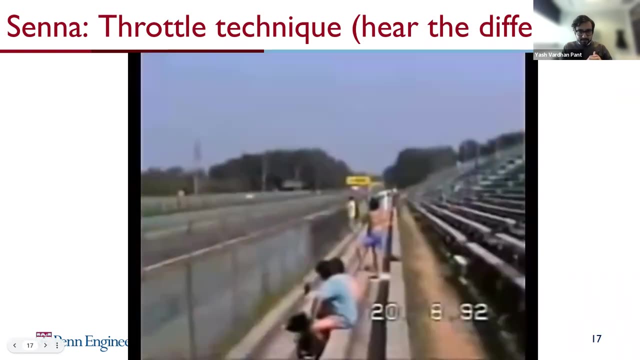 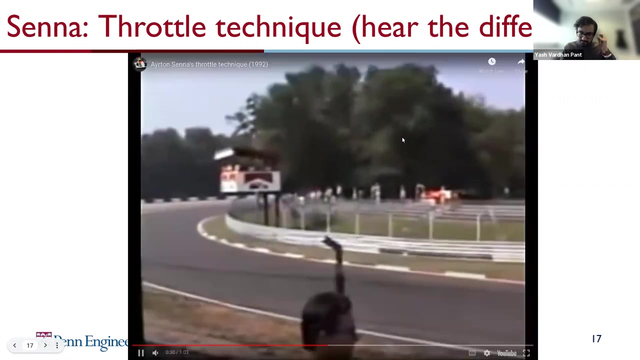 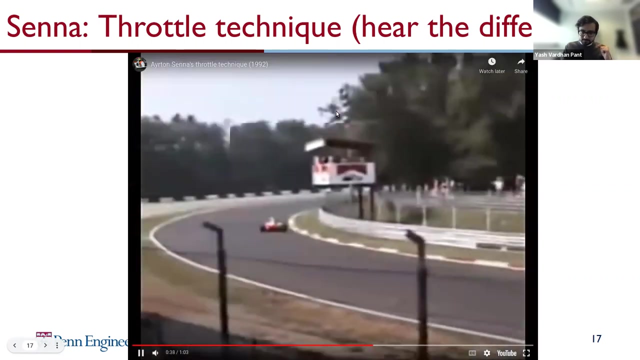 all these three drivers. Now we'll look at the McLaren of Ayrton Senna coming in and pay again. pay close attention to what you hear. That's one example. Let's see Senna drive by again And once more, All right. uh, does anyone want to describe like what they just heard? 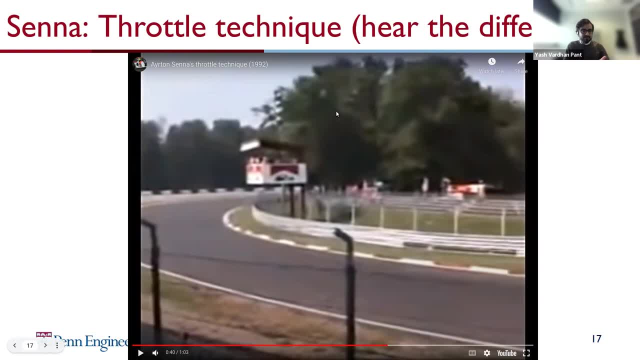 Like, what was the difference between the first three drivers and the way Ayrton Senna was driving around? You can come up here. Uh, he was pressing the throttle, uh, intermittent. Yeah, exactly, He was pulsing on the throttle. He was going on and off with the throttle. 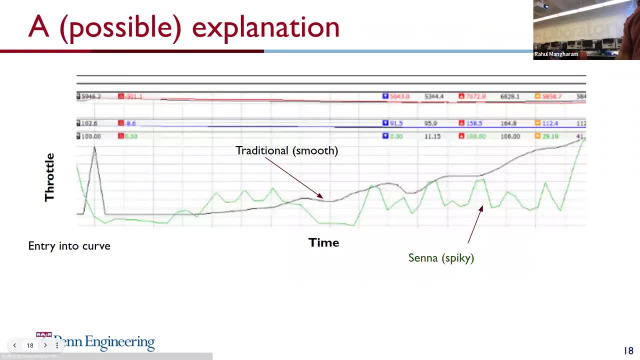 And oh sorry, let's get to the next slide. All right, and that's kind of shown in this particular um figure over here. This is some data that um- I'll give a reference to it- um just plotted by someone. So it's the throttle over here versus time In black, you have a traditional throttle. 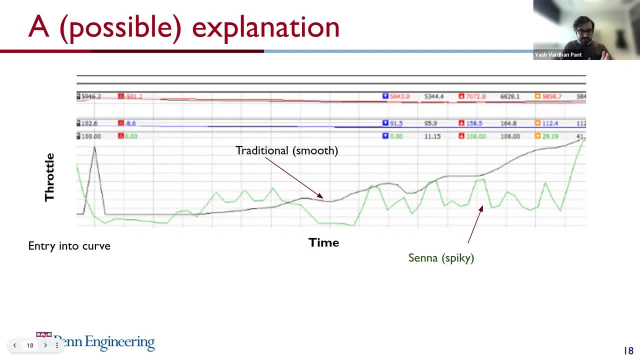 On the left-hand side, of course, your x-axis is time, y-axis is throttle. Your leftmost point is your entry point into the curve. So you see that the traditional both Senna, um, they drop the throttle. So you see the throttle go down. 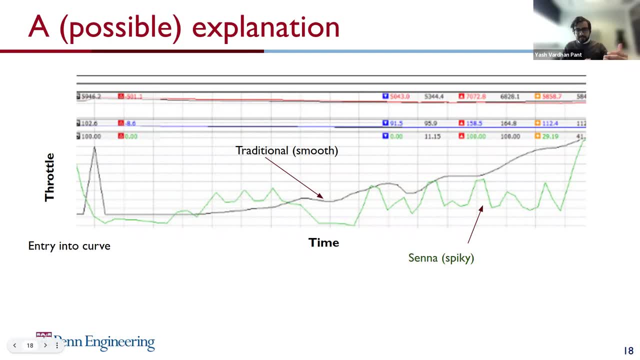 And then for the other drivers, they are gradually smoothing- uh, they're smoothly increasing the throttle as they come out of the curve. Senna, on the other hand, as you heard, was going up and on and off with the throttle, So it has the spiky behavior that results in these. 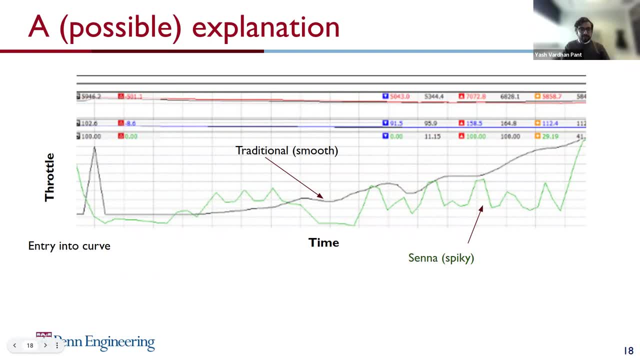 pulses of sound And the reason why Senna might have been doing this again. this is just one possible explanation. There's a couple of them. There's a couple of them, Um, one is to that he was trying to compensate for turbocharger lag. 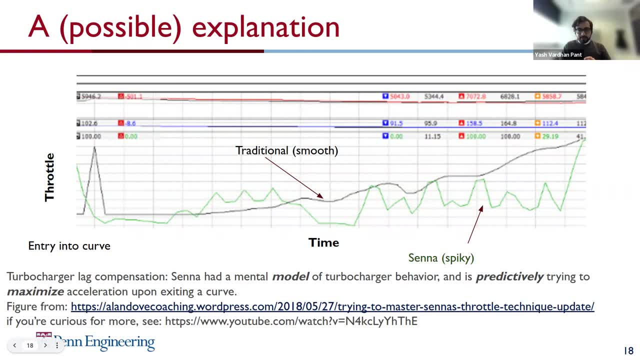 So Senna started racing um, I guess in the 70s, back when a lot of these cars were powered by turbocharged engines. Turbochargers back in the day took some time to spool up. So if you went full throttle you would have this noticeable um fraction of a second lag before the engine would. 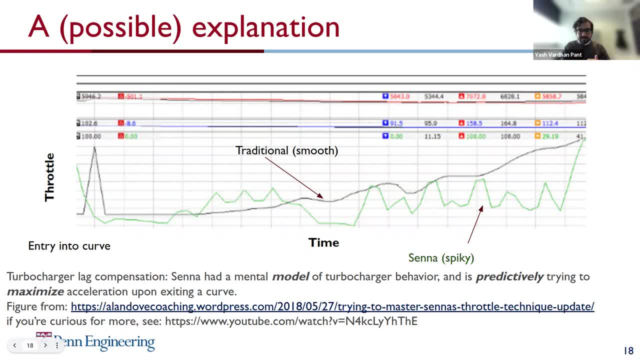 actually spoo-, the turbo would spool up and you would get maximum acceleration from the car. What Ayrton Senna is doing over here is that he has a mental model of the turbocharger behavior. Because of that model and the spiky um uh throttling that he's doing, he's actually keeping. 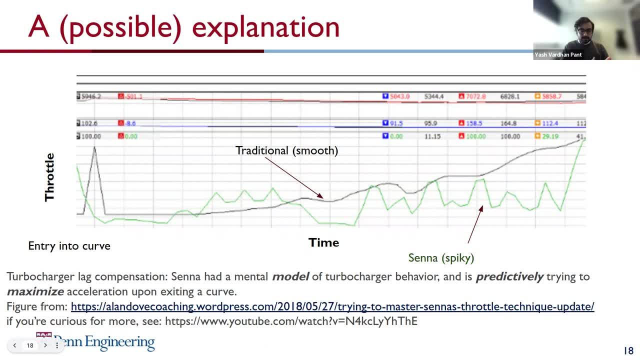 the turbocharger spooled up because it depends on the rate of your throttle And because he's keeping the turbocharger spooled up, he's predictively. you know he's thinking ahead. He's thinking about what should I do at the end of the curve. So by the end of the curve he's trying to maximize acceleration. 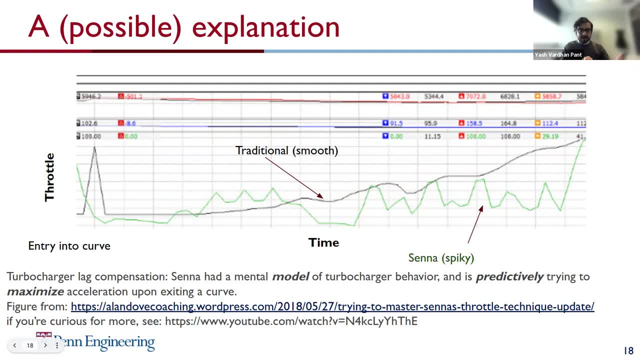 and come out of the curve faster than anyone else, Which is kind of why Ayrton Senna was so good in the early 80s driving mediocre cars and he was competing with the top drivers Because he one of the things was in addition to his natural talent that you know he could. 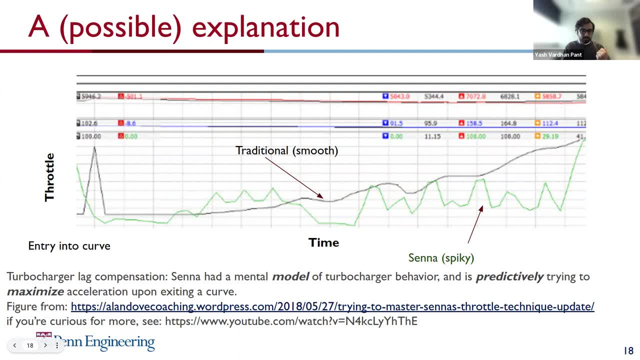 he was very fast exiting the curves due to anticipating turbocharger lag. Now there are a couple of references over here. if you want to take more um, if you want to take a deeper look into what's going on, I'll share the link of the slides with Rahul and he can share that with you. 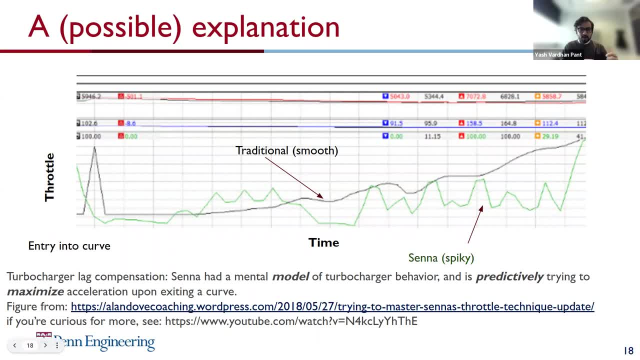 later on. But again, what he's doing over here is he has a model and he's predictively trying to optimize something, Which is exactly what model predictive control does as well: Uses a model and some look ahead, tries to optimize for some objective function. So with that let's move on to 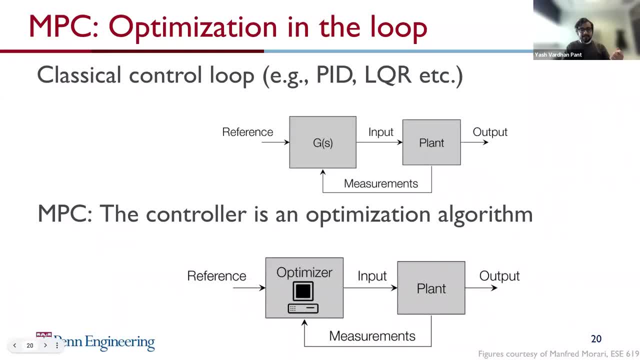 what MPC is trying to do. So again, like I said, the MPC can be thought of as an optimization algorithm in your closed loop that is going to be computing your control input for you, As opposed to classical control like PID or a linear quadratic regulator, which is a fixed mathematical function but takes 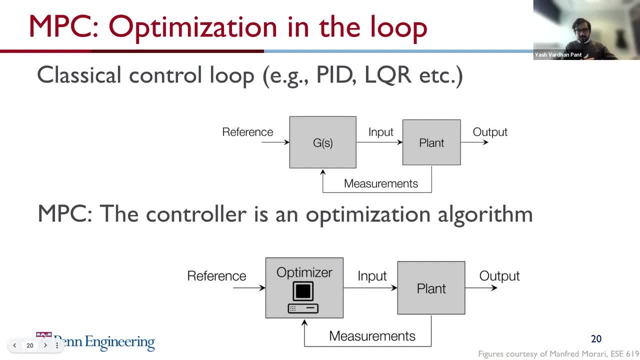 in a reference, takes in the measurement, computes the error, gives you the input to the system. But MPC always is going to take in the reference, take in the measurement and it has a model of your plant or a model of your dynamical system, just like Ayrton Senna is thinking about turbocharger lag. 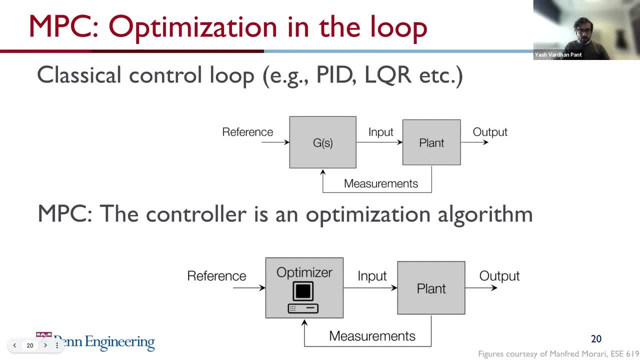 And now, instead of planning, computing a control input that is just optimal, now, you're trying to compute an input that is going to be optimal over some time horizon. I think, just like Ayrton Senna, he's looking to the end of the curve. MPC will be looking at some. 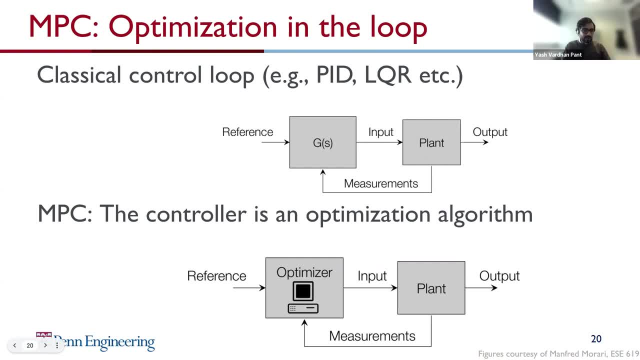 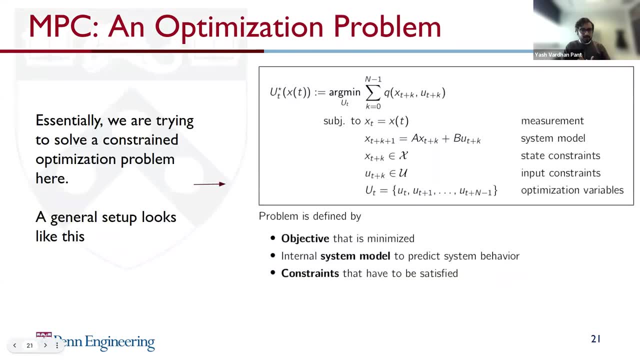 moving time window to optimize over. So again, the MPC, as opposed to your classical controllers, is a, an optimization algorithm in the loop. The question is, what is that optimization algorithm then? And essentially, we try to solve the constrained optimization problem with the very general form of that shown over here. So you're trying to, um, given your current state, 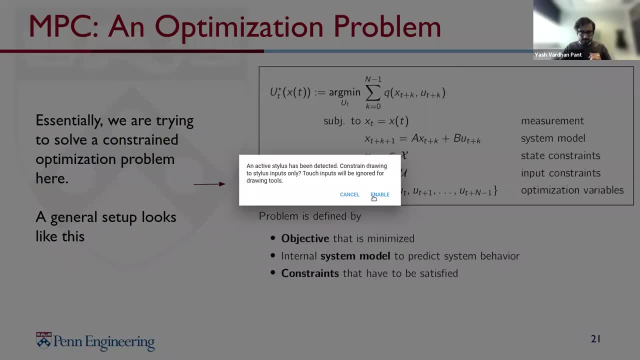 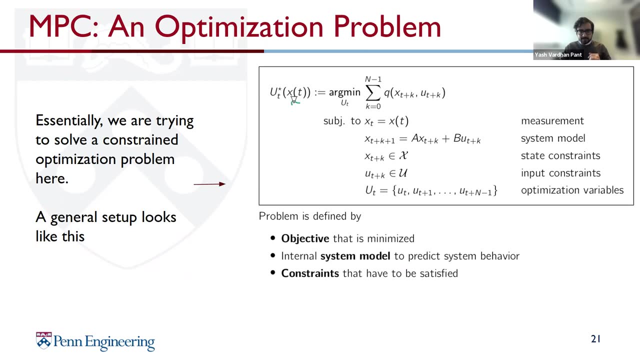 of the system. oops, Okay, I'm just going to try to see if I can do some annotations over here. All right, so this is the current state of the system x of t and you're trying to find a sequence of control signals u of t that minimize a given. 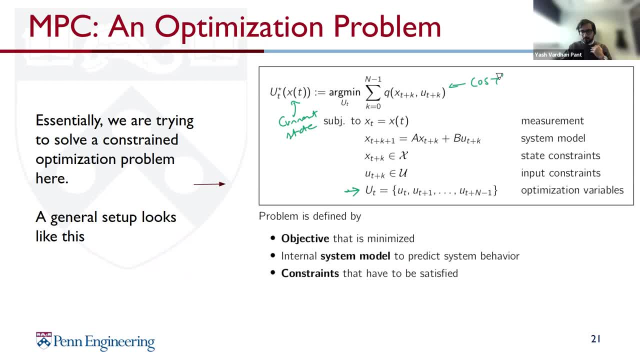 cost function. so this over here is your cost or your objective to be minimized. we'll take a look at some mathematical forms for this later on. you're doing this starting off with your measurement. so this is your starting point: that you start off with your initial state and you're using a system. 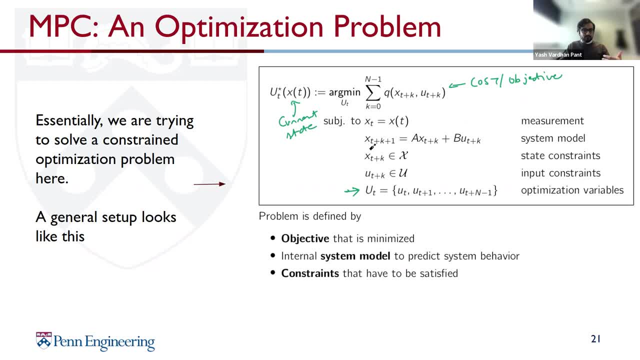 model. so the evolution of the state and time. so for k plus one time steps ahead of your current time. now the evolution is going to be given by some system model. mpc mostly uses linear dynamics on the inside for computational tractability, as we'll see in the next few slides, let's assume. for 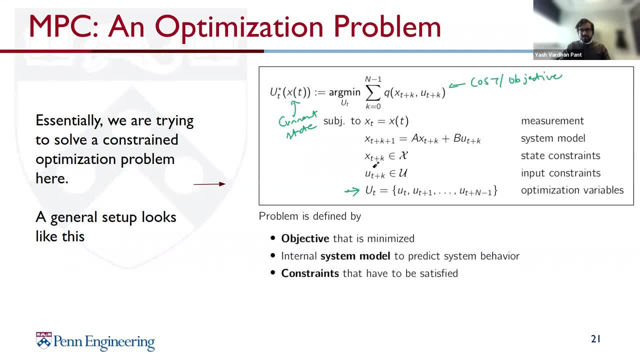 now, this is the kind of a model that we're interested in. it's going to take in constraints on the state of the system. state of the system could be the position, velocity, orientation of your car. takes in constraints on the input. it could be throttle and steering constraints and again it has these optimization variables to take into account. 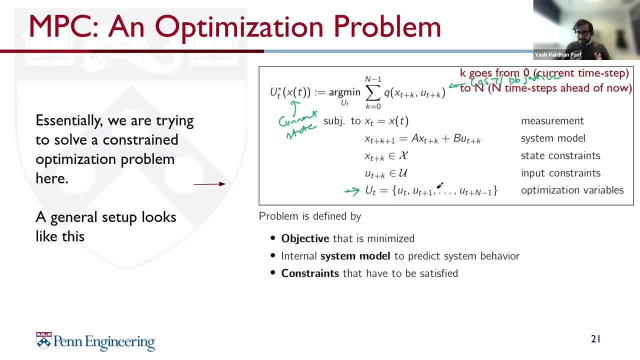 so the problem for mpc? oh yeah, these constraints are not just for your current time step, but this k increments from zero going all the way to n, where zero is your current time step and n defines some time window for you. so if you're discretizing your system at a sampling time, dt, n times, dt is. 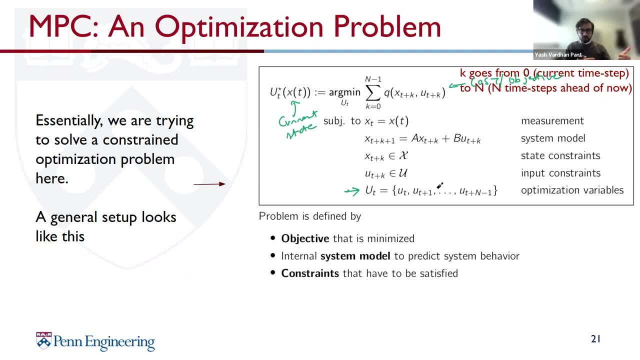 going to be how many seconds ahead your optimization is thinking, or what we call the horizon of a model predictive control. so the problem is then defined by an objective that you're trying to minimize could correspond to lap time or tracking error for a given trajectory, and so on. you have an 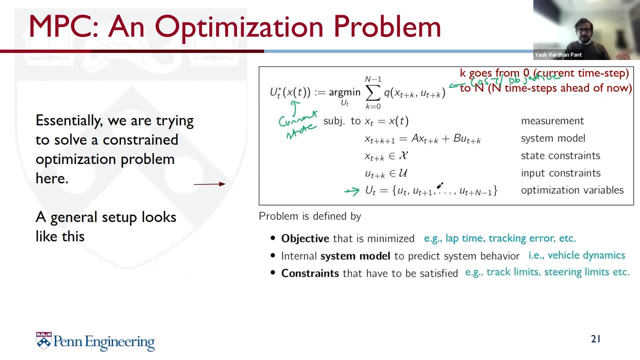 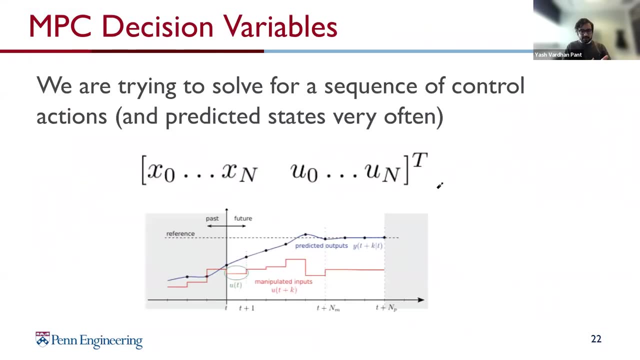 internal system model for your vehicle dynamics, and then you have constraints on the track, steering limits, etc. so let's briefly take a look at what kind of decision variables we are computing for mpc and through this minima. what are we getting through this minimization? all right? so usually we 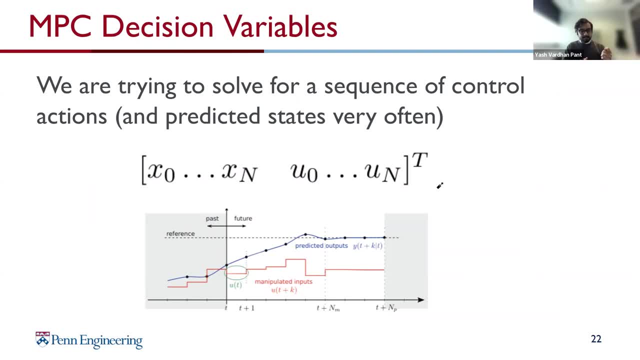 try to solve for a sequence of control actions, or let's say, you know, i'd say pairs of acceleration and throttle at each time step, starting from now to some end time steps ahead. and also you could solve for your state predictions from now till the end of your time horizon, and that's what mpc is going to give. 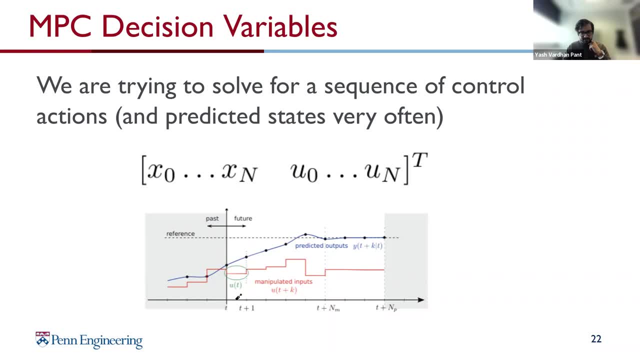 you as an output, and what you see over here is, for example, starting at time t, you compute your control signals, going all the way from p to t plus np, which is, let's say, your prediction horizon, and you get some predicted states or predicted outputs, shown through the blue line, that is. 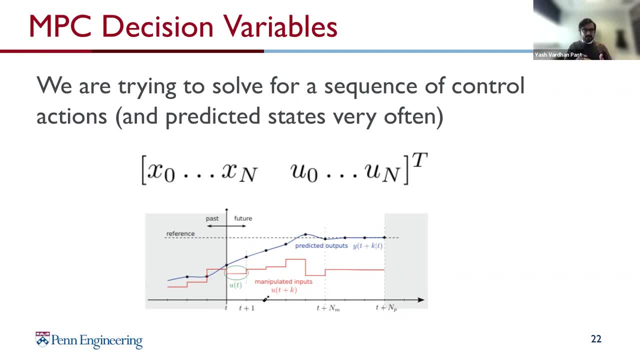 trying to track a reference: what you have done through solving the mpc optimization. you know again. we'll see in detail what the components of the mpc optimization are. but let's say someone gives that to you and you solve it is you've computed an open loop sequence of controls. 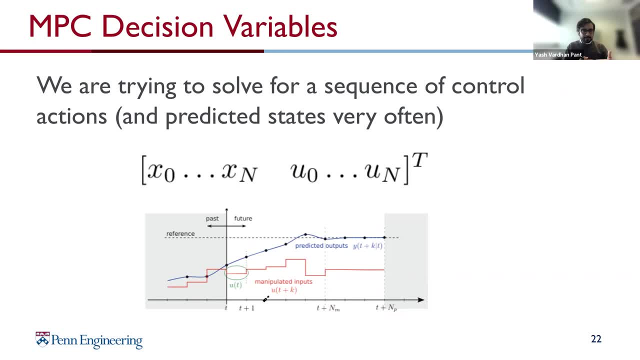 by open loop we mean we haven't applied them to the plant yet. your dynamics could be different. they could be different from the one that you're using in the model. there could be noise in the system. so your closed loop behavior, when you apply these signals, might be different from what you're predicting in an open loop manner. so the first: 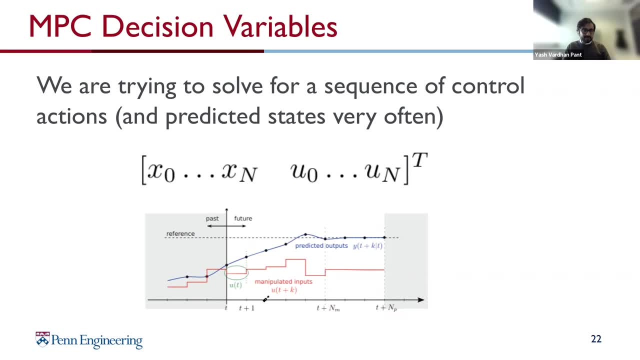 thing is, mpc is, to begin with, an open loop optimization, and you've predicted, you've essentially computed your controls from time step now till some end of the horizon, capital n. the next question, then, is: how do we use this for closed loop control? because that's what we 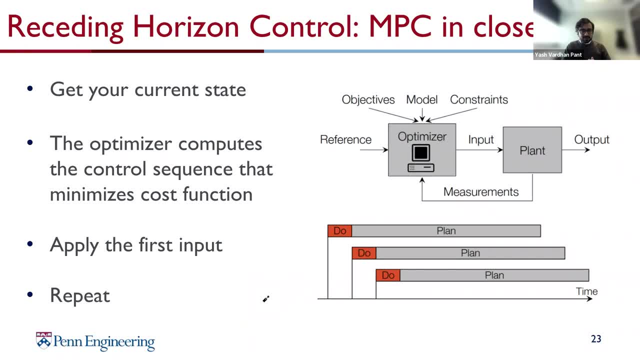 want to do, and for that we're going to use this thing called receding horizon control, which is essentially an algorithm to use mpc in closed loop. it's a very simple idea: you start by taking in your current state or your measurement at time. step t, let's say you start off. 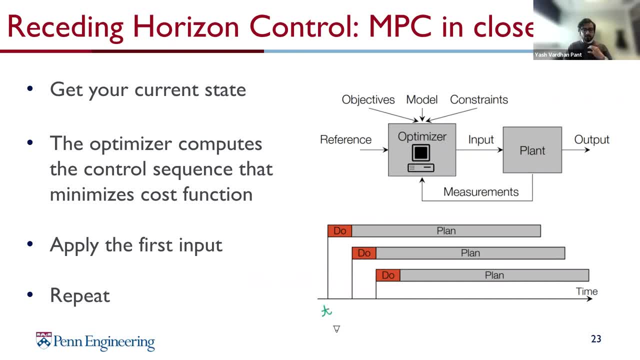 time step t, which is over here, and you compute your control sequence all the way from time step t to t plus n. so let's say this point of time is t plus n or the end of your horizon. the optimizer is going to give you what this 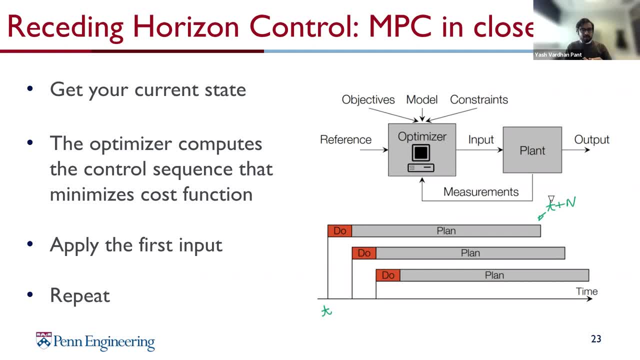 optimal sequence is what you're going to do is you're going to apply your first control input. so, for example, you apply what your first acceleration and throttle is. that is the stage over here, written by. do so, that's your apply the first control input, and then you repeat. 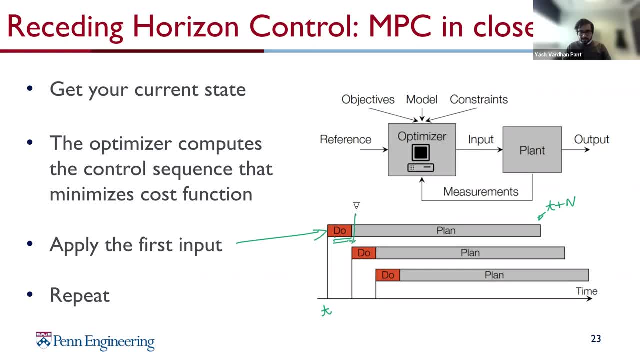 the process. you get another state estimate, which is over here. you get a measurement at time step t plus one. you now solve your optimization again with the n step. look ahead. so now, instead of solving t plus n, you solve to t plus n plus one. apply your first control input. repeat the process. 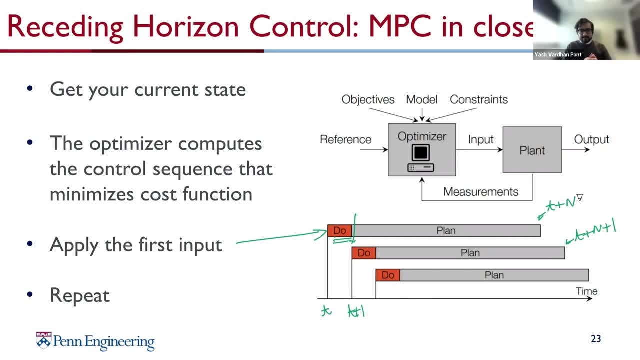 and repeat and so on until the end of your event. so in this way, what we have done is we have taken our open loop optimization and turned it into a closed loop controller by taking in the measurement and then accounting for the measurement, because your state could have moved. 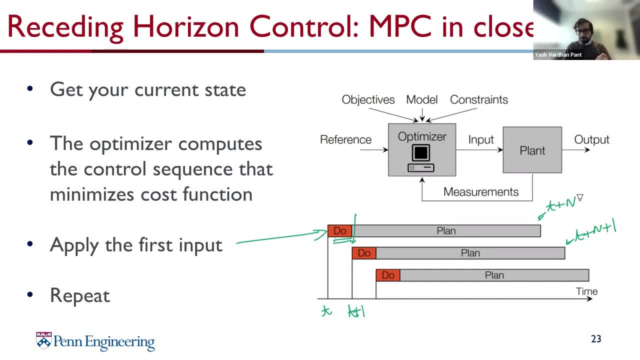 more than what your prediction was saying it was going to. and we call this a receding horizon approach because if you sit at time t and you look at where the horizon of your npc is, it's going to go further and further away from you as time progresses. so we call this the receding 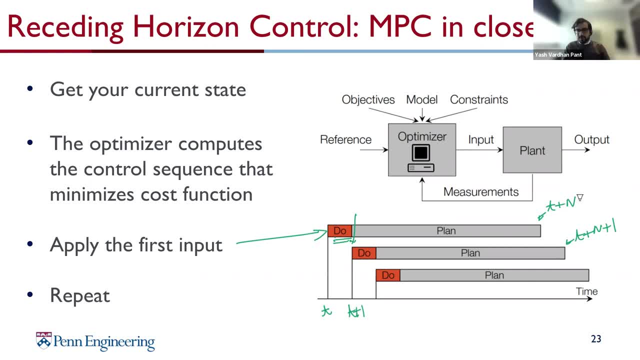 horizon approach. anyway, this is how you're going to be applying npc in a closed loop manner. um, any questions so far before we get into some more details. yeah, there's a question. cool, so you're assuming here that we do have the control input at time? at time, t equals zero. right for me to uh use that here, but since it's an optimization problem, 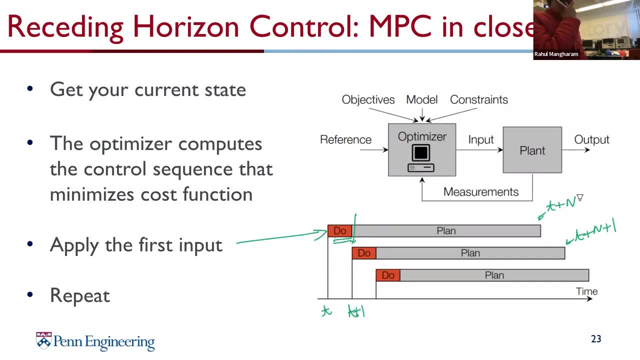 won't it take me some time for me to get the control input itself? so how do i do the do action without me performing the optimization? that's a good question point. so right now we are assuming there is no um computation delay, and so let's say you start. 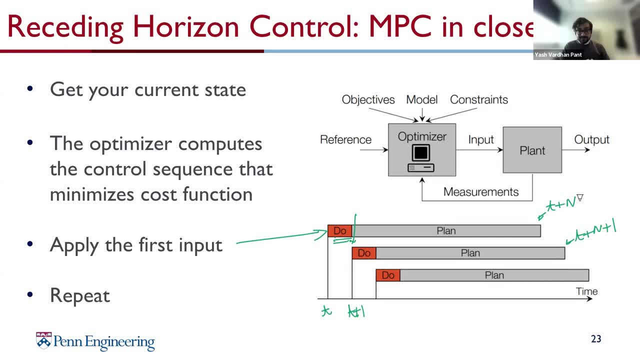 off for time zero. you can instantaneously compute a control. you're right, there are usually some delays, and but you know again, you can solve npc in a fast enough manner, as you'll see later on, that those delays won't practically matter, if you do want to take them into account. there are. 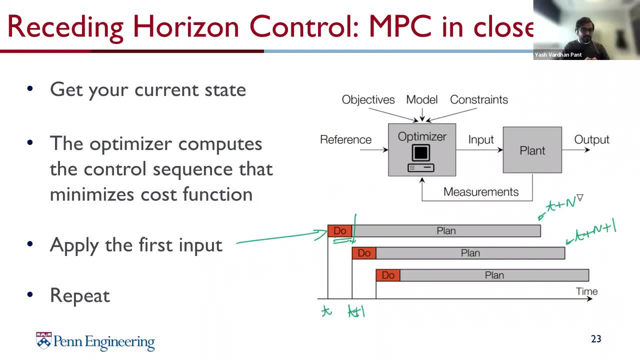 modeling tricks that will let you account for that delay as well. but for now, just think that the computation is fast enough that you don't really need to bother about the computation view delay. but yeah, that's a very good question, thank you. thanks, you solve it, for, like you know, 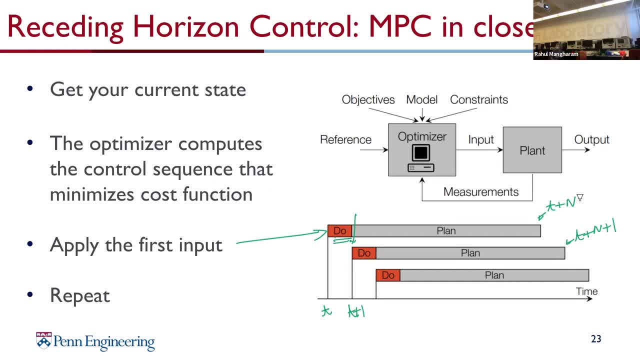 you can solve it at 50 cycles, 50 hertz, and that's fast enough. yeah, absolutely yeah, you can. depending on your system, you can solve it at tens of hertz, which should be enough, and maybe at the end i'll show you a slide that you can also do npc for nanosecond rate updates, if you have to. 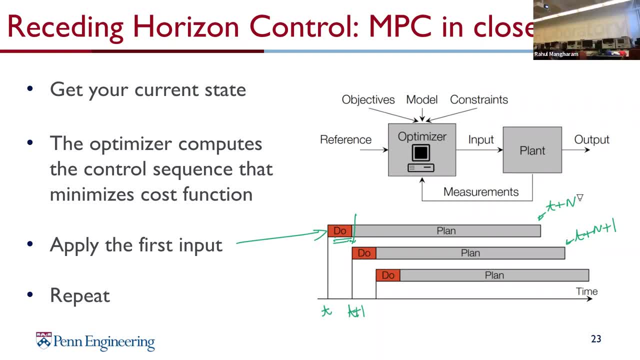 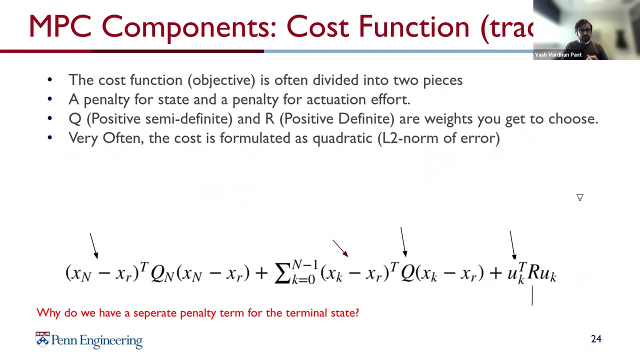 for certain kinds of systems. any other, yeah, all right. all right, um, now let's move on then. so yeah, so npc is an optimization. it gives you an open loop sequence of control signals to be applied and you can apply them in closed loop by doing this receding horizon method. all right, now let's take a deeper look into each of the 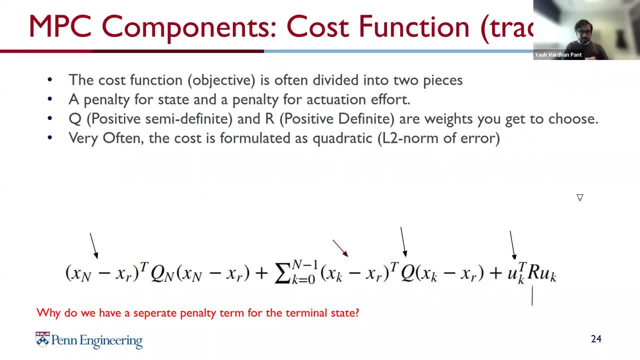 components of npc. first is your objective function that you're trying to minimize. we call it a cost function or an objective. divide it into two parts. first part- actually let me go one by one- is a penalty for your how much your state is deviating from a given reference. so x of k over here is your state at time. step k: 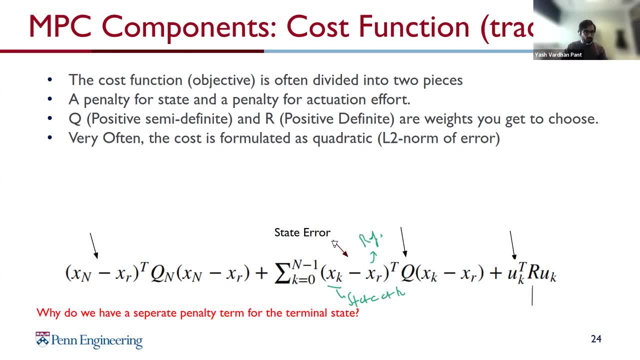 and xr is your reference or your desired state that you want to be at. think of it as, say, you're tracking a trajectory. so this could be a sequence of positions and velocities. so you have a state error and then you have a penalty matrix for the state error. so q over here. 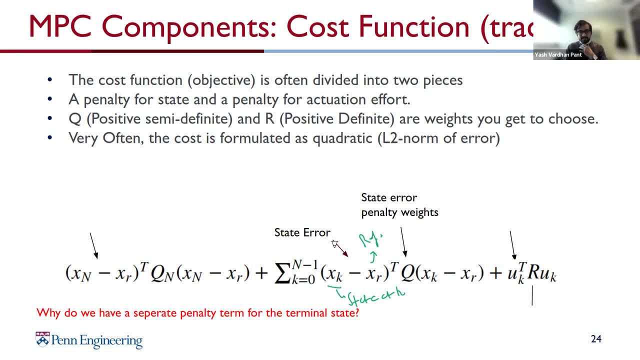 is a positive semi-definite matrix. positive semi-definite means that its eigen values are greater than equal to zero. this is one design restriction: that your matrices have to be positive, semi-definite or positive definite, and that gives you a quadratic penalty over your state error for. 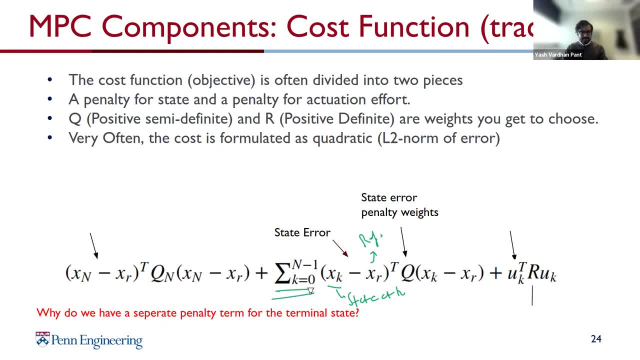 your entire horizon. so you see this sum. this sum is going from time step 0, which is where you are right now, to time step n minus 1, which is the end of your horizon. similarly, you also have a penalty term for and rk with n for times e, n, 1 and s for n minus 7, which is the end of your horizon. similarly, you also have a penalty term for. 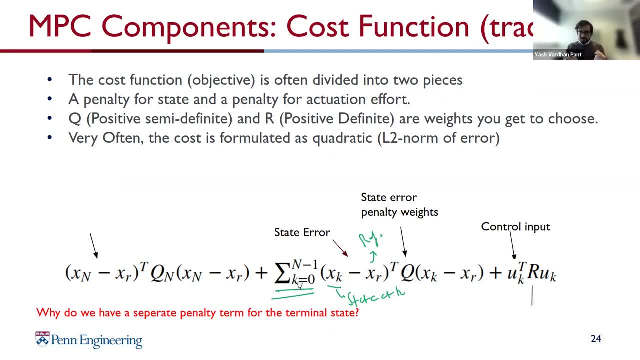 how much control effort you're putting in. for example, if you're doing a lot of steering or if you're applying a lot of throttle, you kind of want to penalize that as well. so you can penalize that through a quadratic term on u, which is your control input, um r over here is your weight. 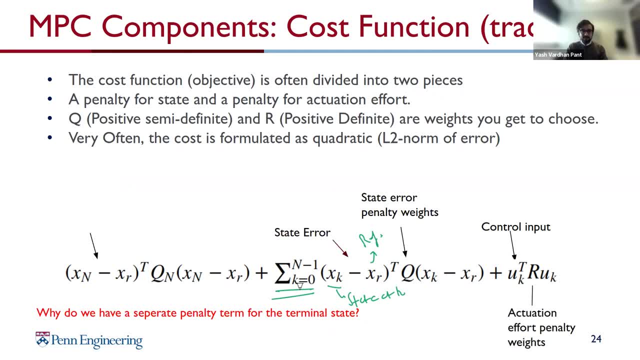 again, and this weight matrix has to be positive, definite, that is. all eigenvalues have to be greater than zero, which essentially means you should penalize all your control inputs a little bit. you can't have any control input that is not penalized otherwise, at least numerical. 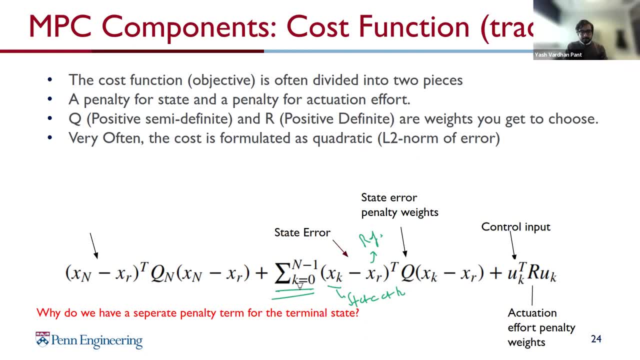 instabilities and also you lose a bunch of guarantees. um, finally, you also have a terminal state error or a cost for the state that you get at the end of your mpc horizon when you're doing things in open loop. um, i guess the question over here is: why do we need to have it? 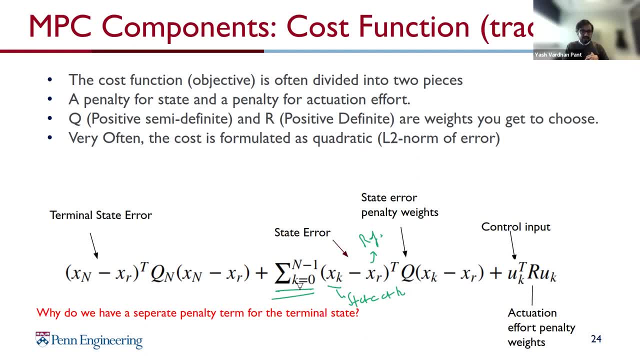 you won't see the answer in these slides, but the answer is: you want to get some strong guarantees on stability of your model predictive controller, so that's why you have a terminal cost as well. in general, if you look at this cost function, it's a quadratic term and it's a cost function. it's a quadratic term and it's a cost function and it's a. 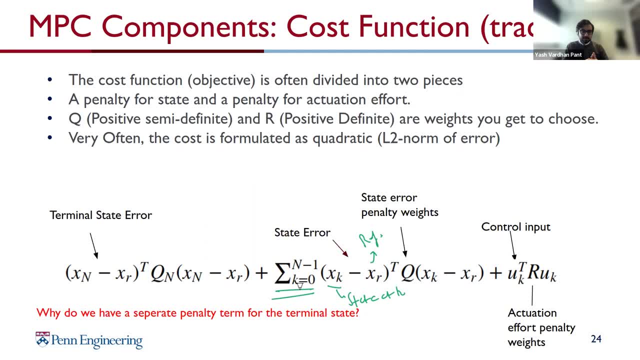 quadratic function and it's going to be convex because q, qn and r all have eigenvalues greater than zero. so something to keep in mind when you design your cost function. but usually we'll think about quadratic cost functions when we design model predictive control. all right, um, so that was. 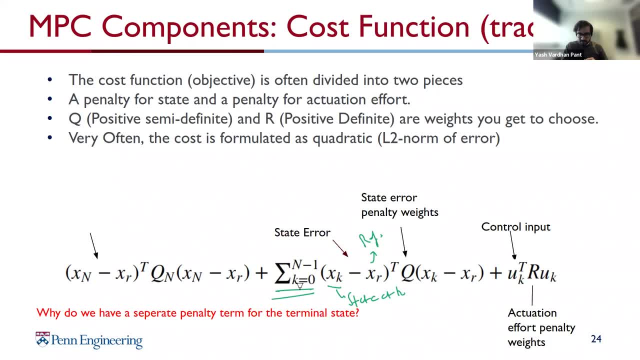 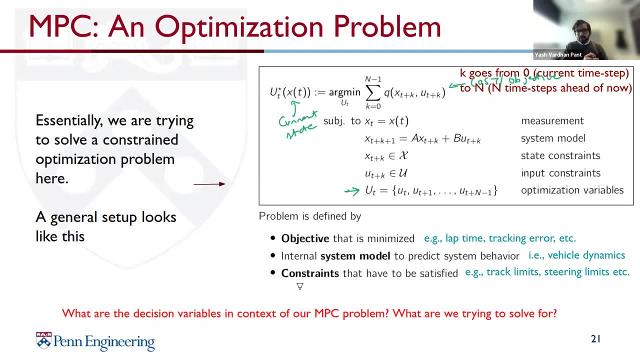 the cost or the objective part of npc. so maybe let's go back a couple of slides, right? so npc has a cost function, right? that's the that, what you're minimizing. and then you have a bunch of constraints in model predictive control that your variables should satisfy. so now let's talk about those. 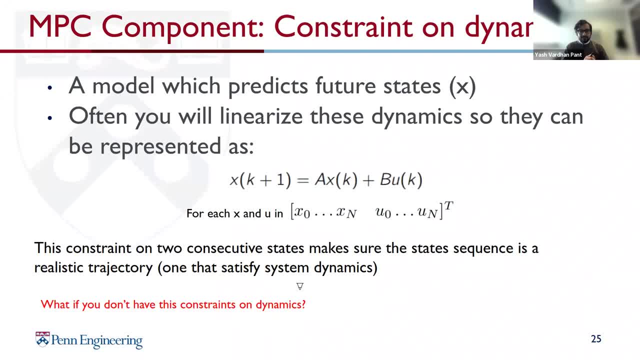 constraints. the first constraint is that you have to use the right model for your system because you want to predict what's going to happen all the way to the end time steps ahead. so we'll work with the model. often times we'll work with linear time, invariant or lti systems. if you've taken esc500. 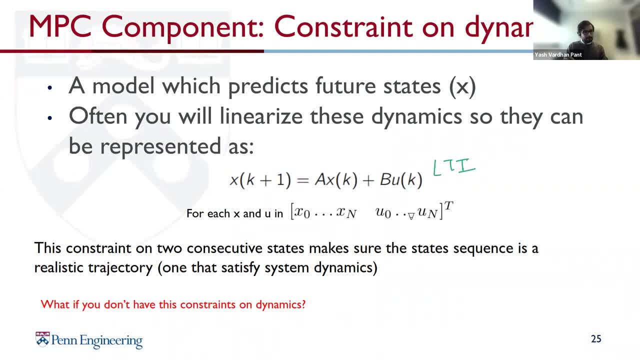 on a linear systems class. you should know what this is. if not, we'll briefly talk about them at the end of the lecture. so, yeah, you have these dynamics that will tell you what your next state, or, given your current state at time k and your input at time k, um, what your next state at time step k plus one, should be. 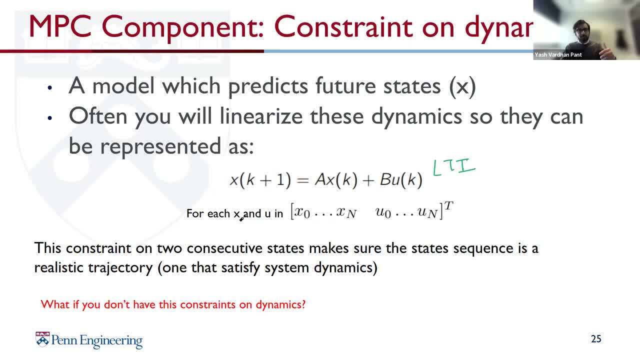 and you're going to apply this for each of your time steps. so this is a model that we'll use on the inside of npc to predict our behaviors. um right, and of course, we'll have these constraints on two consecutive states to relate the state evolution in a continuous manner. that is, um. 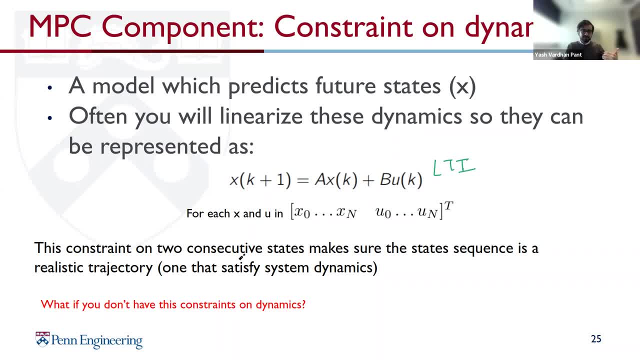 you know that your current state is going to be impacted by your previous state and the previous input. usually we have these kind of markovian behaviors, but you could also have regression models where your state is a function of not just the previous time step, but maybe 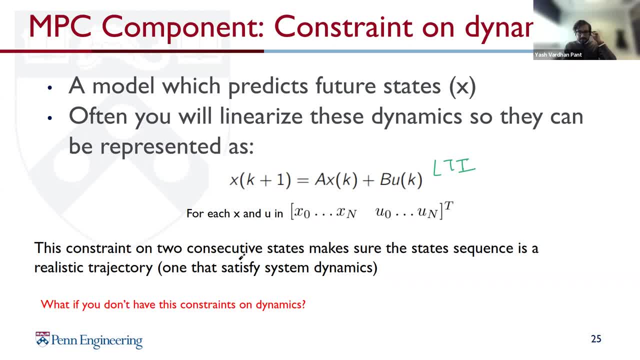 some memory before that as well. this question over here is: what if you don't have these constraints on the dynamics? what kind of? what kind of trajectories could you generate then? does anybody want to take a guess at you know why we, why these constraints are very important? 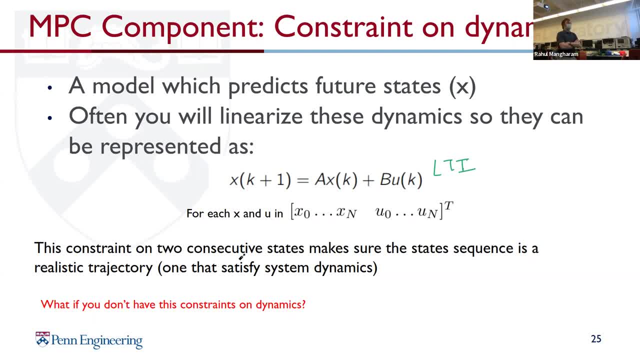 my first guess is that it's because non-linear dynamics are much slower to tech, uh to calculate. so, like it was brought up before the delay issue, you run into issues with that and also just non-linear equations are not friendly, um, so right now we're only restricting ourselves. let's say the: 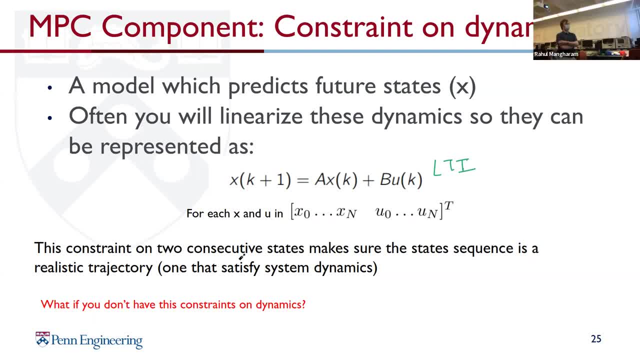 system is actually linear. let's say there are no linear dynamics. so the question is: why? why should we have this constraint when we try to predict what's going to happen: the next step in the next time, step times after that and so on? oh, in that case, it's just because the because it'll ask for. 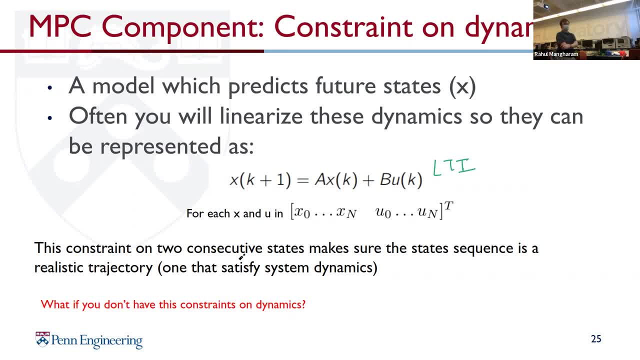 it'll ask for inputs that with uh dynamics and it won't actually know what it's doing. yeah, that's kind of the answer. yes, uh, you want to generate dynamics that your car. you want to have predictions that your car can. by the way, thank you to the student to give the answer. 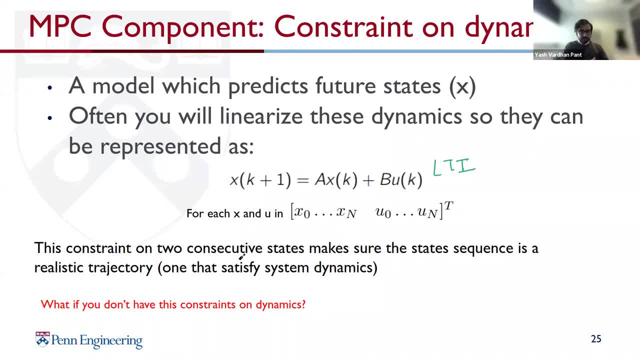 you want to predict your states in a way that the car can actually drive through them, which is why you have to connect the state from one time step to the next using your dynamics. so it's very important to have these dynamics constraints in your mpc, otherwise you're 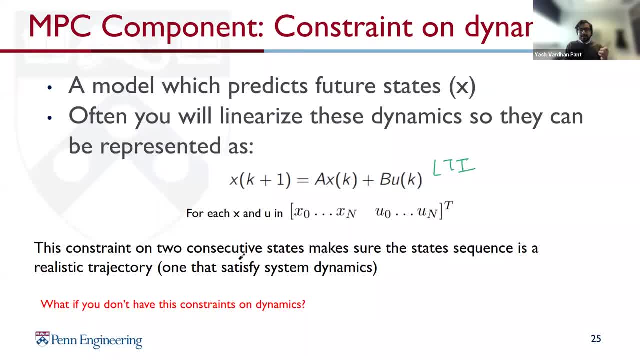 solving pretty much a meaningless problem. and right, uh, we use lti. i think the first part of what the answer was was that you're going to use linear time invariant systems because they're they lead to convex optimizations which can be solved easily, as opposed to if you use the actual 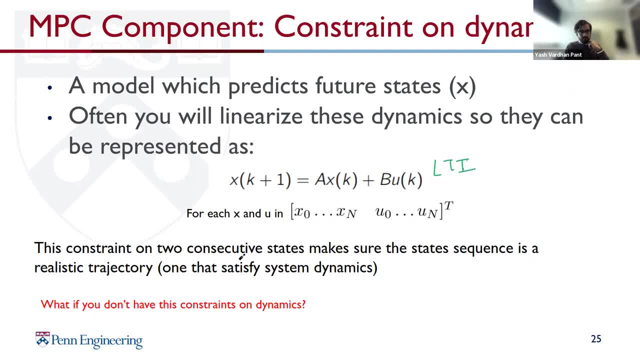 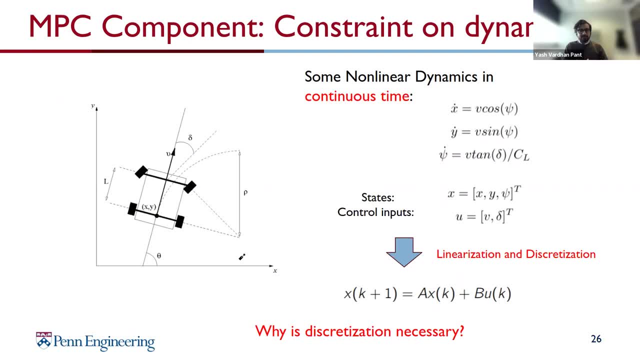 non-linear dynamics for your car. it'll make the mpc much more computationally intractable, so but yeah, we'll get to that. in fact, if you think about these dynamics, uh, you start off with some non-linear dynamics. for example, these are known, uh, holonomic dynamics for your vehicle with a. 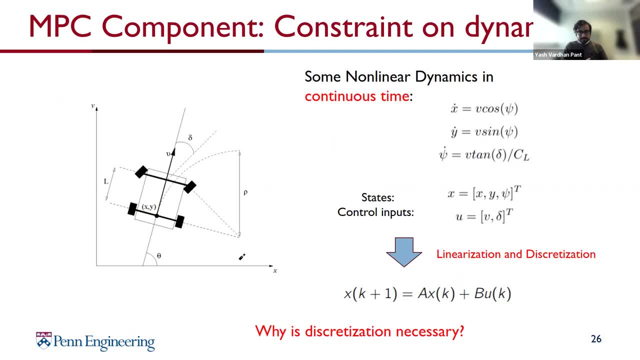 steering angle delta and a fixed velocity. v, that states your positions in x, y, orientation and also again, your inputs are your velocity and let's say steering angle delta. it's a non-linear system and we don't want to throw it directly to the mpc. this also is a continuous time system. you don't get the 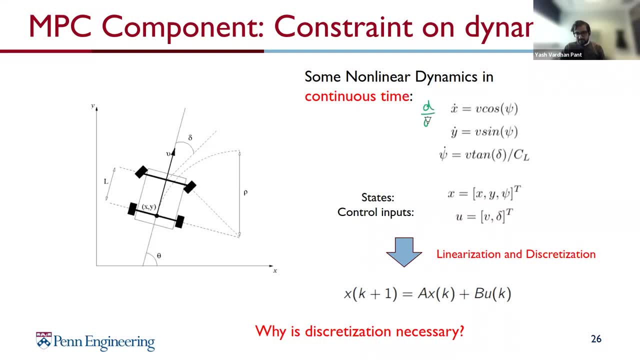 next state. but what you're looking at over here is the time derivative of these physical quantities. so if you say x, dot, we really mean um, bx by dt or the rate of change of a variable with time. similarly for the rest of them- and again, this is not something we can throw directly to an optimizer. 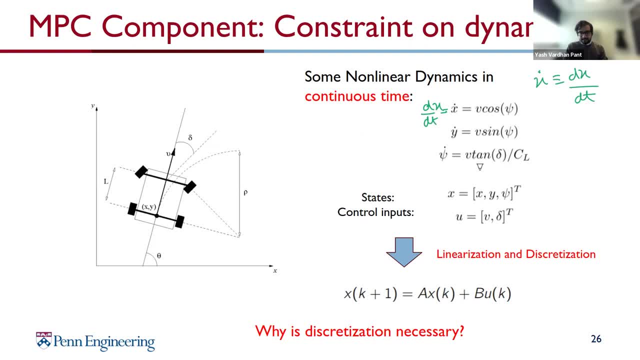 so what we're going to do is we're going to first linearize the system, come up with an ordinary differential equation, and then, further, we're going to discretize it, and i'll answer the question over here. it has to be discretized because, again, if you're writing an 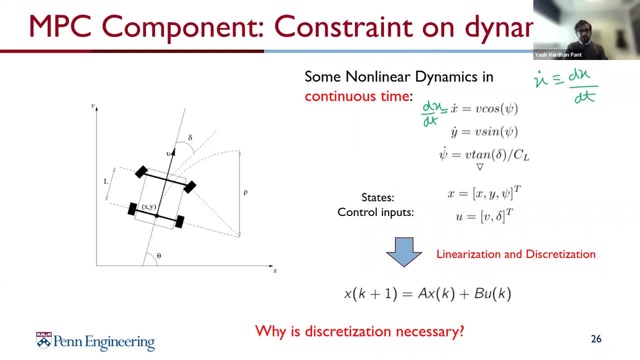 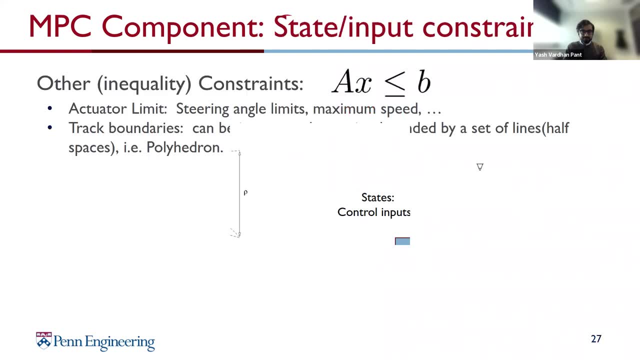 optimization, there have to be a finite number of constraints. so if we want to talk about n time steps ahead, we should have n states, and so we're going to discretize our dynamics in time. all right, so those were the first type of constraints which are for your dynamics. 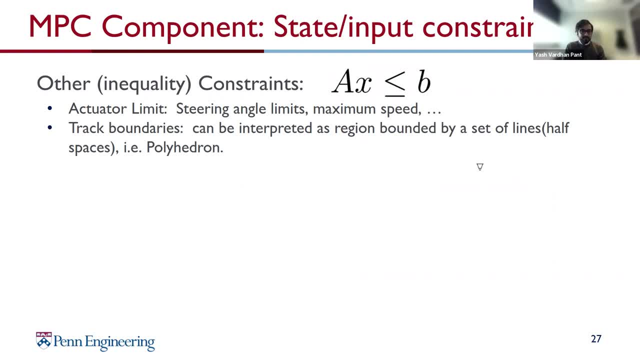 you can also have other constraints on your state and input. for example, you could have actuator limits that a steering angle has to be within, say minus pi by three, and pi by three, your car can't go any faster than 20 miles per hour. you want to take that into account because you don't want to. 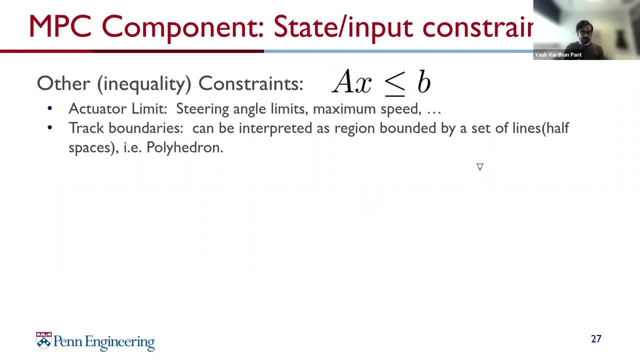 plan trajectories that go all the way to 50 miles per hour when you know your car can't actually go that fast. you also want to take into account things like your track boundaries or other cars on the track, and so the way we're going to represent these constraints. 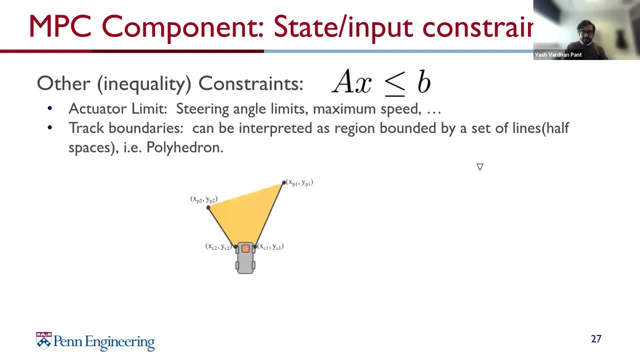 is, through the polyhedral form, ax less than equal to b. so i think what's shown over here are some kind of polyhedral constraints that you could have. for example, you have a car with a cone that it's going to try to stay within. 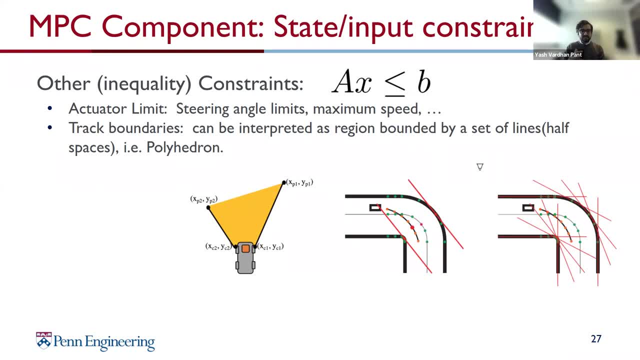 or try to stay within the boundaries of the track by looking at these two essentially stay within these lines. these lines are called half spaces because they break your space, divide them into half, if you are on the left side of it or the right side of this half space. 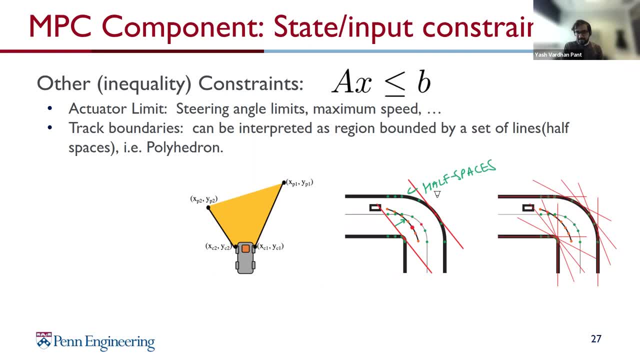 you get half of your entire 2d space and you want to stay within these kind of lines. the intersection of these half spaces is what defines a polyhedron. we can write this in matrix form as ax less than equal to b, where a is a matrix of an appropriate 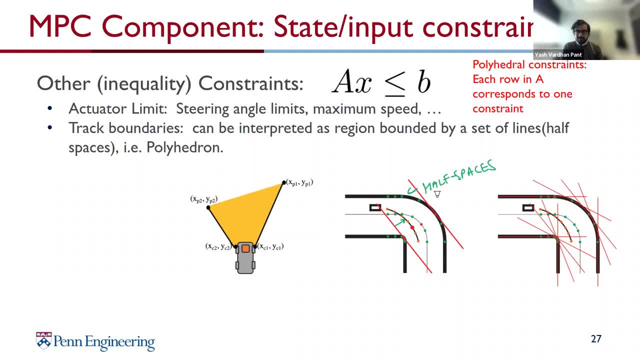 size b is a vector and x could be your vector for your state or your input, or you can concatenate it all together, put it into one vector. but in general, for our model predictive control algorithm, when we say constraints of the kind that our state is within a set x or our input is within a set u, 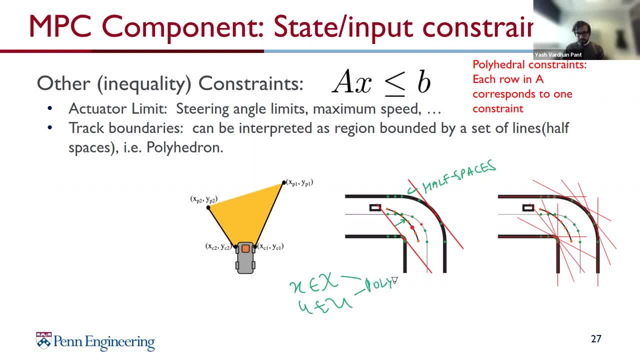 these x and u are going to be polyhedrons or polytopes if they're bounded. and again, this is in order to keep. at the end of the day, you want to have computationally tractable optimization to solve, which is why we're going to use these kind of constraints. 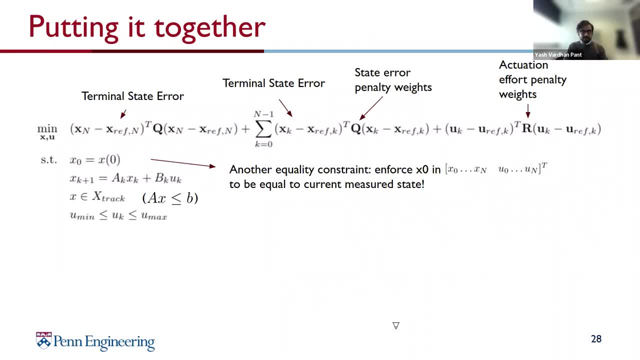 all right. yeah, let's put it all together. then we have the NPC in a following form: we have a quadratic cost function to be minimized. as we saw, there's a terminal state error. I think terminal state error has been written twice. this is not terminal state, but just state error. you have some. 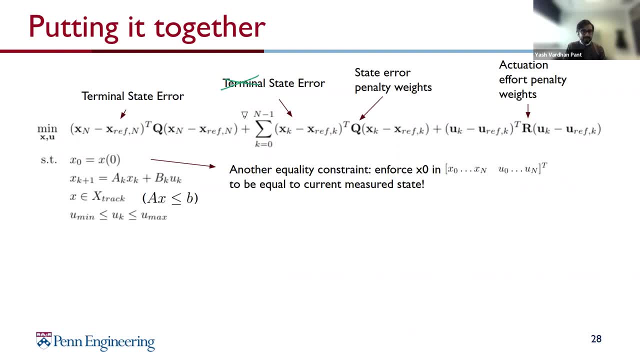 penalty on how much actuation effort you're going to implement. and then you have constraints. the first constraint is start at the right state, so take in your feedback or start with where you are, bar at time 0, then you use your dynamics to update what your next steps are going to be. 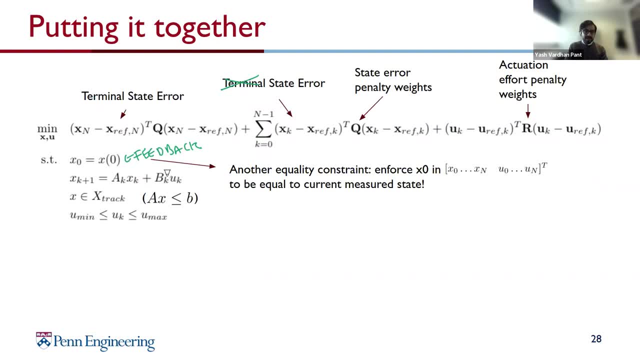 You can then have some polyhedral constraints, for example, staying within the track and for keeping your control within some given bounds. So this is one example of a MPC with a convex optimization. linear constraints- Questions. On the previous slide you were showing the state constraints. 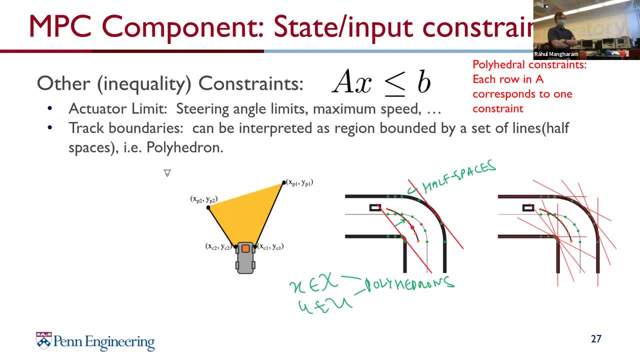 And so my question is: isn't it fairly easy for that constraint to become non-convex, given we don't know the shape of the racetrack? Yes, that's a great question. Do you have any suggestions to avoid that? 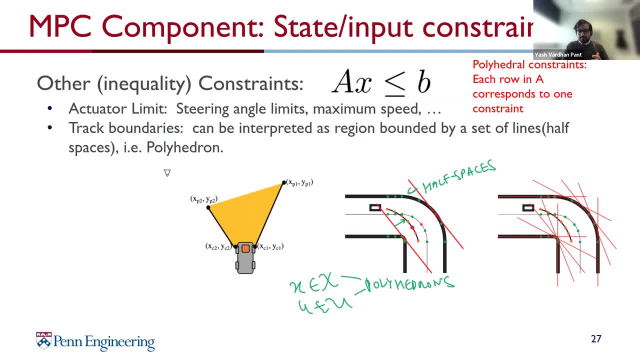 Yes, and we'll see this when we actually we won't see this in this class, But there'll be a reference to the model predictive control and control paper, And in there they come up with these ways in order to convexify your track. 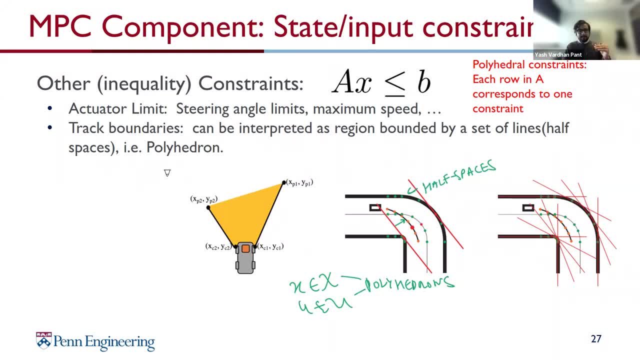 Think of it this way: You're: As you move along the track, you want to keep a look ahead that only cares about some vicinity in front of you, And for that you can find the right half spaces to stay within, like in this third figure over here. 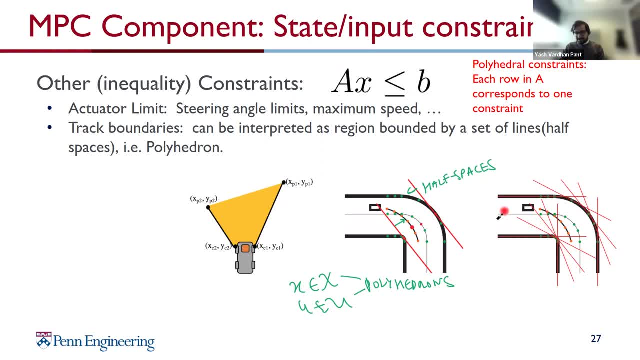 Let me put the pointer: If you're at, let's say, this position in the track, let's say all the way to the left, you maybe just want to stay within these two lines, which will define a convex constraint Next up as you get closer to the curve. 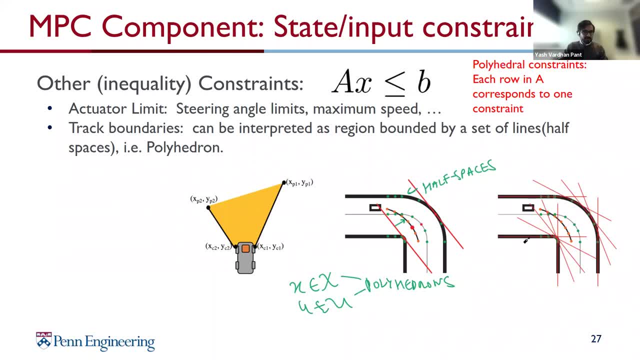 you could take the track and find a linear, under-referenced, linear approximation of it by finding, let's say, the tangent lines to your track boundaries, And that's going to define a half space to stay within. Similarly, as you move along, just keep on finding the tangent. 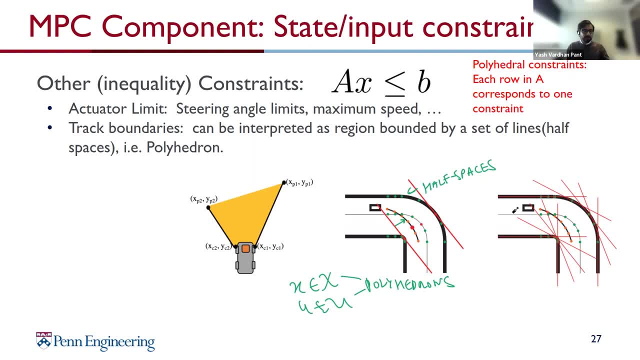 stay within it. So now update your constraints at each point in time. So that's one heuristic that you could use to get convex constraints. OK, thank you. Thank you, That was a good question. Yeah, and these kind of things will be covered in more detail. 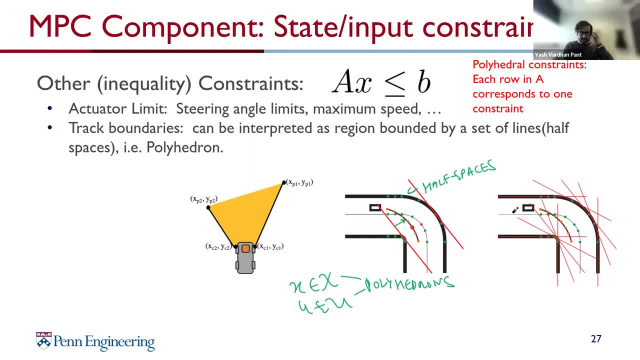 in the reference for MPCC. I think that's what you folks will be using as an implementation as well. So But yeah, for now, I assume someone at a higher level gives you, someone tells you, what your convex constraints are to work with. 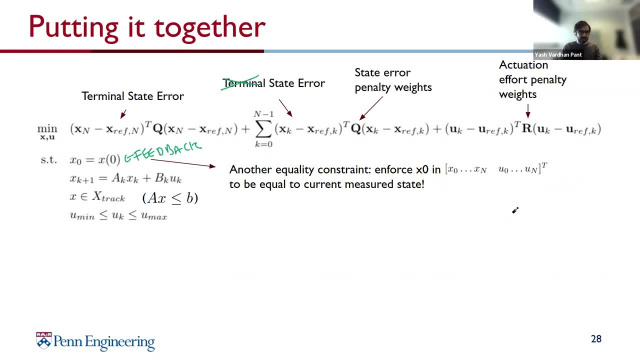 So those are going to be our track constraints And, yeah, they could be changing over time. as we just talked about, They're not necessarily time invariant. All right, so we can put all this together in an optimization, And the question then is: how do we solve this optimization? 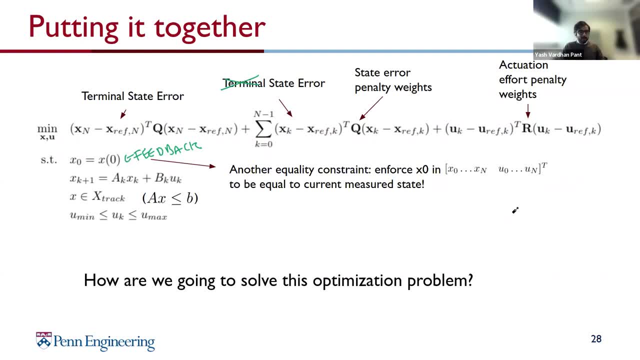 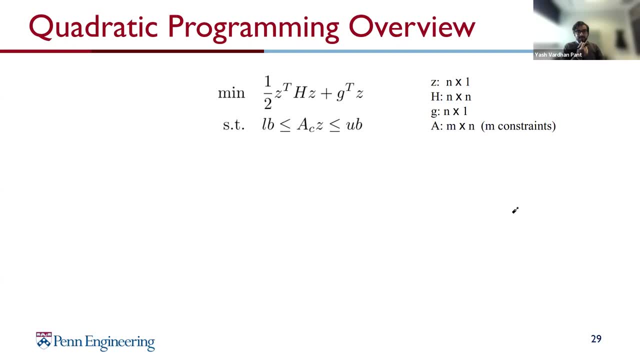 problem, Long story short, is that we're going to throw it to existing optimization solvers. Let's take a look at what some of them can do for you. So, on the inside, we'll be using quadratic solvers, And so just to give you a quick overview, 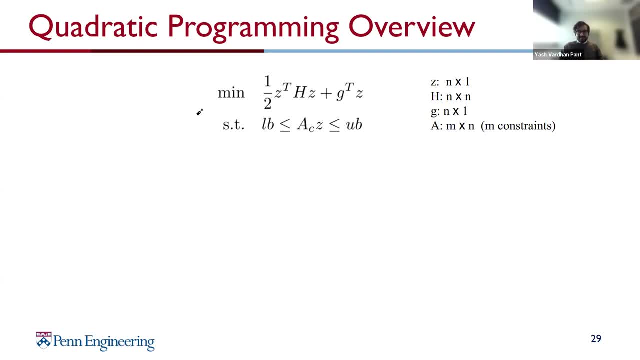 of quadratic programming. you're looking at a quadratic cost where Z is your optimization variable. So you're doing this minimization over z. Z is in some dimension. rn. H is a square matrix that has to be greater than 0, that has positive definite. 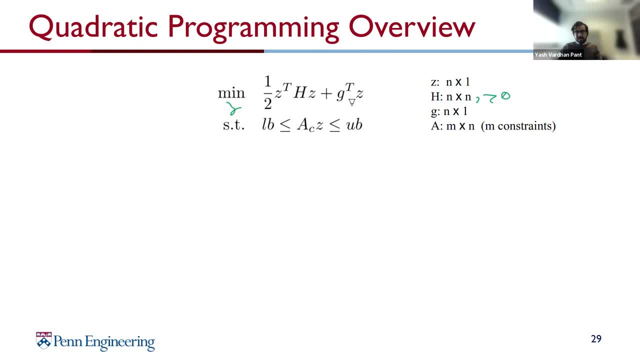 G is a vector that gives you some affine term or a linear term to have as well. OK, have upper and lower bounds on z based on some constraint matrix- ac, so it should be ac. so this is what a general quadratic program looks like. model predictive control also fits into this. 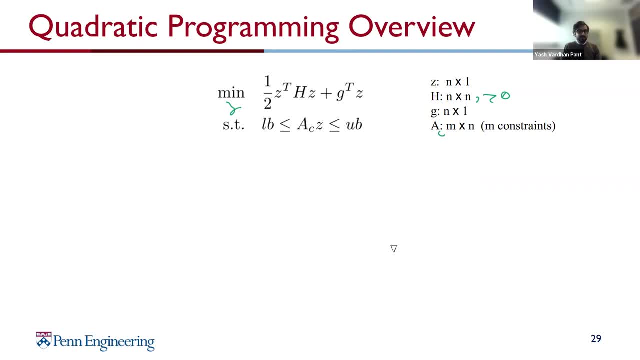 category. we saw it. it has a quadratic cost. it's called linear constraints. now all we need to do is massage it into a form that we can write it. in this form, essentially define h, g, ac, lb and ub for mpc and then throw it to a standard solver that can solve these kind of optimizations. 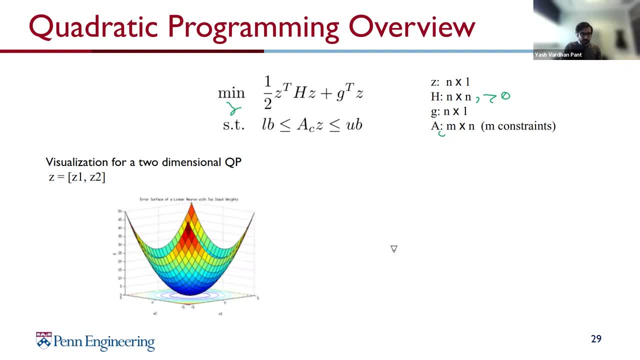 let's take one example of what a two-dimensional quadratic program would look like over variable z1 and z2 and some positive definite matrix edge. so quadratic functions usually have this bowl-like shape if you think of them in higher dimension, and this is something that again is. 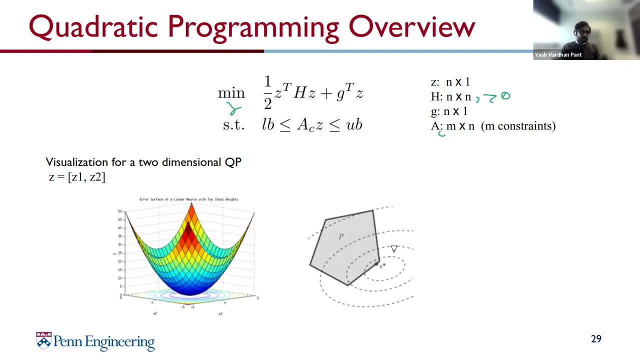 obtained because you have a positive, definite matrix edge. now the property of quadratic, solving quadratic programs, is that gradient descent-based methods shown over here is the constraint set defined by the polyhedron, by a, by this matrix a and the upper and lower bound. but essentially you have these linear polyhedral. 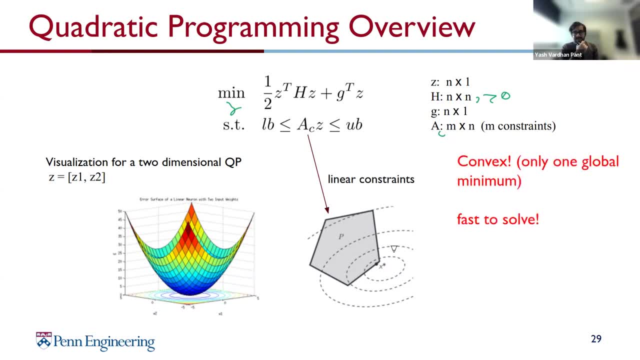 constraints and because the problem is convex you: any minima is guaranteed to be a global minima, and so these methods can be solved quickly through gradient descent and you have nice convergence guarantees. so again, mpc with linear systems, linear constraints, is a quadratic program and you can just solve it using off-the-shelf solvers, right. so the next step then is: how do we massage? 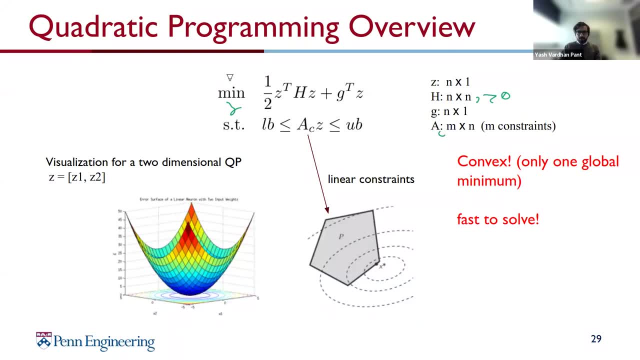 mpc into a form shown in these two equations on top. essentially, we want to write it down as a quadratic program and we'll see what we need to do then in order to do that. oh yeah, i guess the question is what happens when the constraints are non-convex? 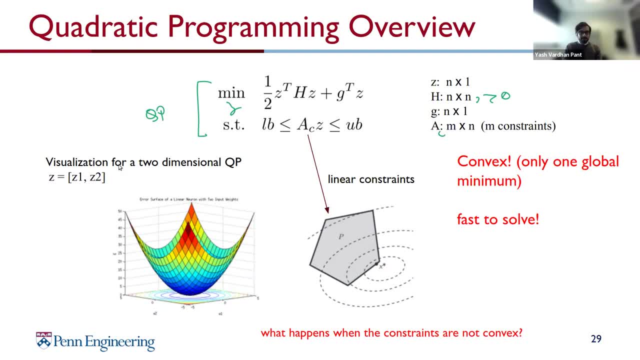 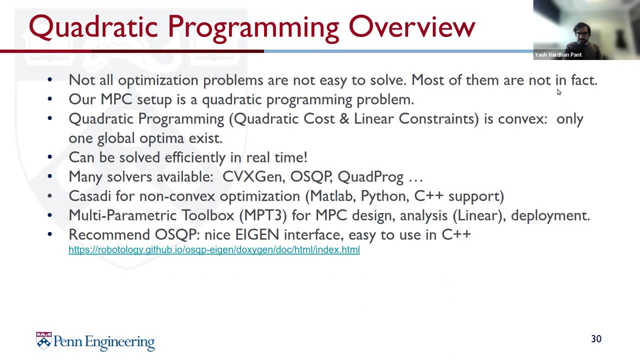 and the answer is nothing good, so we won't talk too much about that over here in this class. oh sorry, um, to get rid of this message right. so yeah, uh, we can take our mpc. we'll see in the next few slides how we turn it into a quadratic program, but not all optimizations. 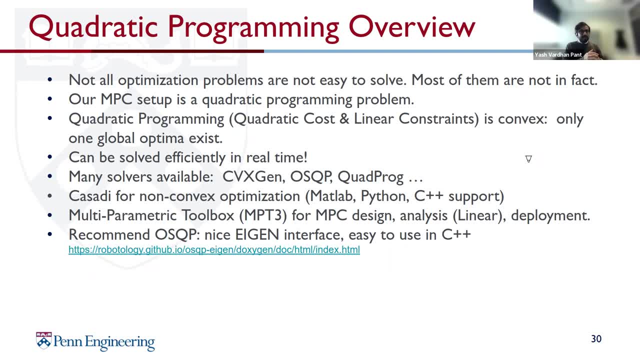 are easy to solve. um in general, we get away with a lot of things if we have an mpc that can have linear dynamics, linear constraints. there are a bunch of solvers that can solve essentially these kind of problems almost in real time. you could use tools like cvxgen. 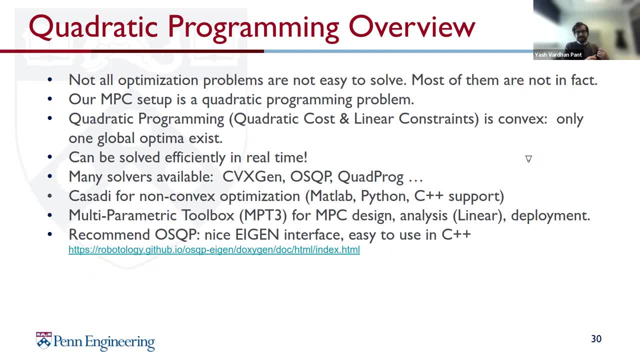 which is an online tool that will generate c code for you, which you can directly send to a microcontroller or implement it however you want. try to wrap it in a ross node if you want to. um works for systems with a few states and a small horizon- simple constraints. you could also 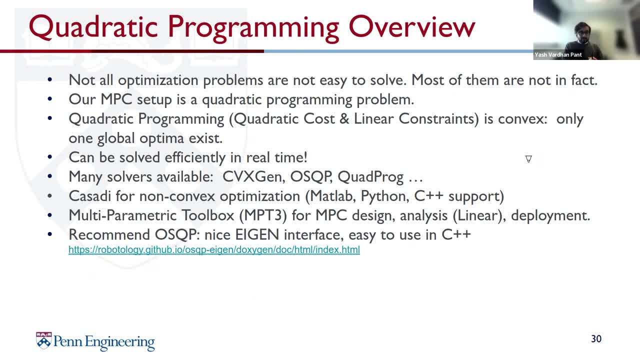 use osqp or solvers like quadprog. if you do want to deal with non-convex optimizations, because, let's say, you're feeling adventurous, then cassidy is a great tool. uh, it's open source. you can, and it has support for matlab, python and c plus, plus interfaces to state-of-the-art non-convex. 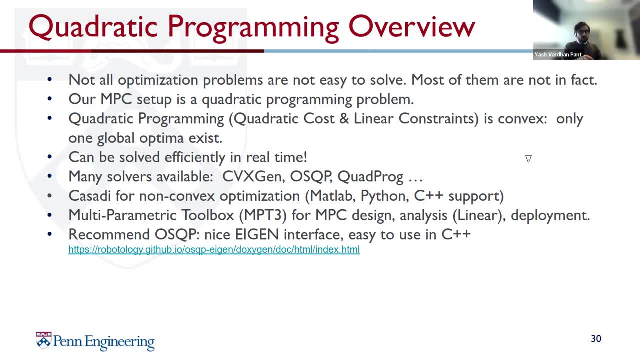 optimization solvers as well. so, yeah, it's a again. if you want to um do non-convex mpc. cassidy is a great tool for that. um, there are also other tools like mpt3 from eth zurich. it's a matlab tool that's great for mpc design analysis, especially for linear systems, even for linear time. 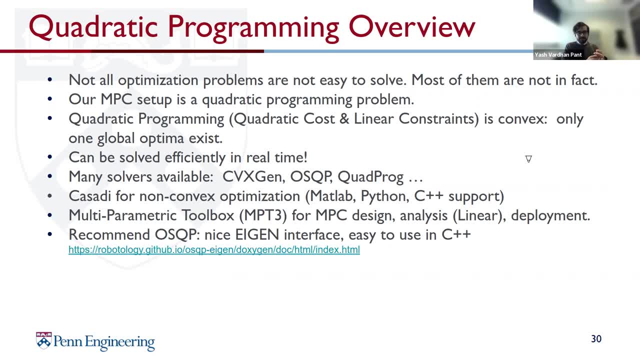 varying systems and it also does deployment for you. if you want to generate c code, it can do that for some classes of simple linear systems as well, and i guess in this class, uh, osqp is the recommended solver. i guess the lab instructors can tell you more about that, but anyway, um, talking about 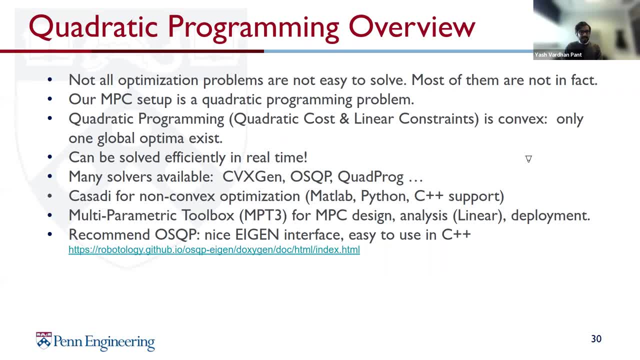 mpc and how to convert mpc into a quadratic programming. because mpc can be turned into a quadratic program and then it can be solved through off-the-shelf solvers. and so now let's see how do we get mpc into a nice quadratic programming. standard form. 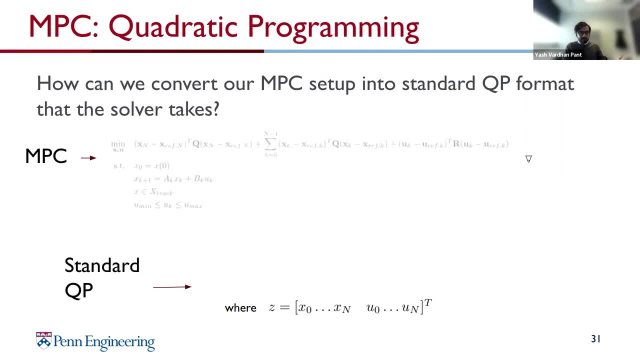 all right, so now let's fill in the blacks over here. the question is: how do we convert mpc into a qp? started off with the mpc in the following form: we have a quadratic objective over variables that are both the state and the input, so x and u. 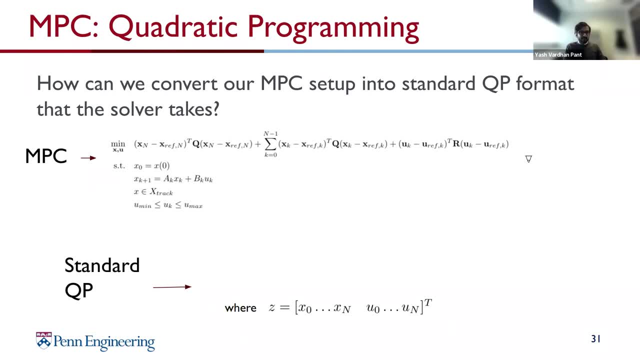 and then we have some inequality constraints for our dynamics and the initial state, and we have some inequality constraints that might define, for example, constraints on the state track boundaries, constraints on the input and so on. standard quadratic program, on the other hand, is given in the following form: where you're working with a single optimization variable, z, it's in some 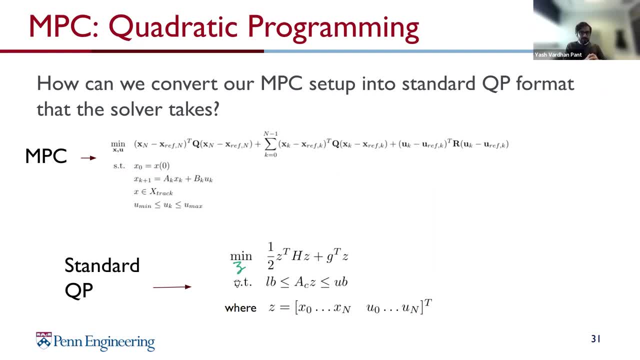 higher dimension, rn, let's say. so you have a quadratic form of that and you want to write constraints in the form that essentially these two polyhedral forms that acz is less than equal to ub and acz is greater than equal to lb. so there's a lower bound and upper bound on what? 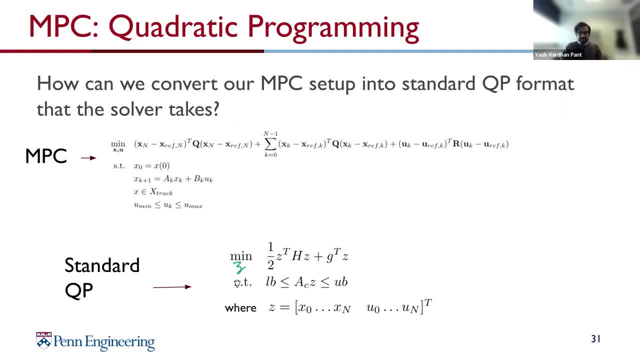 these variables can take, or what linear combinations of these variables can take. so again, this is a quadratic form and this is a linear polyhedral constraint. and again, these kind of problems are called convex quadratic programs. mpc fits the bill, but we need to do some massaging in order to find an h in terms of the q and the r matrices, for example, find ac. 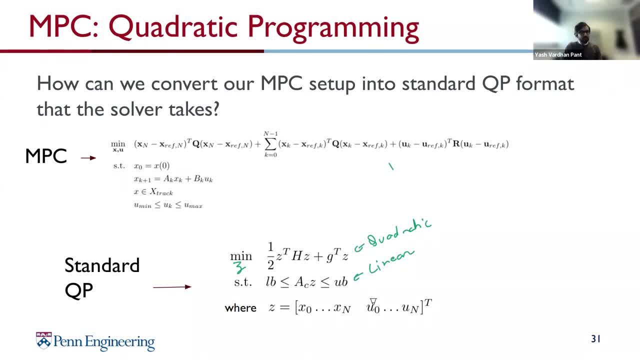 lb and ub in terms of the a and b matrices or the u min, u max that we have over here. so the next few slides we just talk about what kind of bookkeeping it takes in order to get that form again. this is not something you're expected to see out of the box and recognize, but, as you, 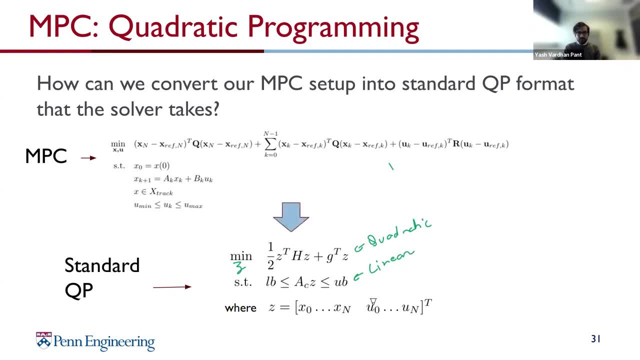 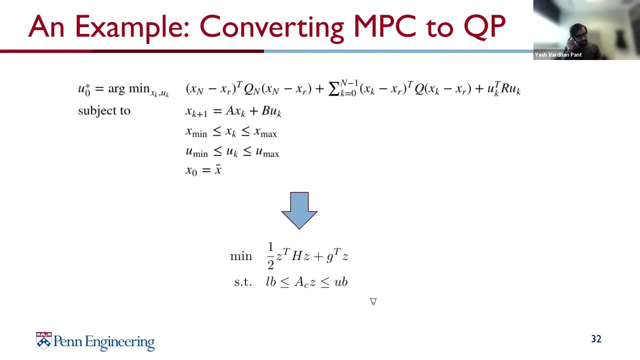 start writing down your own mpc. you'll see yourself going through these kind of steps, right. the question is, how do we do it? and we'll take a simplified form of the mpc where our state x and some set x are just upper and lower, bounded by x min and x max. 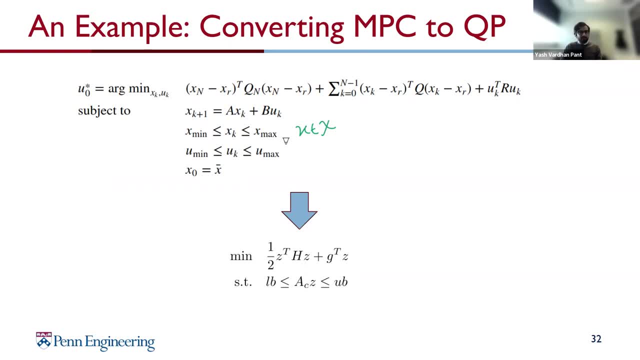 if they're of a different polyhedral form, a similar approach will work. you'll just see different kinds of h. you'll see different ac matrices compared to what you're going to see in the next few slides. right, so we're going to take our mpc optimization, write it into this. 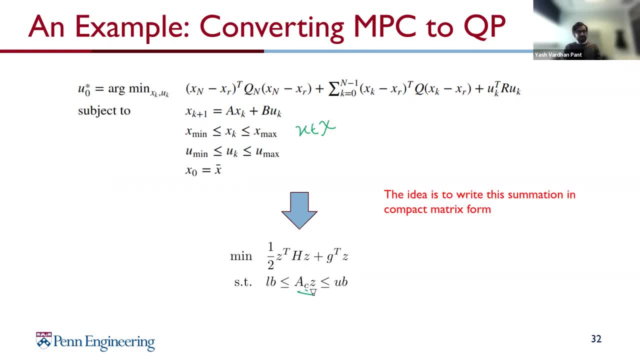 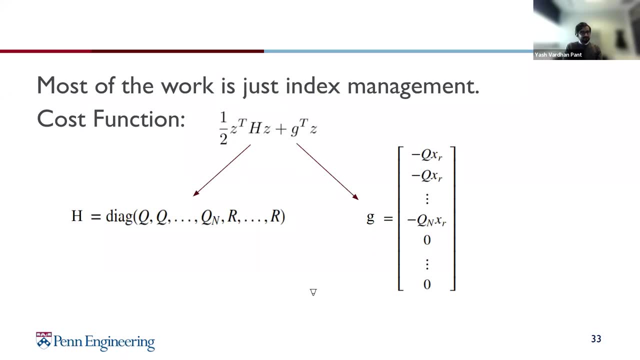 compact matrix form, essentially stack up all our constraints, stack up the objective in the right form and then come back to it in the next few slides. so the next thing we're going to do is we're going to come up with a simple, compact form. as i've alluded to, a lot of this is just bookkeeping, so the edge matrix can be given. 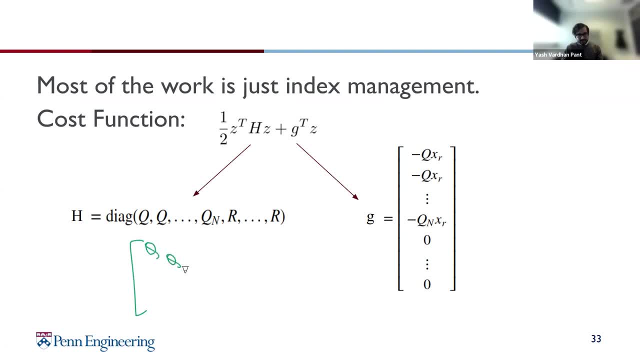 through a diagonal matrix that has q, q and going all the way to qn in your diagonal elements. it also then has the appropriate number of r's. essentially there's going to be n of these q matrices because you had n time steps in your mpc. so if you go back to the sum, 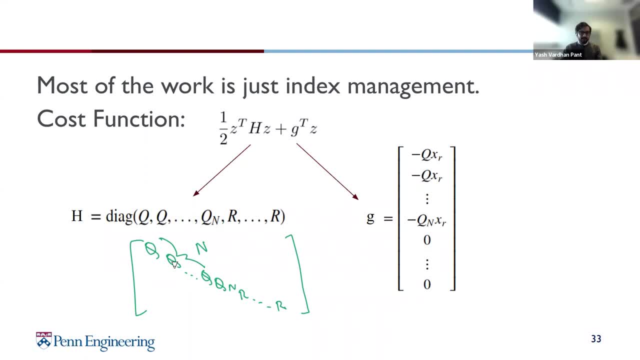 you take a look at it again, it's going a sum that goes from zero to n minus one. this is your terminal cost. so that's your terminal penalty, qn, and you will have nr matrices that correspond to penalizing n of your control inputs. so in matlab you can simply come up with this. 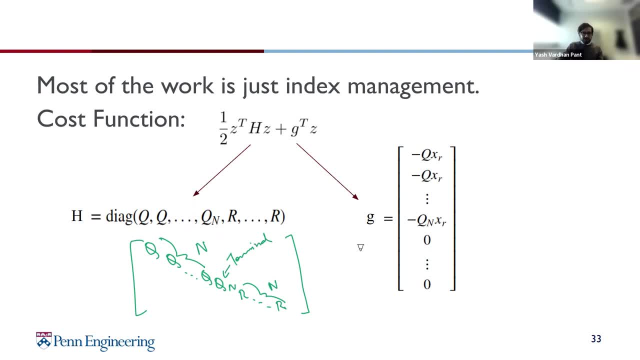 giant edge matrix by using the diagonal command or the diag command. g over here is going to be a linear term that's going to take into account your reference part. so remember we had a cost of function that was of the kind that it's xk minus x reference. transpose q. oops, xk minus x reference. 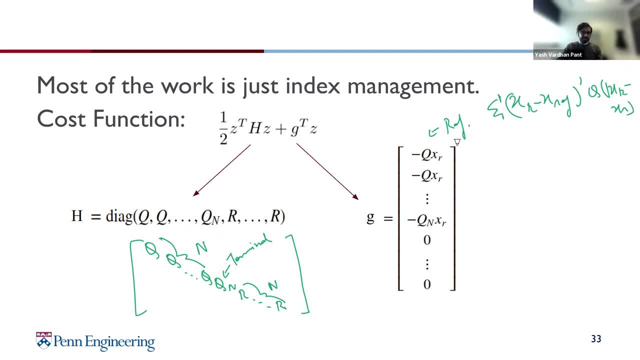 and you're summing this up. so you have those reference terms and we can just take those away and get a linear form for them, as shown over here in g. so again, if you don't understand what's happening exactly, you don't have to worry about it too much, but you will worry about it once. 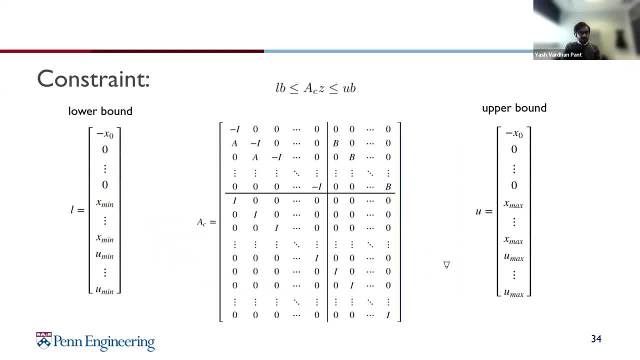 you start to implement some of this on your own. the second part, then, are the constraints. how do we take our dynamic constraints and the state, state and input constraints and map them to this compact form shown over here? and in order to do that, we'll essentially just take our constraints one by one. 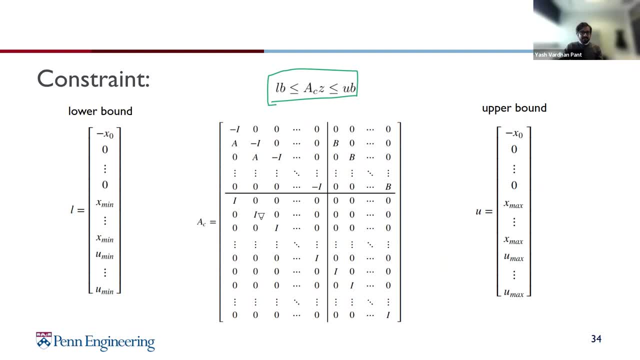 and write them down in a vector form. so, as an example, let's take a look at the first of these constraints. so remember, our vector z is our states: x0, x1 all the way to xn plus n, followed up by u0 all the way to un. so if i stack it up, that's going. 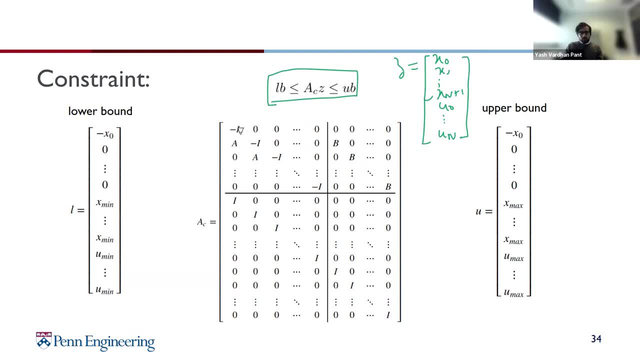 to be my vector z and what the first row over here is saying. let's just focus on the first row. if i multiply the first row with the vector z, i'm just going to get x naught out of it, or minus x naught. and what this is saying is that first row says identity times x0 is. 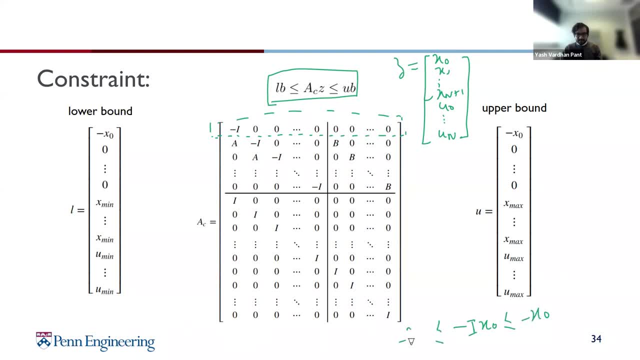 less than equal to minus x naught. greater than equal to minus x naught, or essentially, this is forcing the fact that x of 0 should be um. you should again initialize with the right measurement or with the right initial state. so that's what the first row here is going to tell you. 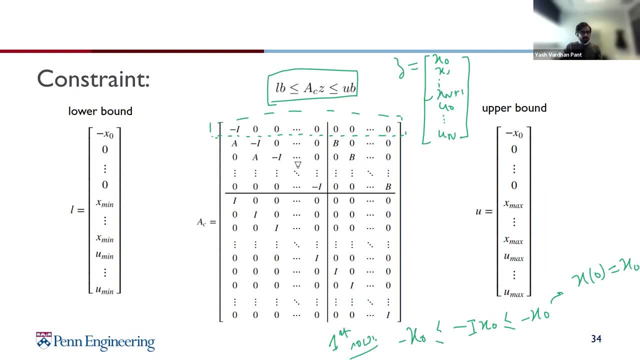 similarly, if you take a look at the second row, it's going to give you a state update equation. it's going to tell you that x1 is ax naught plus b? u0. that's the second row. the third row is going to give you: x2 is ax1 plus bu1, and so on. 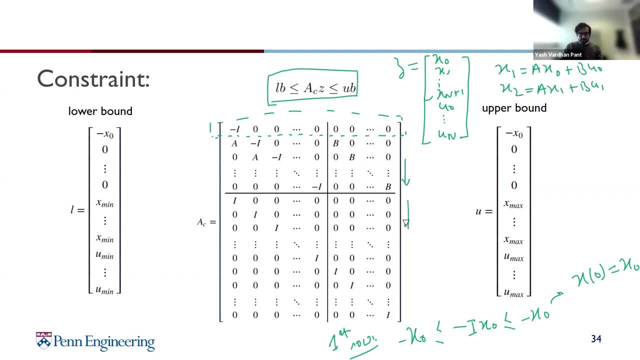 so that's all the way till here, and then, below this, you have your constraints, for essentially, as you see, x is less than equal to x max and x is less than equal to- sorry, greater than equal to, and x is greater than equal to x min. so if you 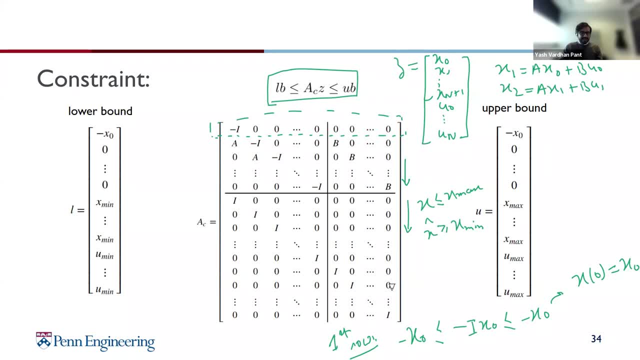 go through these rows. that's all you'll get out of the first um n rows over here. the others are just saying that u is less than equal to u max and greater than equal to u min. so again, just a lot of bookkeeping. but you can take your mpc with your linear constraints. 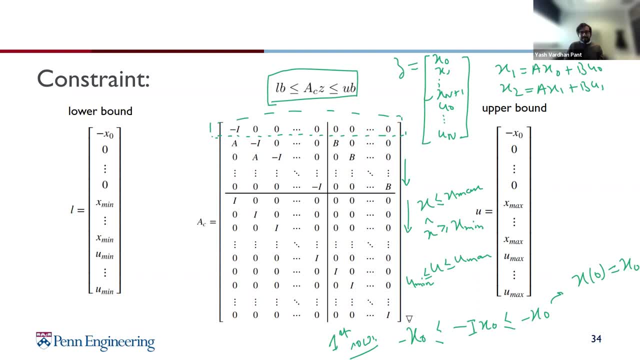 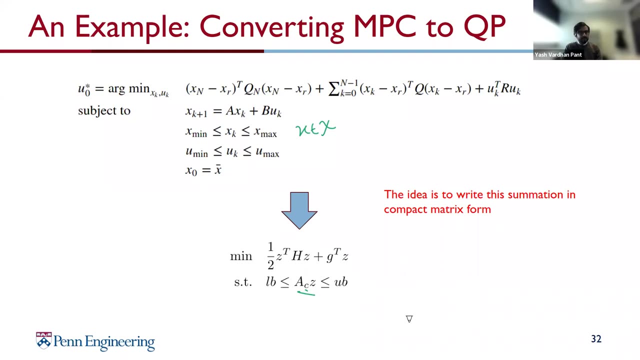 polyhedral constraints, which are equalities and inequalities, and then turn them into the polyhedral form as shown over here. so with that, what we have done is essentially gone from the mpc form into our standard quadratic programming form. any questions so far, before we move on to some of the implementation details on how you do this for f and 10.. 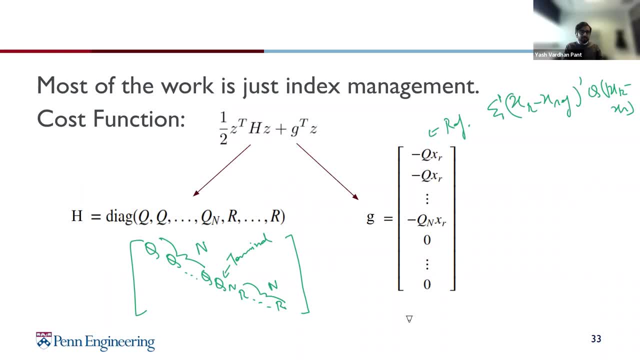 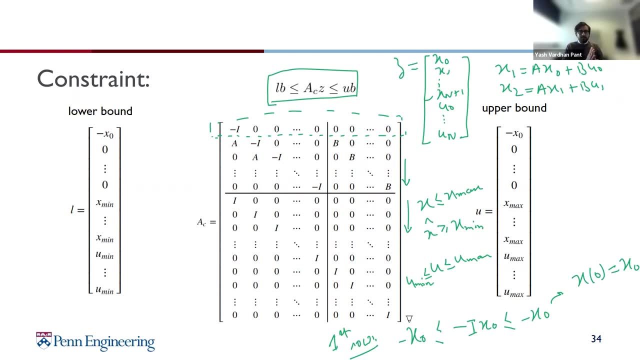 all right, cool, so no questions. usually happens when you get into the math and again, i wouldn't expect you to see this right away and be able to grasp all of it, but if you go back and work it out one row at a time, you'll see that you're. 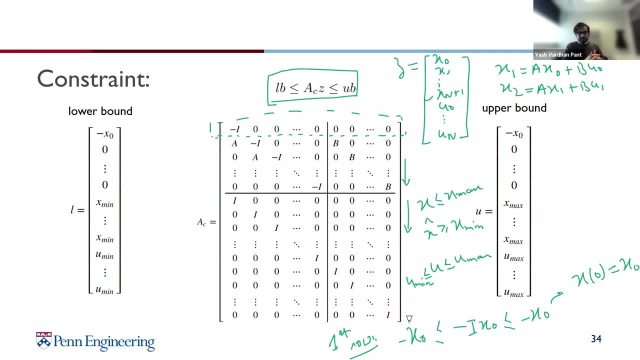 going to recover the same constraints that we had in the mpc and if you see that some of these upper and lower bounds have a bunch of zeros, that essentially is forcing an equality constraint. so i wrote it in the form that x1 is equal to ax naught plus bu naught. 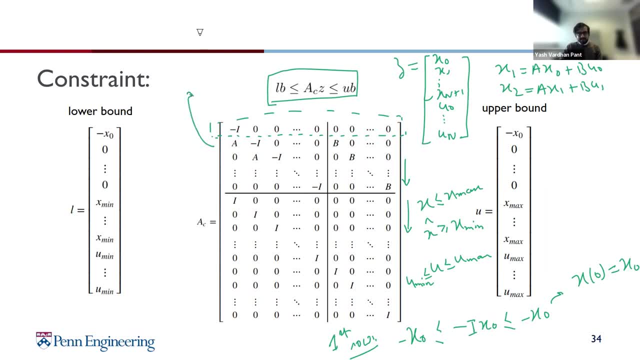 but what this is really saying- like, for example, this constraint is really saying- is that x minus x1 plus ax, naught plus bu naught is less than equal to zero and it's greater than equal to zero. so again, this is just force the equality that x1 is equal to x, naught plus bu naught, which 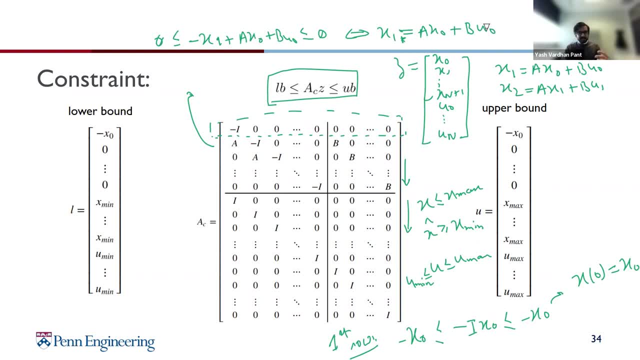 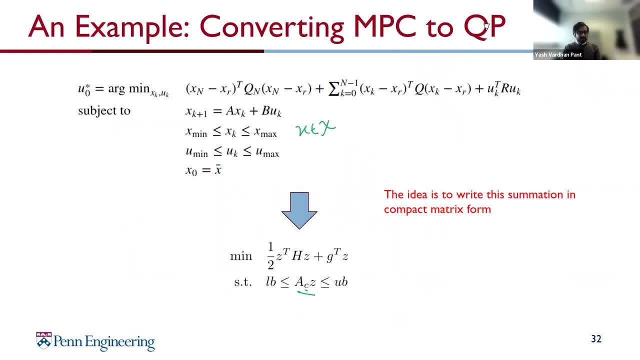 is a linear, dynamical system. so right, so go offline and work this uh through after the class just to get a better idea of what these constraints are. but through this exercise we'll have turned our mpc into a standard quadratic program and through that you can throw it to any solver of. 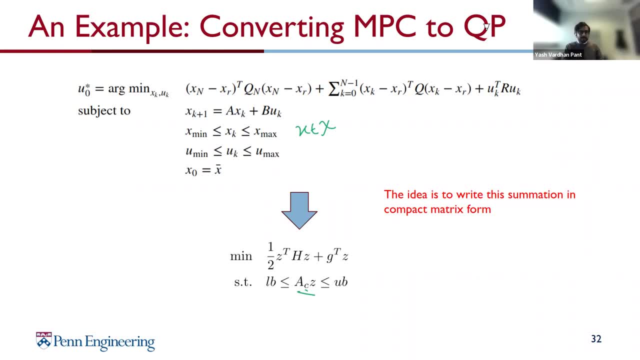 choice and come up with your sequence of control signals that are going to be optimal for this system, and then we'll apply it in the receding horizon manner that we saw before, that is, apply the first control input, wait for the next time step, get your feedback, recompute the optimization. 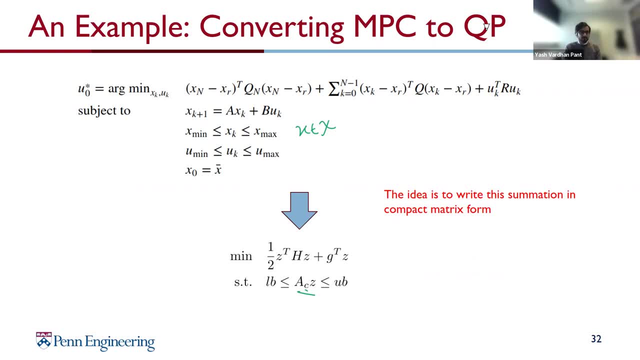 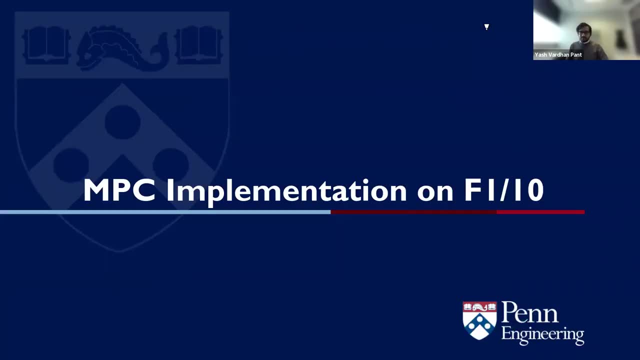 apply the first control input again, redo the process, and so you'll have your optimization working in a closed loop manner for you. all right, cool. so so far, what we've covered are some of the basics of mpc. um, so the underlying math. and now let's see. 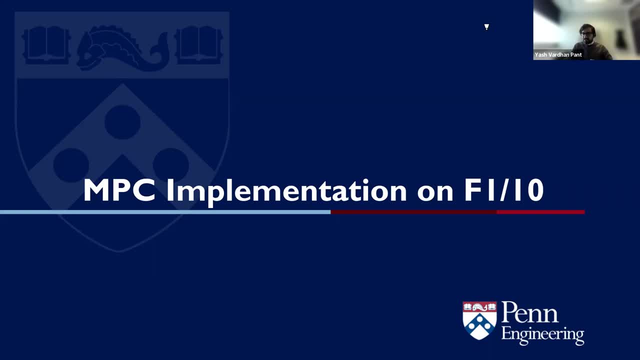 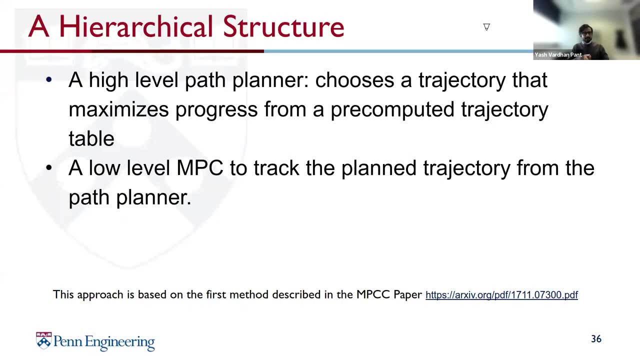 some mpc implementations or variants of mpc that are specific to the f and 10 or, in more generally, i guess, to autonomous driving on autonomous racing. so in the first video that you saw in the applications, we were talking about this hierarchical model, predictive control structure and well. 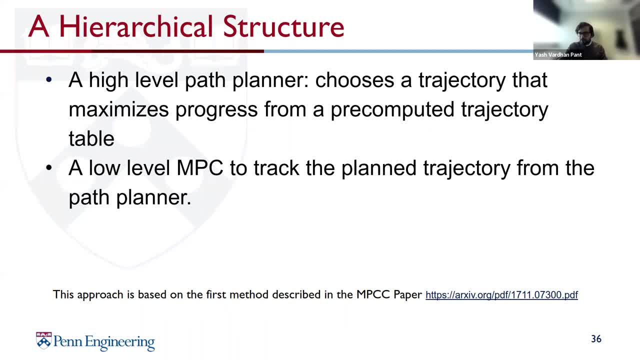 i think this paper uh shown in the with the link in the bottom. this is going to be a reference that you should visit if you have more questions about what's going on on the inside, for example, questions on how to pick the right track, constraints, how to make them linear, given your track could be. 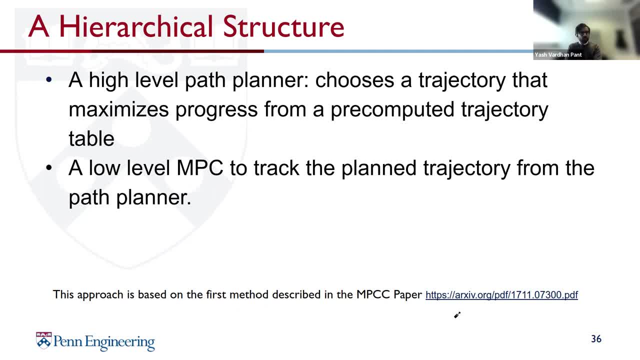 an arbitrary curve. um, so let's, this paper has two methods, um, that we're going to talk about over here. the first is a hierarchical structure for planning and control. first, at a higher level, you have a path planner that's going to pick a trajectory that, let's say, maximizes progress given. 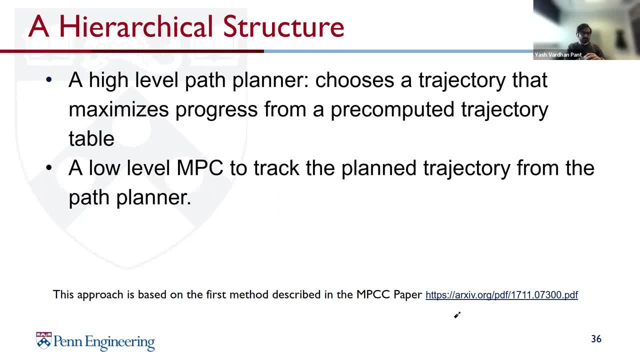 some pre-computed racing line or a center line, so you could use a high level path planner like, let's say, rrt star if you want to discretize your space. a star, although i would recommend that- or any other lattice based planner or whatever, and you have a high level planner that's going to pick. 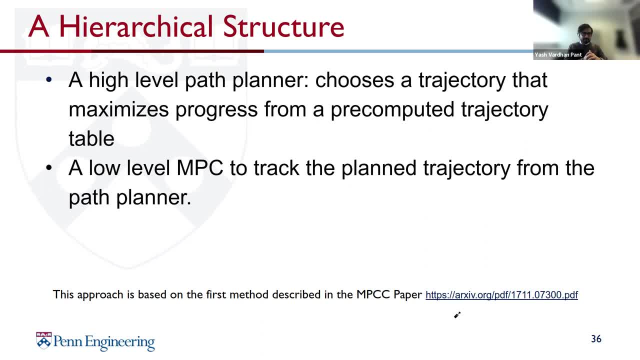 a trajectory that maximizes some notion of progress. that's the first level. the second level is a low level model, predictive control that's going to now try to track the trajectory best it can while remaining within the track, maybe avoiding static obstacles, and then the other way around. so let's say, if you have a high level path planner in your 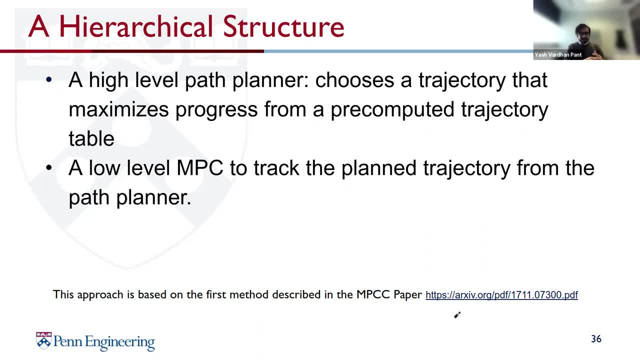 and so on, and that's going to be formulated in a. again see, that can be formulated as a model predictive controller. so that's the first hierarchical way of kind of doing autonomous driving around a racetrack. the idea is that first, in order to generate your high level trajectories, 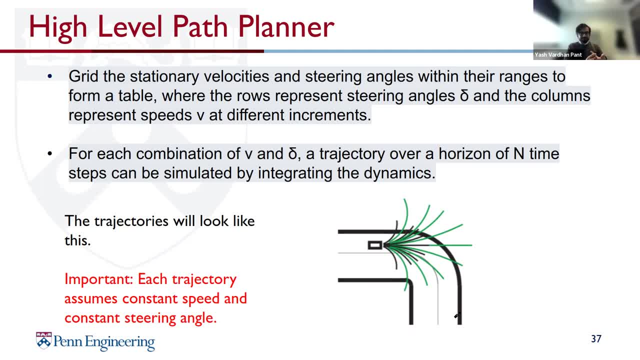 you can take your velocity, steering angles- maybe not track positions, but velocities and steering angles- and discretize them in a grid where, let's say, the rows represent steering angles and your columns represent your different speeds that you could have, and for each of these combinations a trajectory of some time horizon n can be simulated just by integrating the dynamics. 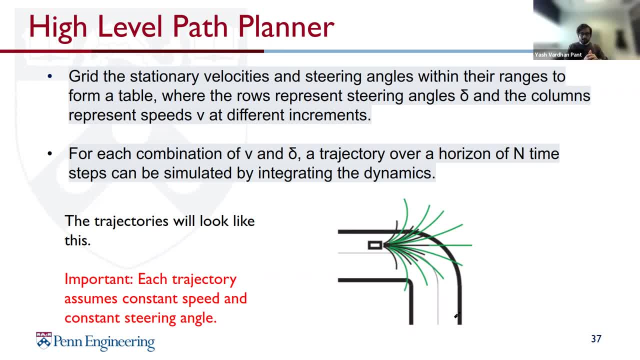 so this is the high level path planner, or the first level of your hierarchical approach. so you're just essentially taking some reference velocity and some reference steering angle, connecting them, integrating them over your dynamics. your dynamics, again, are just your linear dynamics or could be a non-linear dynamics for the vehicle, and you get a bunch. 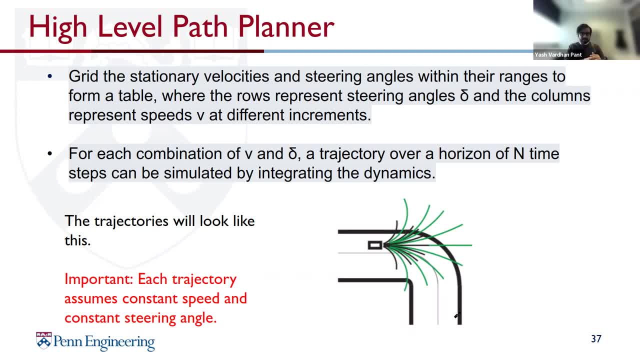 trajectories that could look, for example, like the ones shown over here in green and black, and some of them are going along the racing line, which is the line in the center that we should care about. so let's call this the oops. sorry, this is the center line along which you're going to measure progress. 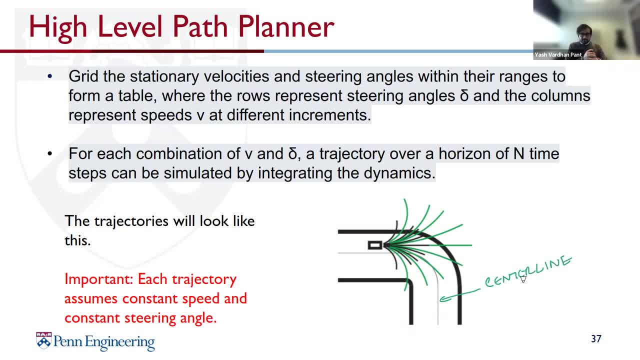 and so some of these trajectories are better than the others. when it comes to making progress along the center line, some of these trajectories are better than the others. trajectories are also pretty bad. they're infeasible- that you won't be able to stay in the track if you. 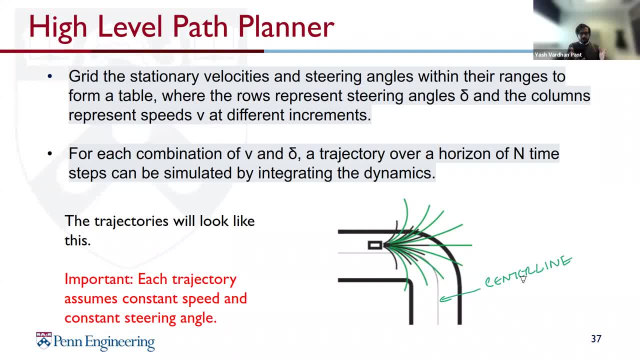 try to follow them anyway. um yeah, an important point is that each trajectory has constant speed and constant steering angle, because you're just doing a forward integration by picking one point in your discretized grid of velocities and angles, but again, this is just one heuristic to generate. 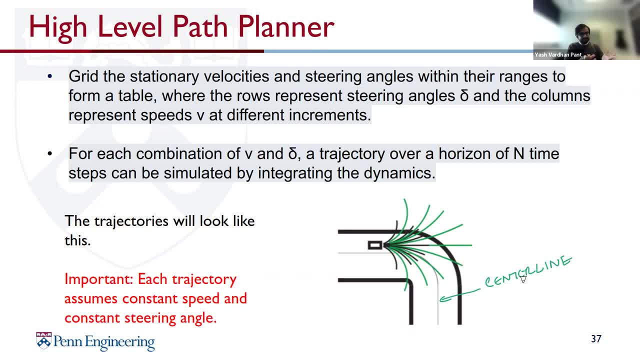 a high level trajectory. you could use rrt star with non-holonomic dynamics for your car. it would do something similar for you. so yeah, at a high level, you've generated some trajectories. the next question is: which trajectory should i pick? and the question after that is: how do i track it? 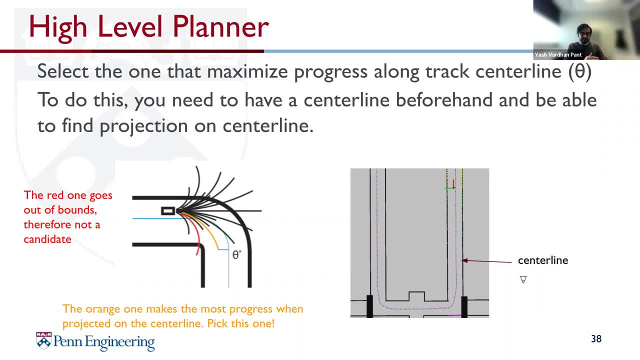 so the first question- how do i pick a trajectory? is first, you of course want to maximize a notion of progress along the track center line, so theta star over here is, uh, the projection of the best trajectory onto your racing line. theta is a measure of progress that's going to be from. 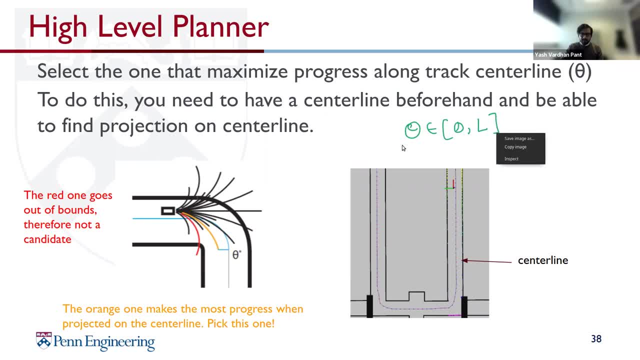 0 to L, or sometimes from 0 to 1, where 0 means you're at the start of the track, L means you've come all the way around and are at the finish line, But you need to have a center line beforehand. 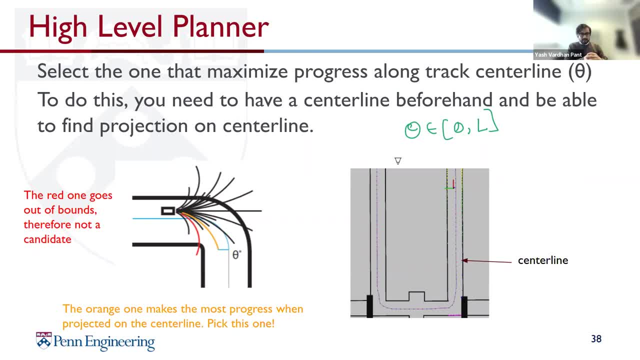 of course, in order to be able to do this. And then you see you have multiple trajectories over here, Like, for example, the black trajectories. they're fine, Let's focus on the red and the orange one. The red one over here, of course, is infeasible with respect to your track, So you 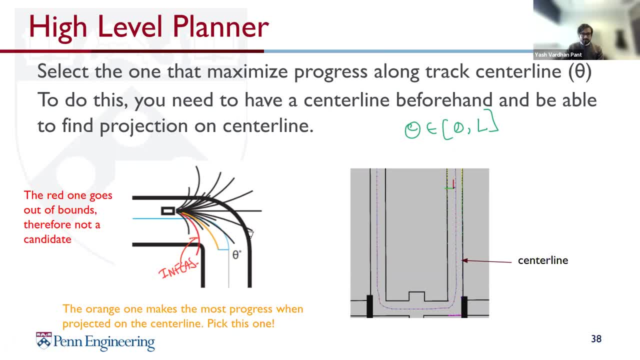 definitely don't want to follow that one. The orange one, on the other hand, is what we'll pick as the best one. Maybe it's not the optimal one, because we had gridded our space of angles and velocities, But you get one of these trajectories that we say is the best or makes 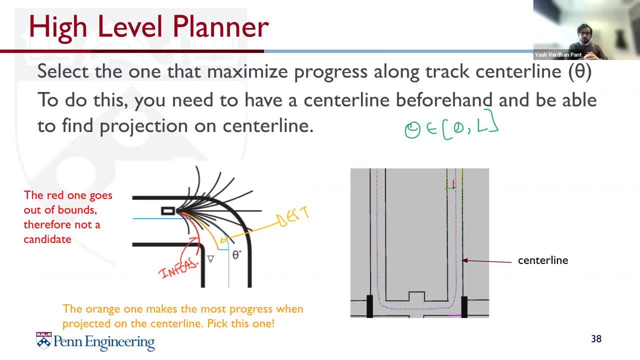 the most project, makes the most progression when projected on your center line, And we'll pick that as our candidate trajectory. So now in our hierarchical planner, at the first level, we have essentially picked a trajectory by generating many and picking the best one. that 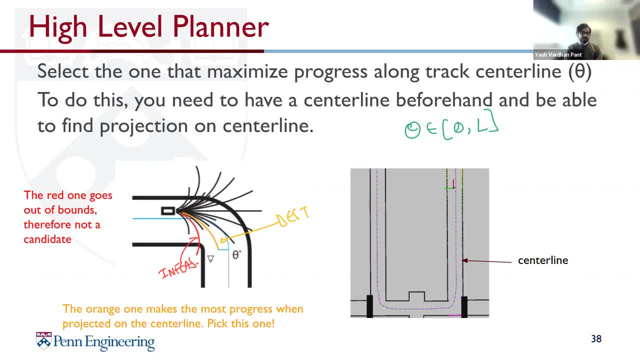 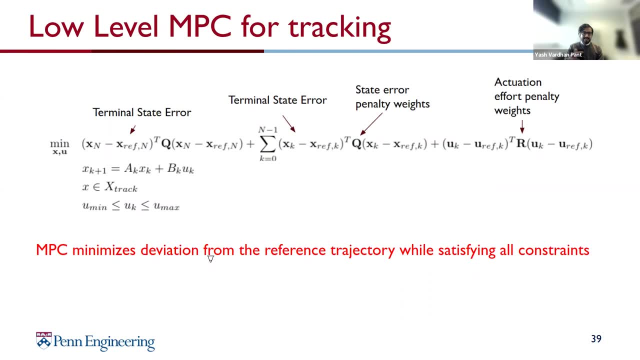 makes most progress. And now, given this trajectory, we can take MPC then to follow the trajectory. So we can write down the following MPC where xref essentially are points along our trajectory And points along our optimal trajectory, the one that we found previously, And so: 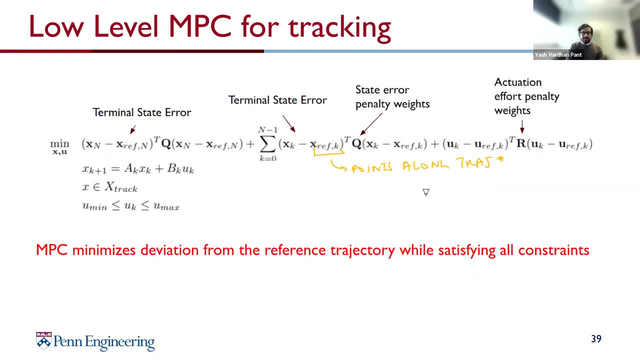 we penalize essentially deviation from that. Take into account your system dynamics, your track constraints, your input constraints, and then you solve the optimization. So you're going to. MPC is essentially then going to track your trajectory. It's going to minimize deviation. 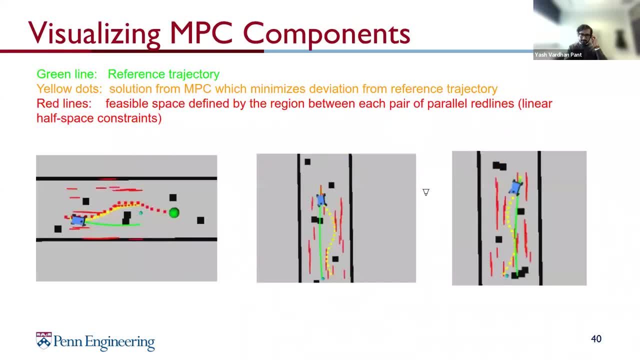 while satisfying all your track constraints. One example of that is shown over here. For example, green line is the reference trajectory, maybe the best one that makes progress along the centerline, But you also have to take into account obstacles. now to something we weren't talking about. 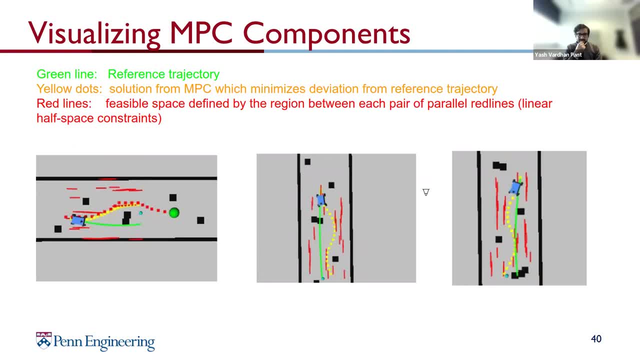 previously. So green line is your reference trajectory. Yellow dots are solution from the MPC which minimize your deviation from the reference trajectory while also respecting your constraints. Now your constraints also include obstacles, And red lines are feasible: half spaces defined by, essentially, regions. 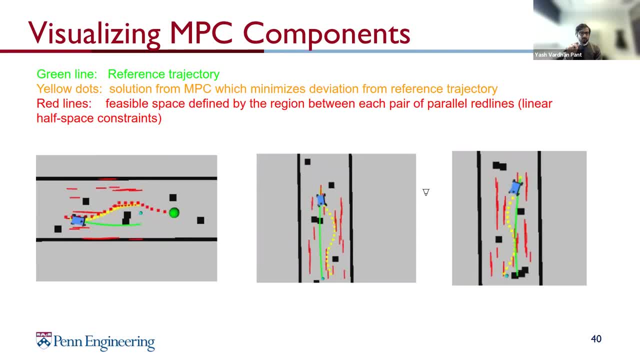 between convex regions, between these half spaces, are what you can pick as constraints for your MPC, So you could have multiple MPCs to be solved over here. But again go to the reference or the archive paper to find out more about what's happening in here, for example. But yeah, you. 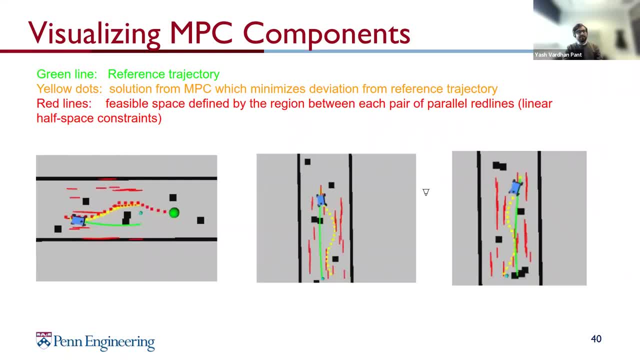 could have a high level planner to generate trajectories and your MPC at the lower level to follow those trajectories in the best manner while also being safe given your constraints. So that's the first of the hierarchical method for using MPC, essentially to track trajectories to race around a given track. 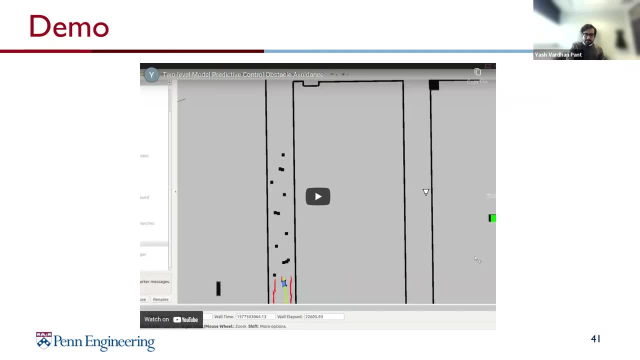 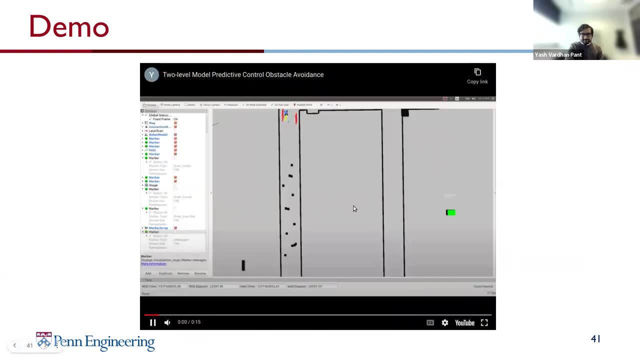 So maybe take a look at the demo again that we saw before. So this is again the two level, or the hierarchical MPC, And in red you have your track constraints. Green is the reference, yellow is the actual line that you're following. As you can see, there are these different constraints that 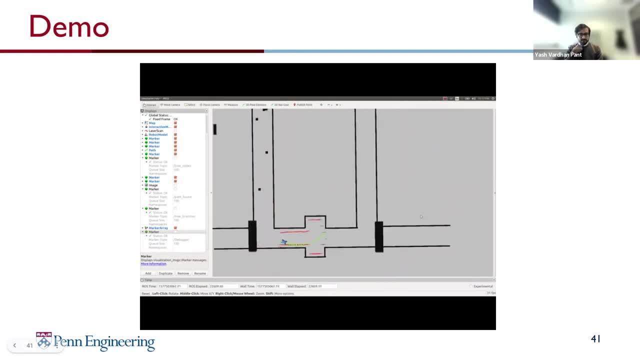 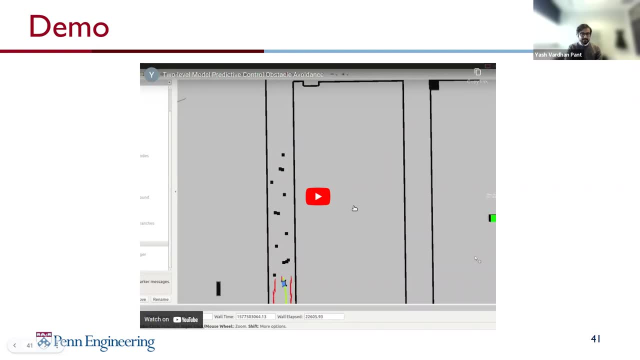 you can pick from- And again there are some heuristics to pick the right ones- And then you stay within those constraints, the tightest bound within those constraints, drive around the track while being safe. So this is one method that you'll see in the paper. I think it's the first. 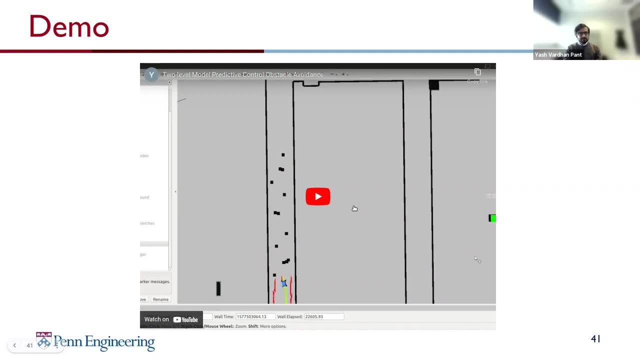 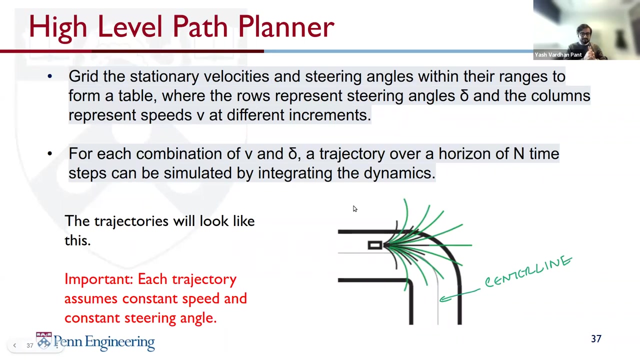 method covered in the second section. Any questions about MPC for this hierarchical MPC algorithm so far. Could you please explain more about the green line, the reference trajectory, how I mean the definition of that. Okay, So the green line is going to be one of the best, it's going to be the best trajectory. that 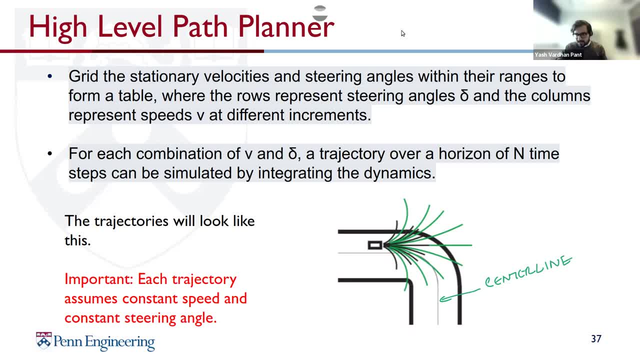 we generate at a high level. So maybe let me sketch out the architecture for what it looks like. You have a trajectory generator or a high level planner. It's going to generate a bunch of trajectories, So it's many trajectories, as shown over here. 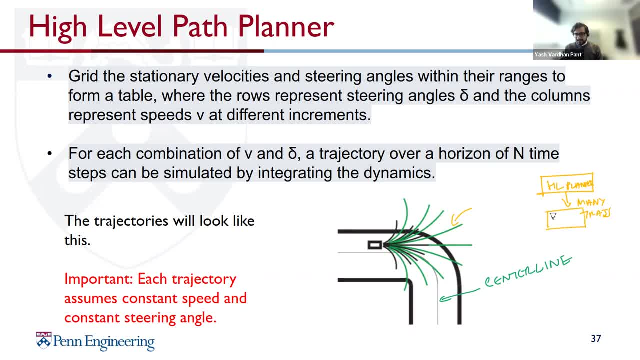 right, It's a bunch of trajectories. You pick the best one through some heuristic, which could be, for example, projection along a center line, And you send this trajectory as a reference for MPC to track. Now, generating these trajectories could be through many ways: RRT star could be one, or you could follow the heuristic presented. 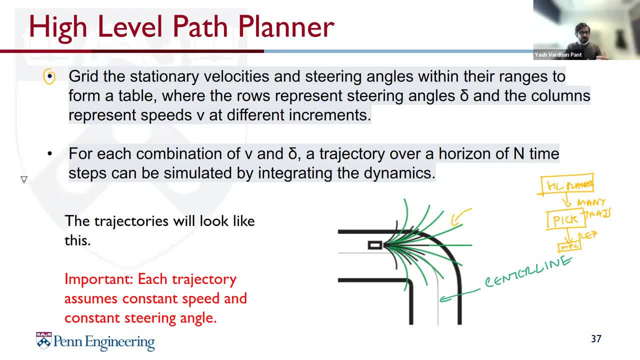 in the first bullet point, which is: take your possible velocities for the car, discretize them, let's say, at intervals of five miles per hour, 10 miles per hour, 15,, 20 miles per hour. Take multiple steering angles, For example. 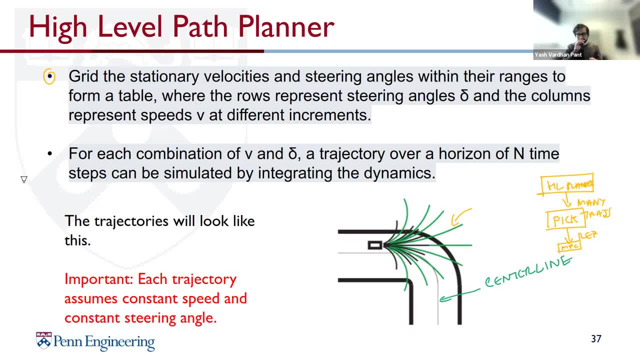 going from minus pi by three to plus pi by three in some increments of, let's say, 10 degrees, And essentially just forward. simulate your dynamics for that, which you can do because you know the dynamics of the car, If you know your constant velocity, constant steering angle. 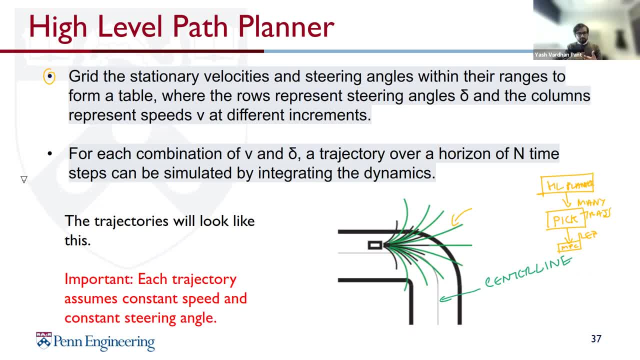 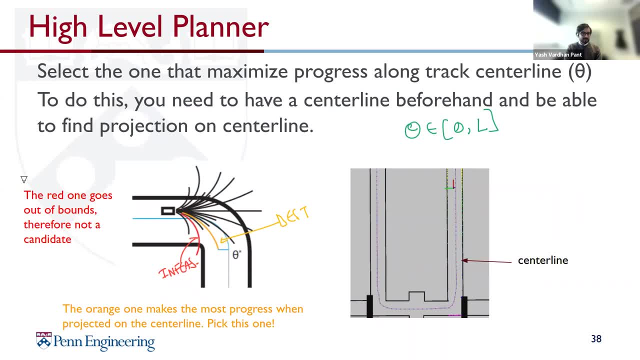 you can kind of see what these trajectories would be. Plot all of them, project them onto the center line And, as the next slide shows you, the one that makes the most progress along the center line is going to be your reference trajectory for your MPC to track. 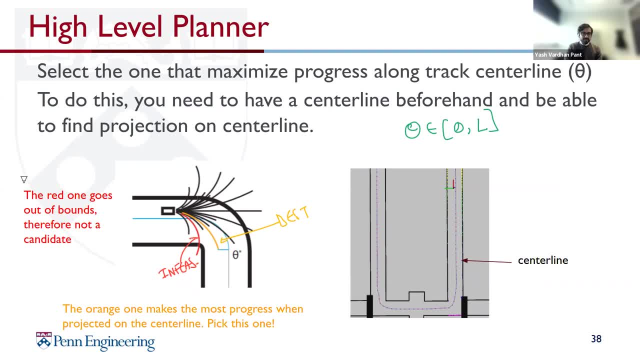 So again, it's one heuristic. sure you can come up with something better, but this is how you would generate your high-level reference trajectory. Does that answer your question? One more, some more questions? Yeah, go ahead. In the earlier slide I think there are some of the darker black lines. is there any? 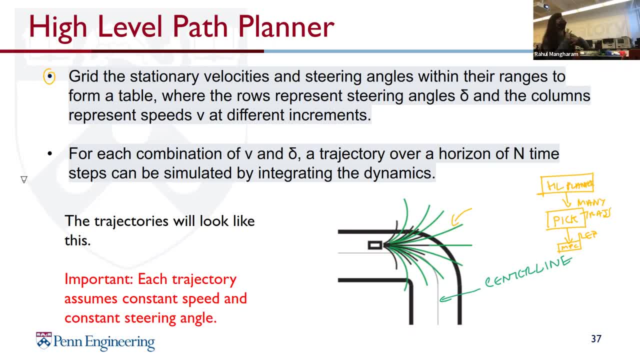 significance to those why they're shorter: RRT, star … KIC … TK for different velocities. so think of it as I've discretized my velocities into two points like five and ten miles per hour. so the black lines are five, green. 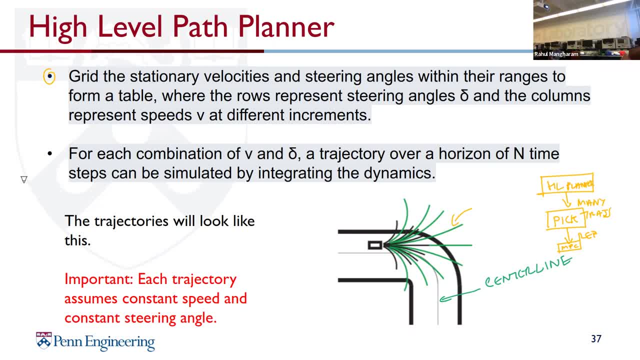 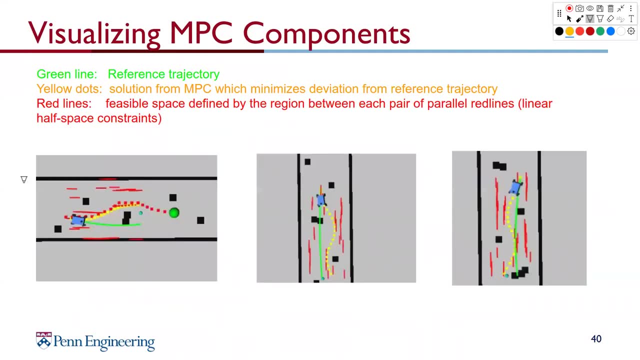 lines are ten. yeah, let's go. can I ask a question? yeah, go ahead. so for the red lines which you show in the simulation, can you go to that slide? I don't. yeah, okay, so far for the red lines that you show in, I mean in all the pictures are. 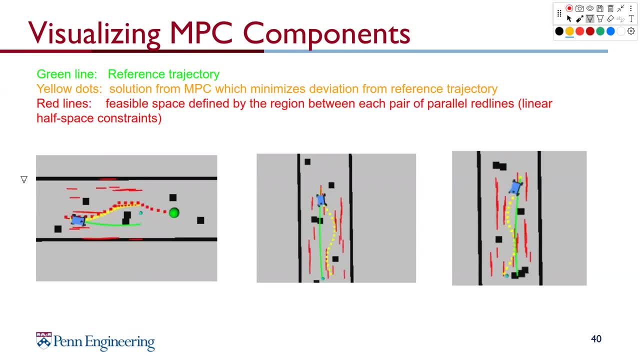 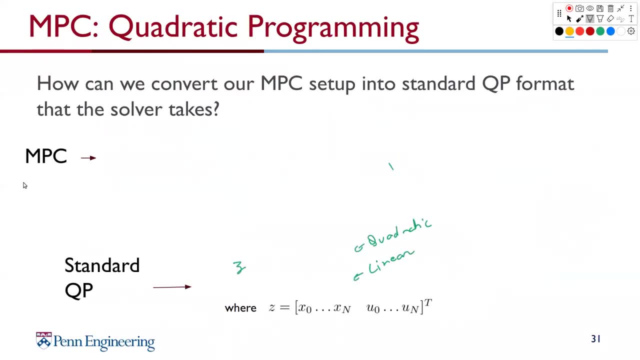 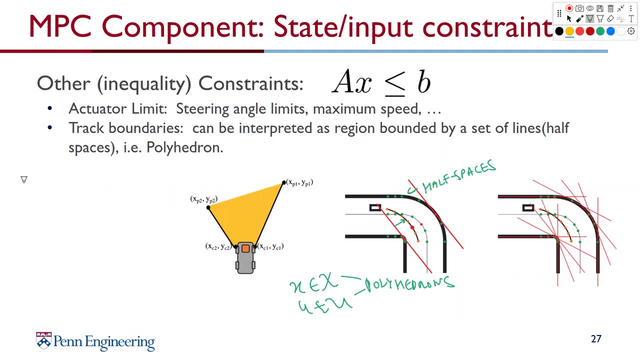 this so that you said half space constraints, but I think on the on the slide 27, could you go to 27? so the half space constraint on your mid picture it seems like it's the projection of your center line, point red dot in your center line. but it's just lies directly on the. 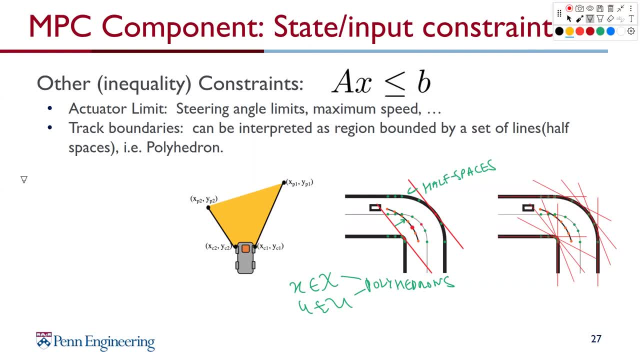 track. so why it's? I mean in the simulation. it does not lies on the track, it's on the, I mean on the, somewhere inside the track. well, because the simulation is using some other kind of heuristics, but anyway. so these constraints, for example, it's like 27- they come not from the. 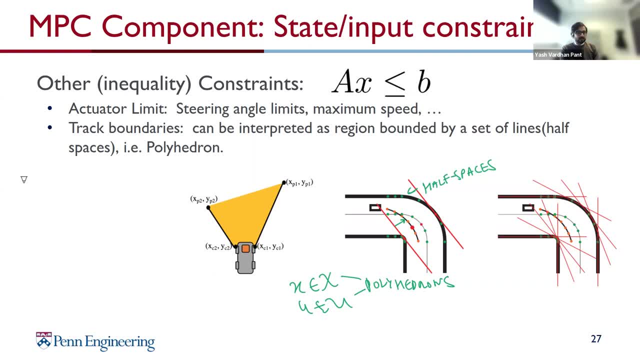 center line, but they're more. you're just drawing the tangent to your edges of your racetrack and those tangents are going to define lines that you should stay within. again, this is one heuristic. for more details I would refer to the archive paper. so if we don't have time, 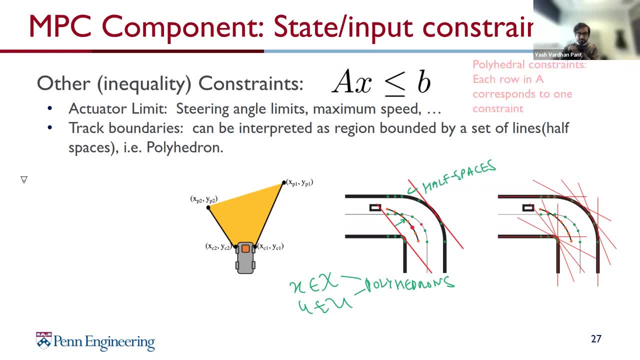 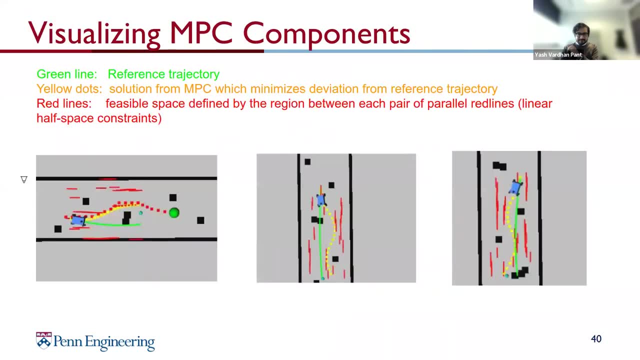 to go into the details of what's going on in there. what's happening in the simulation, though, is you have those multiple lines because you have these different obstacles, so you have all of these different half spaces. you also see that you have some of these lines that are on. 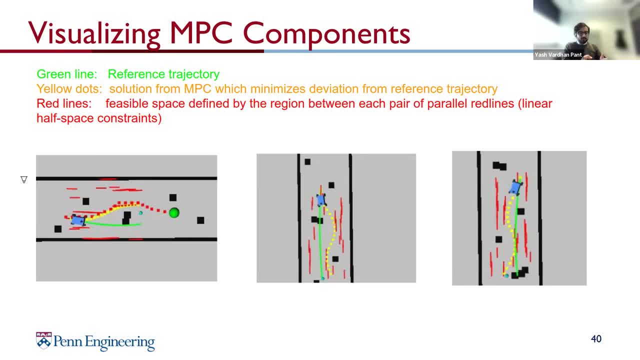 the track boundaries as well. so again, part of this is visualization. these lines aren't visualized perfectly. now, if you take the intersection of all of these half spaces, you'll see that a bunch of these constraints are redundant. for example, if I talk about this constraint over here and this: 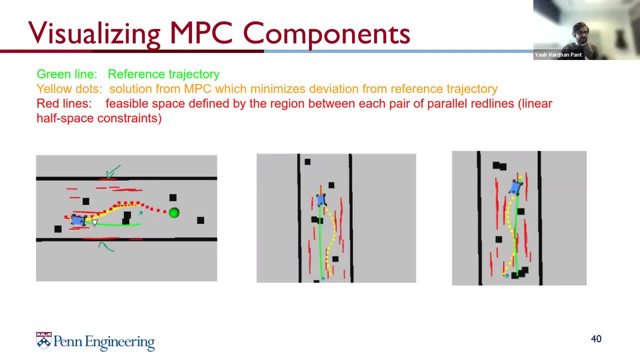 constraint. these constraints are redundant because you have tighter, parallel, pretty much parallel lines like this one and this one to consider right. so what's kind of shown over here is that the heuristic is generating a bunch of half spaces that you should be within. you'll be within the intersection of 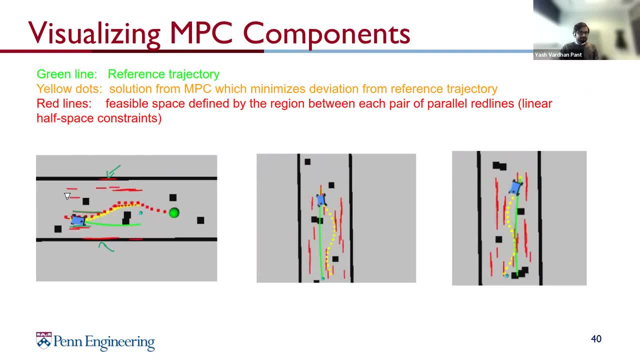 them, which is going to be the tightest possible space. okay, so, and then as you move forward, you're going to recompute these lines and stay within, again, the tightest possible space over here. okay, same um purposes. so it does seem like, uh, going back to the receding horizon problem. 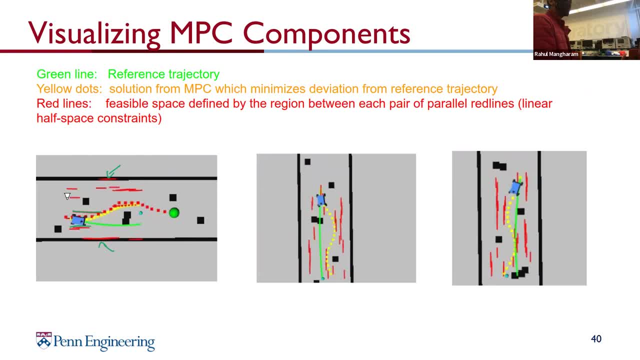 uh, we are, we are, we are optimizing over a time interval, right, so, like, is there a heuristic on what could be, like what should be that time interval taken for me to optimize upon? because it seems like, since, if we are going for feedback, the the smaller time interval I take, the 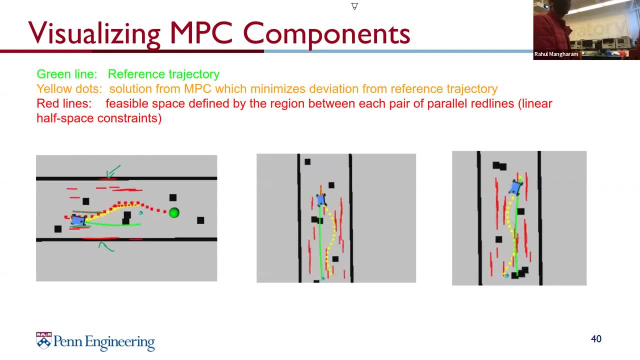 better it is, since I'm just, uh, going back to the, I mean, since I'm in forcing that my state estimation for the state, for the state at the time I I apply, my next control input should be the state I start with. so I see your question, um. 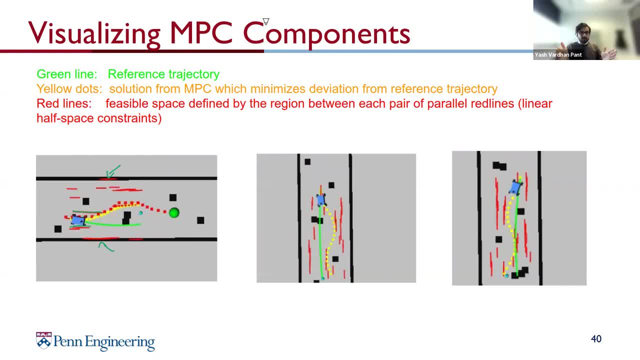 right. so first thing about NBC is that the longer the time horizon, the better your performance, because you know, absent any disturbances and mismatches, you're predicting for a longer time and so you can take actions that are going to be optimal- um, you know, over your entire horizon. 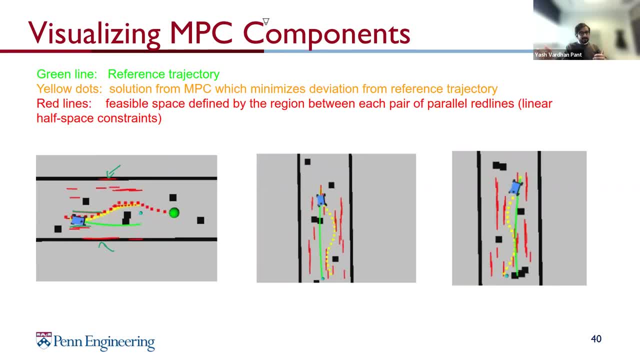 essentially, you want to have infinite time, optimal control. now it might seem that a smaller time horizon is better because you're using feedback, but that's not necessarily the case. in order to pick what the right horizon is, it depends on a lot of factors. there's heuristics, for example. 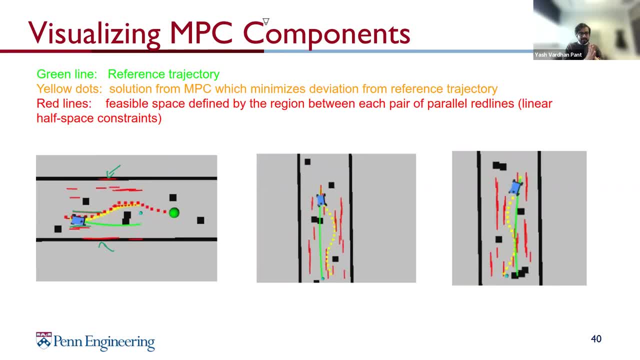 on. again, it depends on what kind of estimates of disturbances do you have. for example, you might be limited by your sensor data, and so that may kind of artificially restrict how big your horizon can be. another thing to consider is your computation time, which was brought up by a student earlier on. 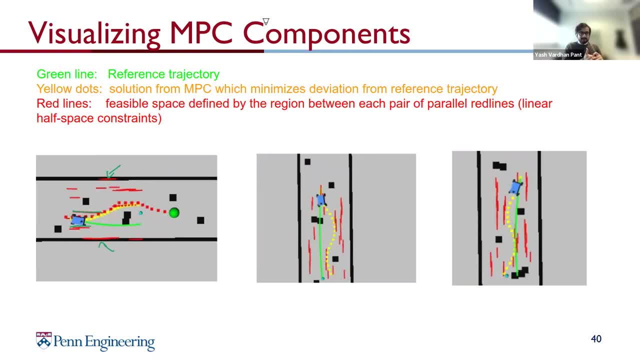 um. the longer the horizon, the more optimization variables to deal with and so the slower your optimization is going to be. for example, if I solve an optimization with 100 over 100 times step horizon versus a 10 time step horizon, 10 times of horizon is going to be much. 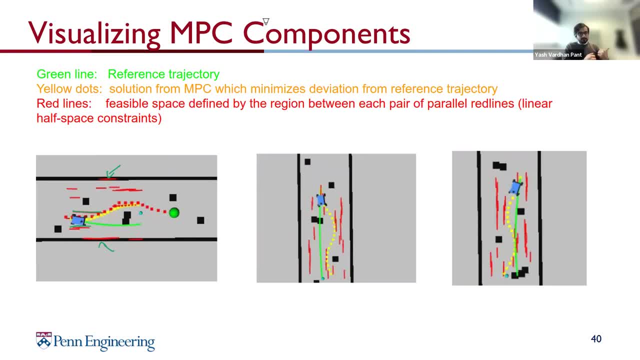 faster, so your compute power, your prediction and also your model mismatch. these are three things that define how big your horizon can be. and the third thing, the fourth thing over there is also like what kind of formal guarantees you're trying to get from model predictive control, and that's beyond the scope of this. 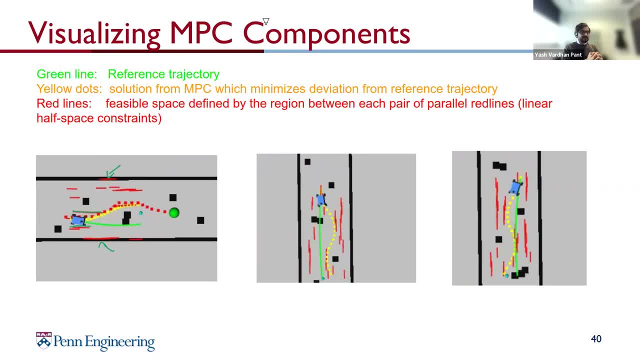 lecture. so, um, essentially, try to keep it as long as you can computationally handle. so, uh, so in case of like, let's say I'm I'm just building it for racing and I don't care how erratic my, my trajectory is. I just wanted to be. 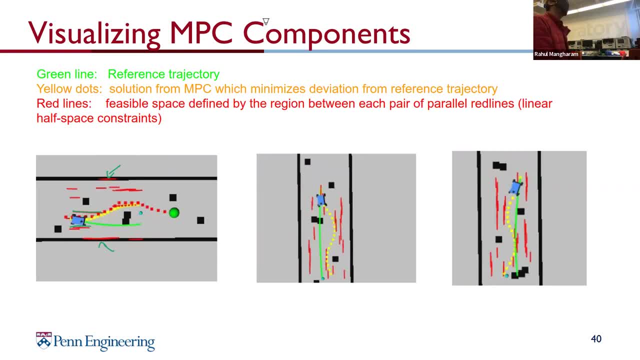 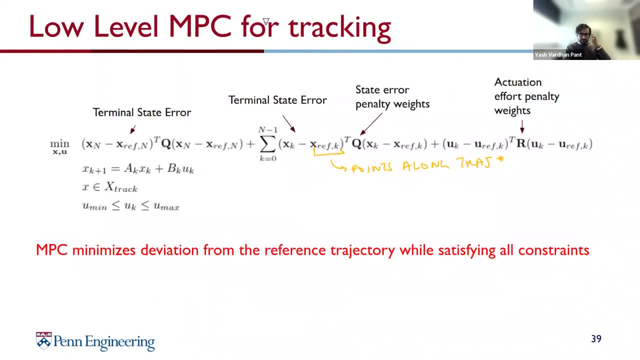 fast. so in that case a smaller one would be better. it would be better in terms of computation time. it won't. it still won't be better in terms of performance, because if you go back to the MPC objective- right, let's say you're trying to minimize um. 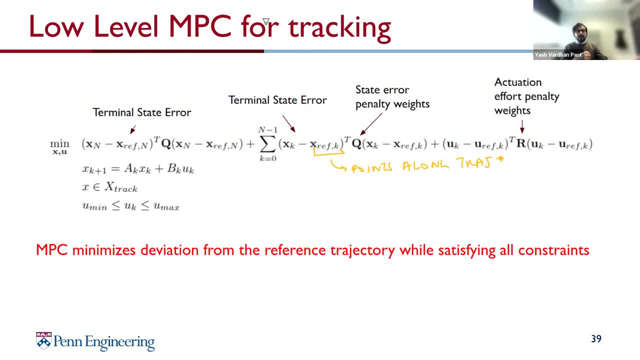 deviation from a reference trajectory. the more look ahead you have, the better you'll be able to do, because you know you come up with maybe smoother trajectories that stay close to this, that converge more quickly to the reference, rather than, if you have a small look ahead, you might have jerky. 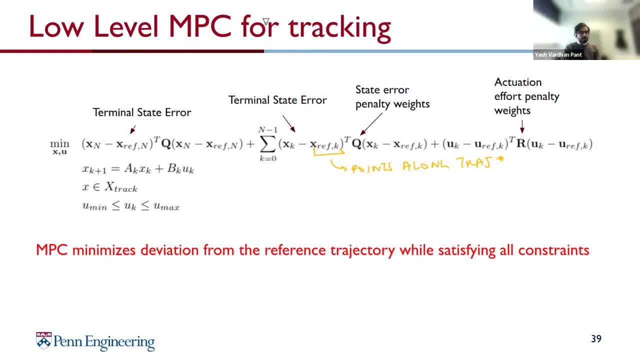 trajectories that move around and then convert slowly. so again, um, longer horizon, better. also, is there a reason why I'm, why I'm having a penalty for my control input? it's just saying that I don't, I don't want to put some effort, or yeah, so this is for, uh, the first thing. 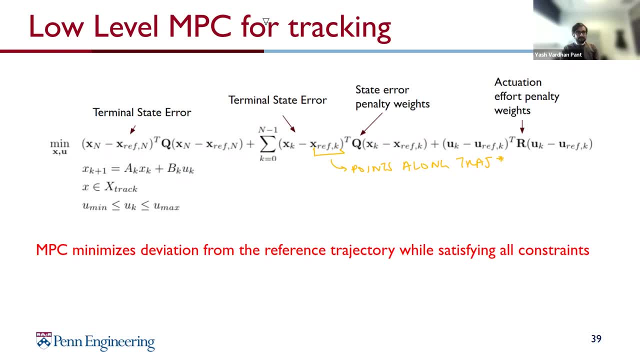 is. this is for the stability of model predictive control. if you don't have any penalty, then you will have large control actions that might lead to very oscillatory behavior when applied to real systems. also, when you do the formal um stability analysis of model creative control, you realize that r actually has 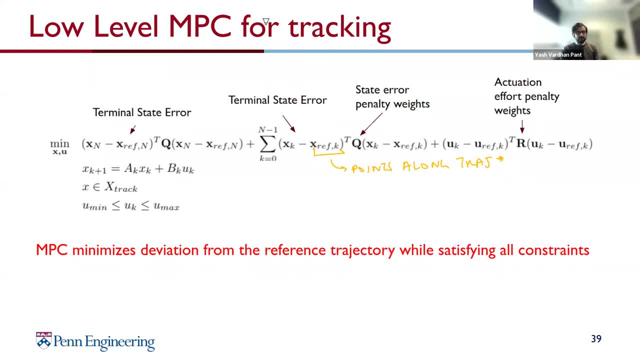 to be a positive, definite matrix. if you've taken an optimal control class and done some linear quadratic regulator, you'll see have a similar requirement on the r matrix in LQR. so it kind of comes from that that you'll be able to do that. comes from that that you want to have. 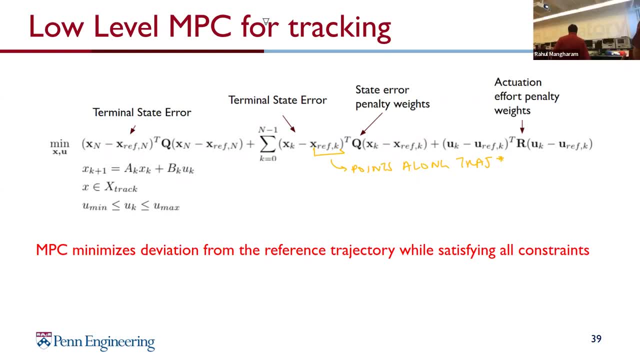 stability of the system. thank you, thank you, some more questions. I just wanted to ask what would happen if the reference trajectory is not feasible? uh, it's not feasible, as in it's going into a wall or something. yes, well then, if you have imposed the feasibility constraint in here, um? 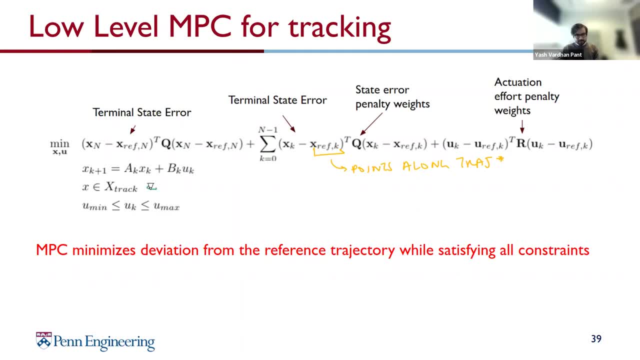 sorry, my pen has stopped working for some reason. there we go. let's say you have your track boundaries in here, then what you will essentially come up with is a trajectory that tries to track your. your actual trajectory will try to track your reference as close to possible while staying within the track. 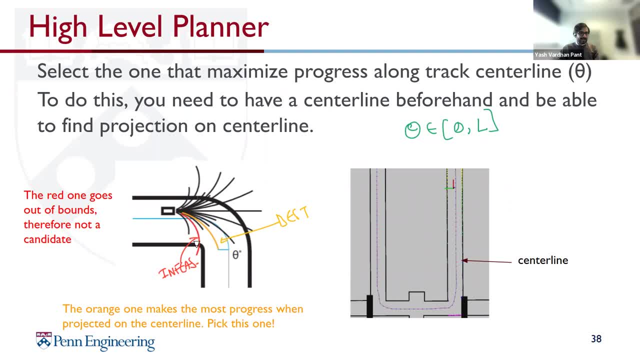 if I were to kind of sketch it out. let's say you're trying to track the trajectory in red right, one of your candidate trajectories could be- I'll use the color blue to sketch it out- this could be a candidate trajectory that MPC makes, or this could be a 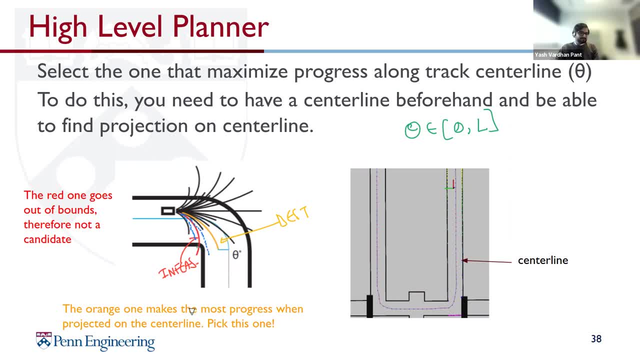 candidate trajectory that MPC makes, so it's going to be optimal with respect to tracking the red line while respecting the safety constraints. so it's kind of on you to impose both at a high level. and if you impose it at a high level, great, if not at the 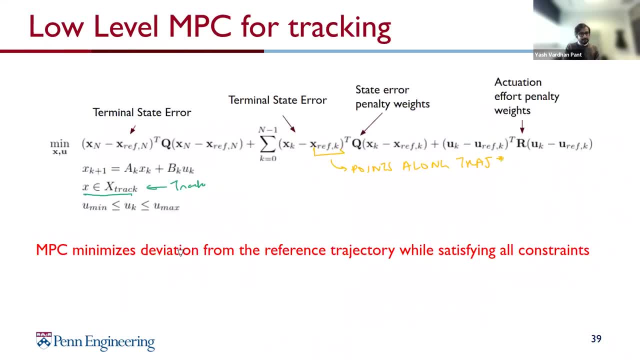 low level. you should impose that your track boundaries are respected. even if we have an obstacle that's blocking the track, we might turn around and go the other way. um, in that case you'll have to kind of find the right constraints, for example in the uh, if you look at the obstacles over here, 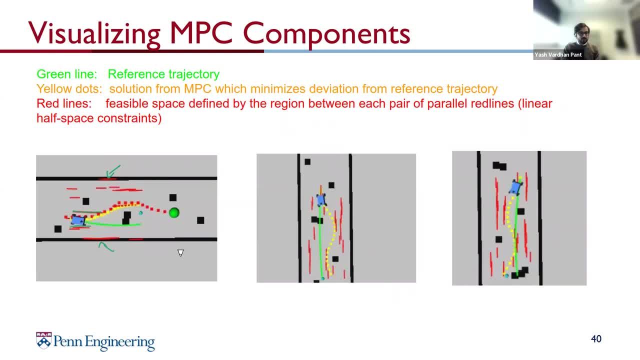 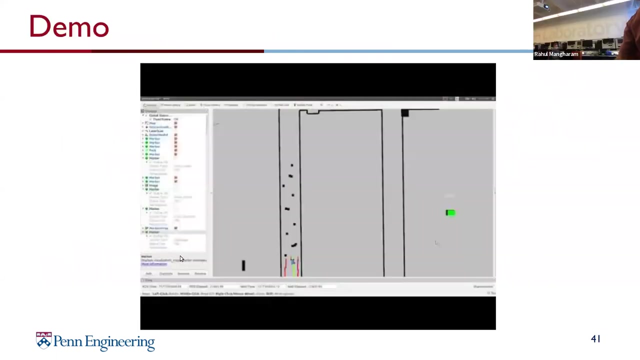 and you see, there's a bunch of candidate constraints and of course we pick the tightest one, but then it's on you to kind of figure out how you will compute these constraints. any other questions? no, these are great questions. yeah, keep them coming. all right, great, uh, right, so we just saw. 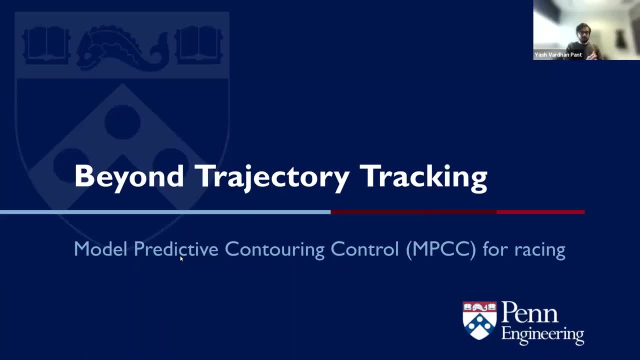 this demo. so so far, what we've seen is MPC for trajectory tracking, which is a high level trajectory generator, generates a bunch of candidate trajectories, could have a bunch of issues with them, but your then your low level MPC is going to track those trajectories to the best of its ability. 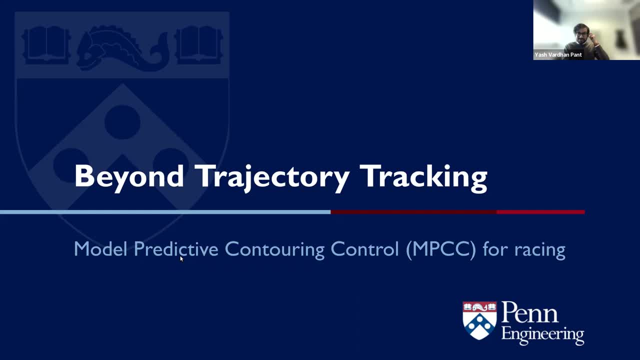 while respecting your constraints the way you've imposed them. first, constraint design in MPC is a big problem and it's very subjective. so it comes down to what problem you're dealing with and you know what kind of domain expertise can you bring to it. but of course we can also use MPC then. 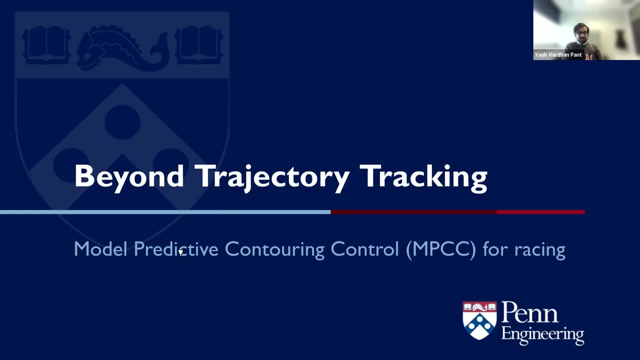 for not just trajectory tracking but for generating candidate trajectories that are correct by construction beforehand, rather than coming up with trajectories that maybe can't be tracked perfectly or hit a wall at a higher level. get rid of the high level controller and instead come up with a formulation that 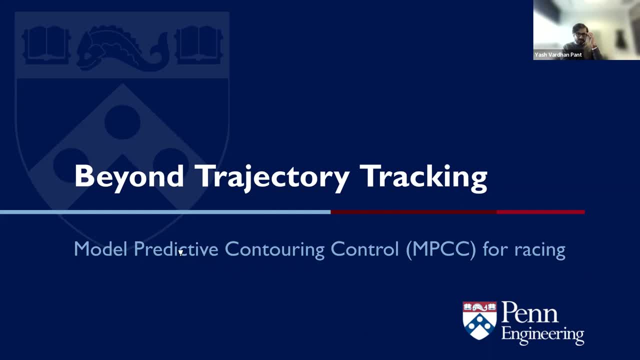 generates trajectories and tracks them at the same time- essentially a local planner. and in order to do that, we'll refer to the paper again that does model predictive controlling, contouring control or MPCC for racing. this is a paper based on the 143rd scale or car. 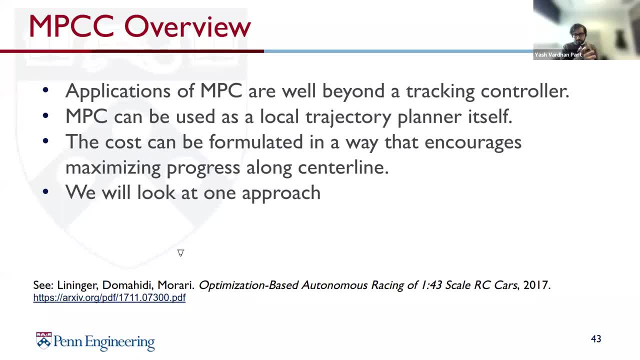 cars. again, you'll find the link in the slides. it's actually: yeah, it's the reference over here. so yeah, MPC, of course, in terms of racing, can do a lot more than just tracking control, not just in racing but for many autonomous systems, including like in my. 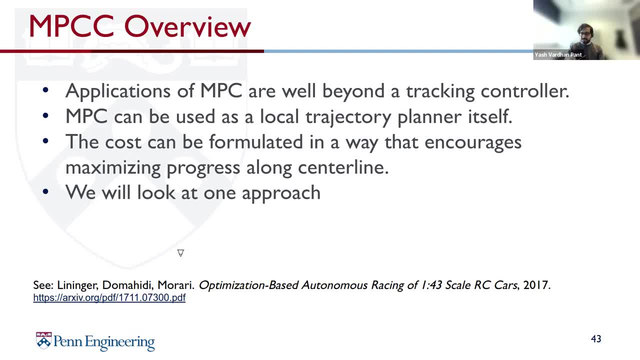 research. with our aerial robots we generated a bunch of trajectories for very complex looking specifications using an MPC like algorithm, so it can be used as a local or even a global trajectory planner. the cost can be, of course, formulated in a way that it still encourages maximizing progress along the center. 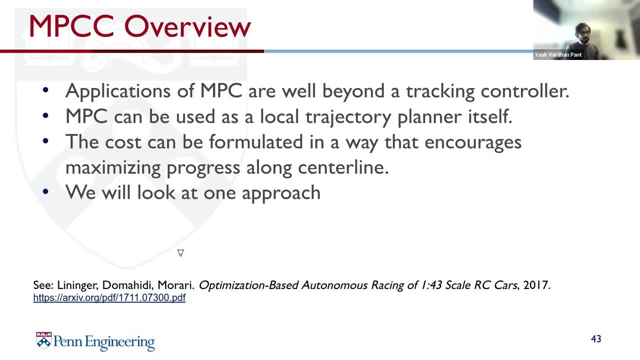 line and constraints should be for safety. and we'll take a look at one particular approach that essentially kind of exploits the geometry of the track and the car to formulate an MPC that will generate local trajectories for you. that approach is called model predictive contouring controller- MPCC. 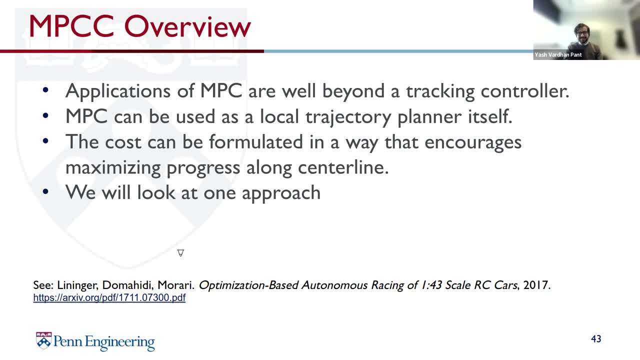 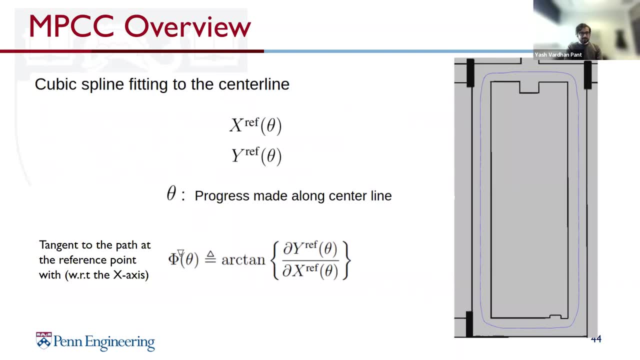 if you go to the reference, it's the second method in it, I think section three or section four. so it does a very good overview of what's happening inside MPCC. the idea is first that you're going to do now, think about trajectories, so take your center line. 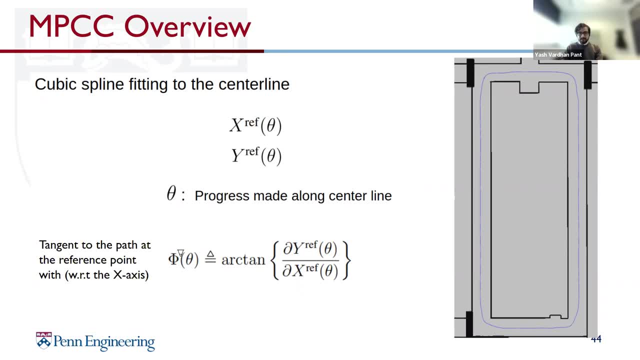 and do a cubic spline fitting to it. so theta again is a parameter that talks about progress made along the center line. it's going to be between zero and L, but L is the again all the way back to the racing line, zero as your starting point. so what you want to write down is x ref. 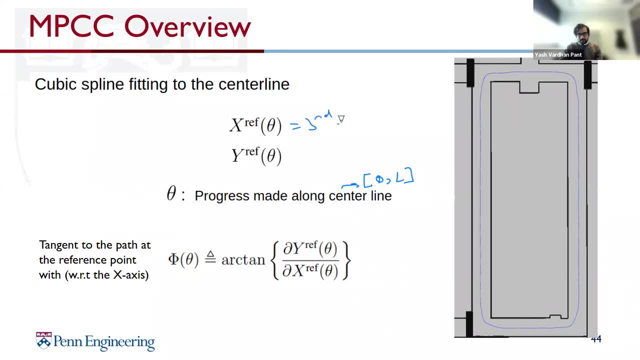 and y ref. so these are third order polynomials of theta, along with some, a bunch of constraints, similarly for y as well, and so these third of the polynomials are what are going to define your center line. so think of this as x ref and y ref parameterized by theta. so let's say this is your start. finish straight so. 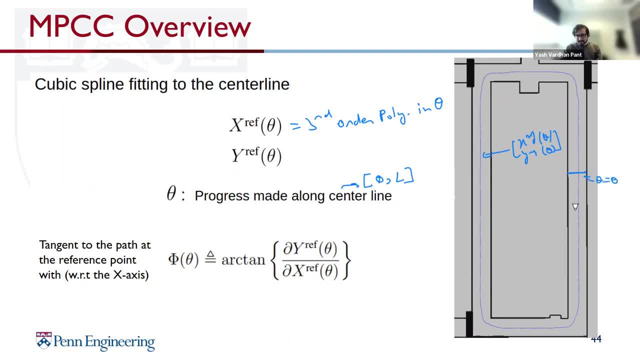 you will have theta equal to zero over here as you go all the way along the track. come back, you will have theta equal to f as you reach the finish line. so as you increment theta, if you evaluate x ref and y ref, this polynomial is going to give you the racing line that's going around. 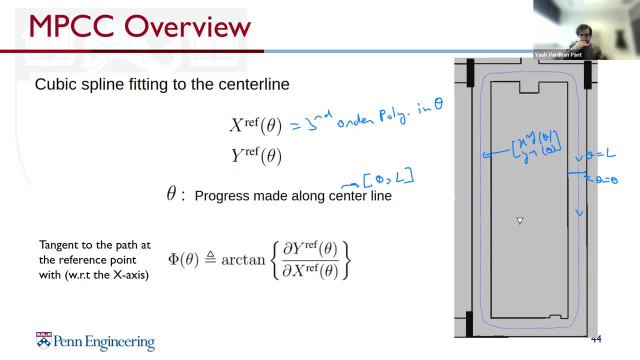 what looks like the m lab and the other spaces in the second floor of levine. now, with this kind of formulation you also get a good kind of a reference orientation to track for free, which is phi of theta, which is a tangent to the path at your 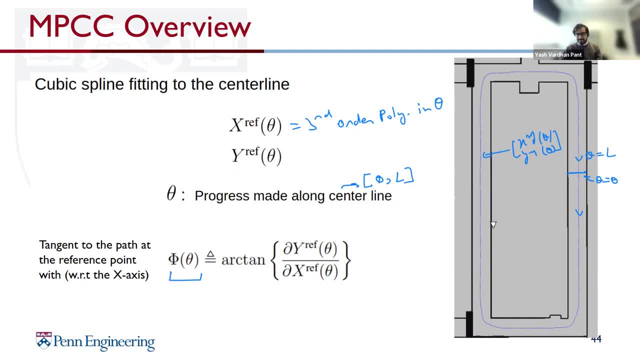 reference point and it's going to be the angle, with respect the x-axis. so if there were a couple of axes, this is your x-axis of this as your y-axis. so again, first we'll start off by just fitting a cubic spline to our center line and again this: 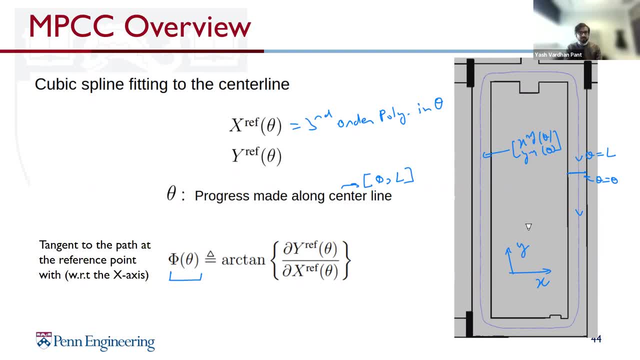 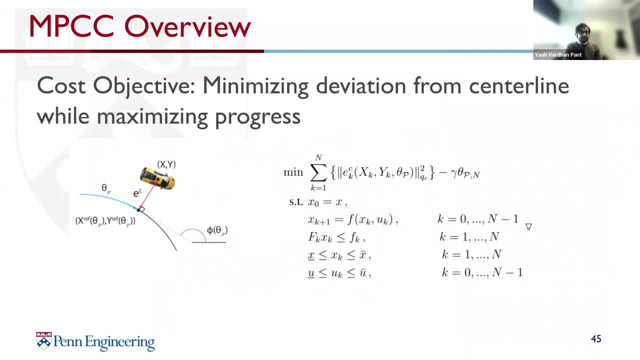 may not be an exact fit to the center line because you're restricted your splines to be third order polynomials. this is what we'll start off with. sorry, then. the objective for model predictive control is to minimize the notion of deviation from the center line while maximizing progress, or how far away you are going to go along the center line, which is why 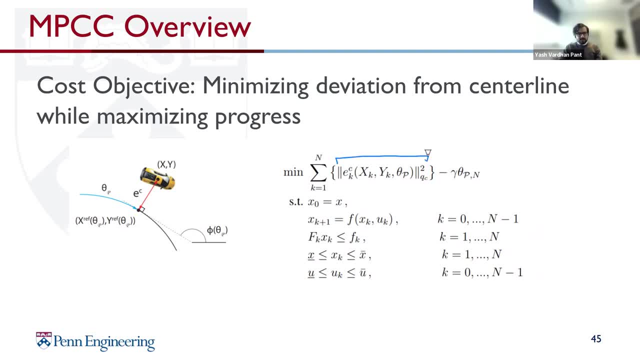 you have this kind of an objective where the first term- and we'll talk a little bit more about what these are- this is your deviation- that is to be minimized, and the second thing is progress- that is to be maximized, which is why you see you have a negative sign over here, because you 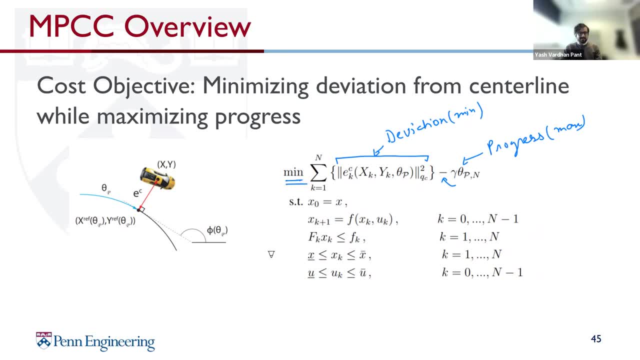 essentially want to maximize it, but on the outside you're solving an optimization that has a min on it. so you know, minimizing a negative number, a negative function, is the same as maximizing the positive version of that function. gamma greater than zero is like a trade-off parameter. 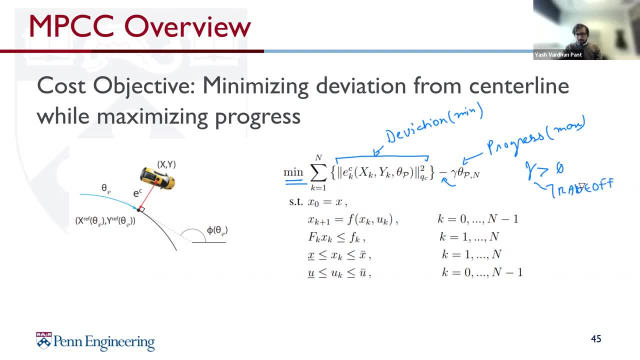 over here. it tells you how much do you care about making progress along the center line, to staying close to it, because you could be very far away from the center line and make a lot of drastic progress. but then you know, maybe you're going slower in the process over there, so you 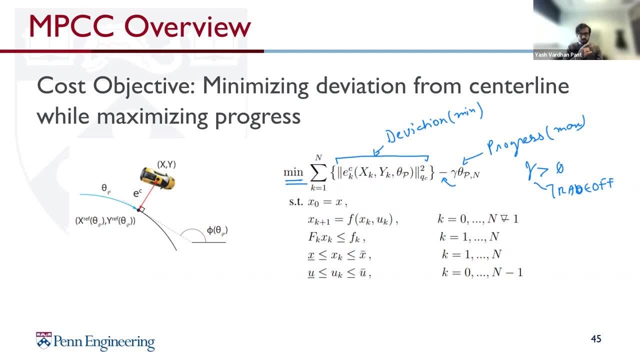 want to stay close to the racing line or the center line and make a lot of progress along the center line and make a lot of progress along the center line and make a lot of progress along the it. so gamma lets you kind of trade off these two things and the constraints then are kind of the 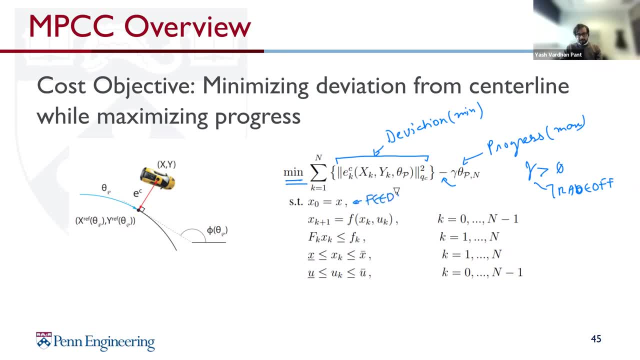 same. you start off with your feedback or your initial state to start off with. you have some dynamics. we use the general non-linear form of dynamics. over here again, we linearize them. you have your constraints for the track. for example, that's given in the polyhedral form shown over here, shown as a time varying polyhedron. 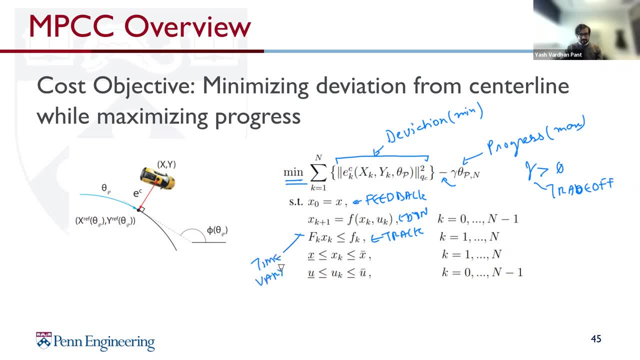 that's given in the polyhedral form, shown as a time varying polyhedron. so these are time varying constraints, as you see, because they're indexed by small k, which is the time step in our horizon, and then, of course, you have state and input bounds. 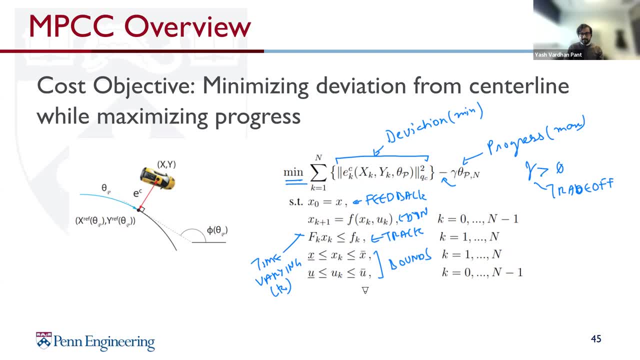 for example for steering throttle, for velocity, acceleration, orientation of the car and so on. so what we're trying to do in mpcc is first come up with a nice representation of what deviation is and essentially then turn all of this into at the end of the quadratic program to be solved that you can throw to a solver. 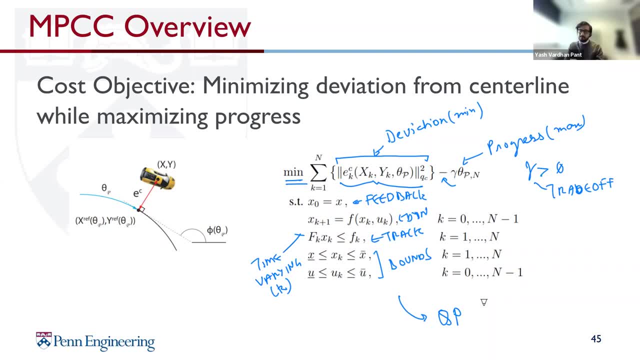 so, in order to do that, we will rely on some geometric constructions, as shown in the figure on the left. so you have a car, you have its x- y coordinate, you have x ref and y ref, parameterized by theta. you have theta p, which is a progress indicator. you have your angle phi, which is 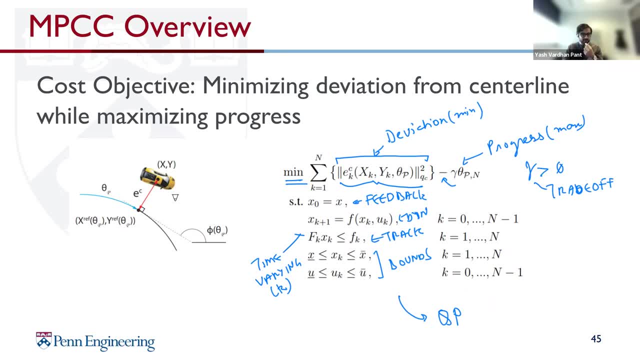 essentially the tangent to this. and then you have two kind of errors that you should care about. so ec over here right now kind of shows you deviation from the center line. so this is, uh, oops, deviation, and what we want to do is come up with a good way to compute what this is, such that you can turn it into a quadratic objective. 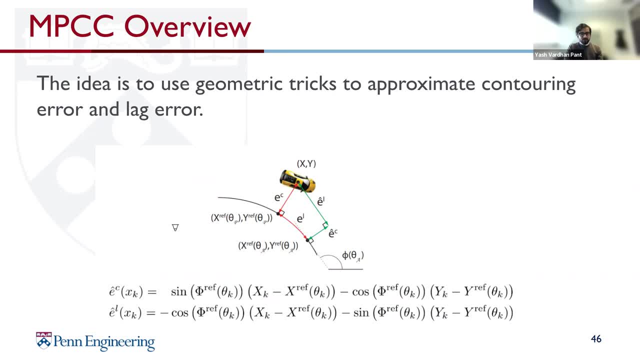 now. you'll find more details in the paper, but the idea is to use a bunch of geometric tricks to approximate two kinds of errors. the first is a contouring error, that essentially contouring error tells you how far away from the center line i am. and the second term that we have is lag error, which kind of tells you how far behind 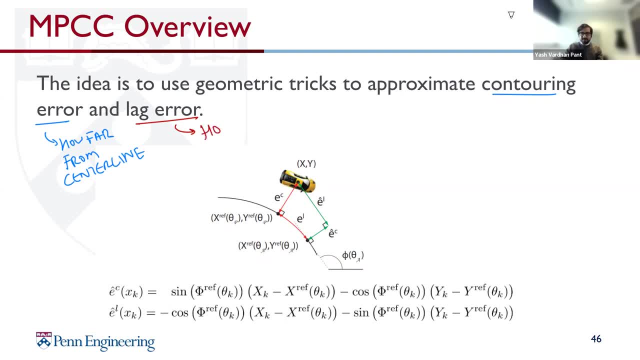 you know some reference, look ahead point or essentially an indicator of progress. pretty much so. if you look at ec and el, ec is your directly, your deviation from your third order polynomial. so this is your third order polynomial. in theta, as we saw before, it's a cubic spline. 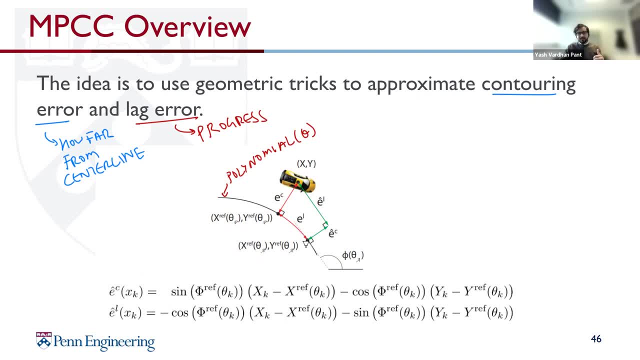 you have ec, which tells you how far away from the spline you are, and you have el, that tells you how far beyond a reference point or a progress point you are as well. if you look at ec and el, these are kind of hard to write down mathematically: ec not so much, but el more so, because it's along. 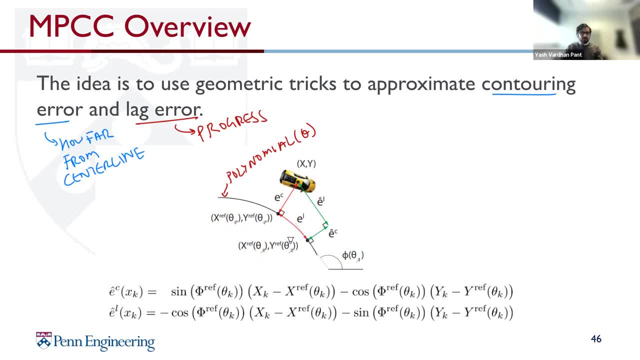 this arc. so what we first do is work with some approximations of this n-th element and then we'll work with some approximations of this error. so we're going to approximate the contouring error and the lag error given by the form shown over here. so this is a. this is going to be your. 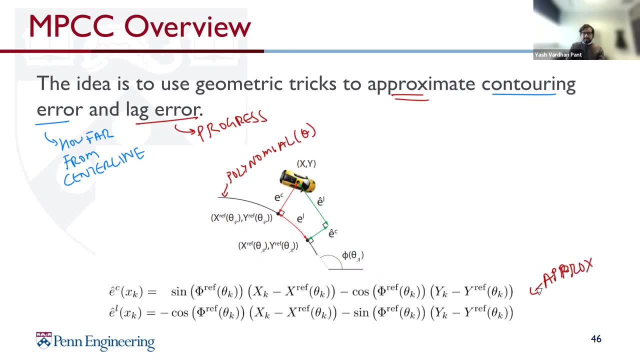 approximation of the two errors. now, as you can see in your variables of interest, theta y and x, this is now a non-linear form. so this approximations are still non-linear. so this is not something you directly want to use in your mpc in the objective. 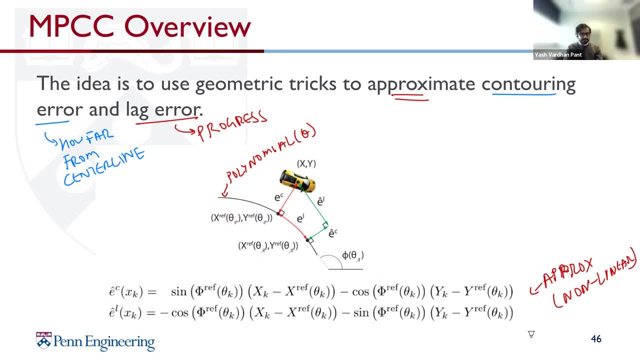 but anyway, if you go, if you go into the paper, you'll see more details on how these things are worked out. and yeah, i guess in the interest of time, we won't get too much into that. so, yeah, you have these non-linear approximations of what these two kind of errors are. 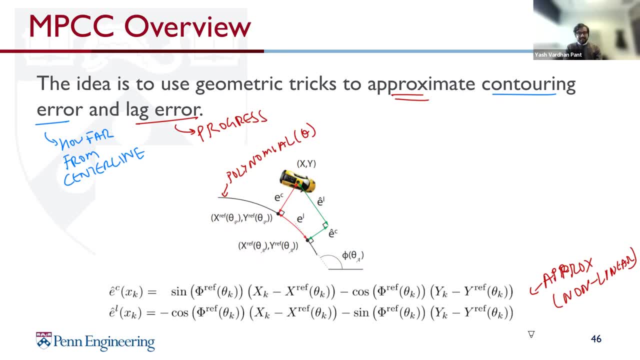 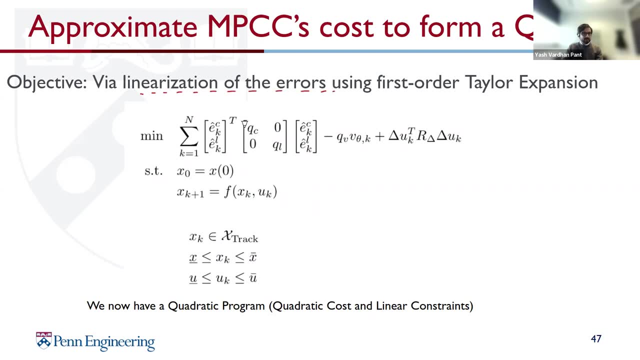 for, you know, closeness to the center line and progress. and then what we are going to do is essentially we linearize those error equations. so we saw those non-linear equations and we'll use first order taylor expansion, for example, to come up with a linear approximation of. 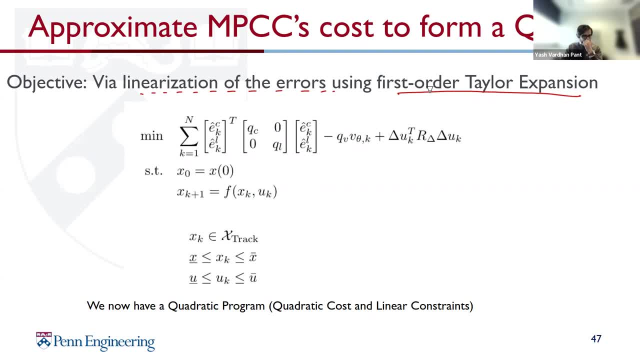 e hat c and e hat l. once we have that linear approximation, we'll essentially turn it into a quadratic objective to be minimized. so this over here, as you can see, is of the form summation of some error transpose q times error where error is a function of your states again. so it's going to be some x transpose qx. that's the first term. 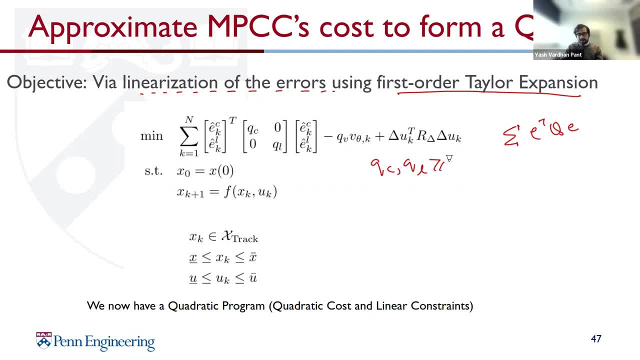 you have the constraints that qc and ql should be greater than equal to zero. in order for this q matrix to be positive semi-definite, you have, of course, your control penalty. so this is your control penalty again: r has to be a positive semi-definite term. and then you have 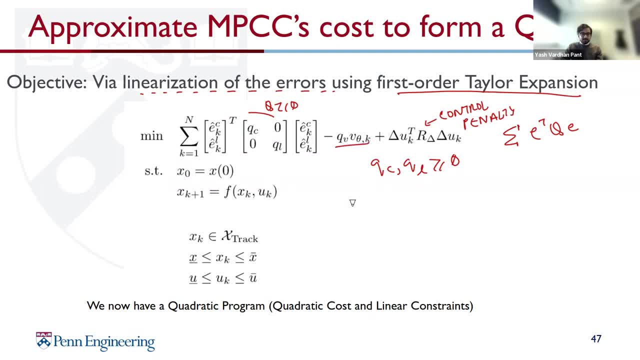 essentially, if you want to go fast, you can kind of maximize your abs, your not absolute value, but your maximize your positive value of speed. so that's kind of what you're trying to do over here. this could also be a progress indicator or whatever you want to use. so again, 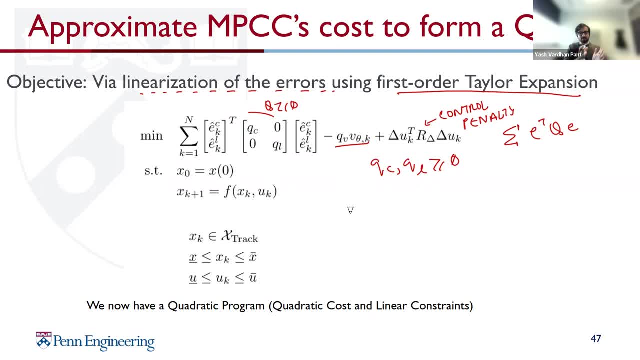 first I'll just set your normal치가 advantage to be direct, so you can see that for your function, set to forced recurrence, the other function you have is inflation. all right. so, for example, if you can't do theuais and in fact you're in charge of a 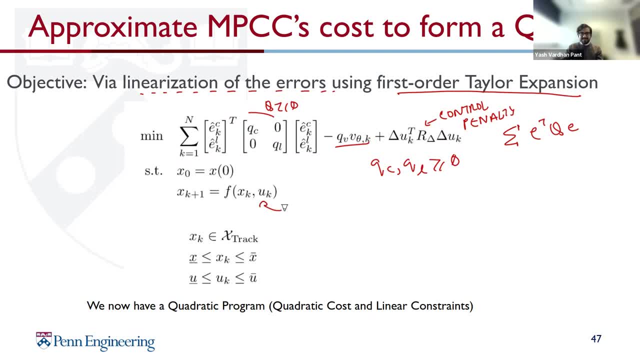 function that you need to simplify your Duck clam specifically over here you can set maybe more than one million dollars those. this function is no longer required, so it's just one of them, just to have one of them, and that's why we're building these. so we think that we have this. 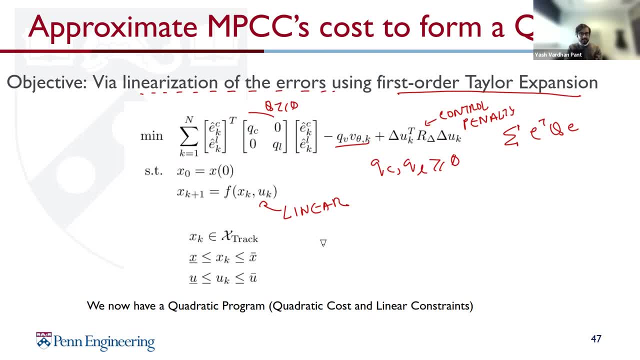 actually calledετεchnology엔, electrical engineering functionality. where, if you were to want data free in a corporation, you have a côté celebrated query. where, if you were to calculate the parts of the framework that will be listed and the económically inside those 同学es column and Compound them, would have a balanced idea of term and 5 times aware of them. 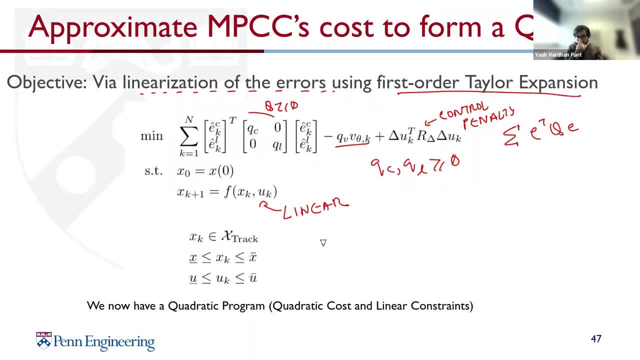 all right, now let's see some other things. so if we set this in the form ofтраf, получилось essentially come up with model, predictive control, contouring control, which is both creating a local trajectory. so now you don't have to use rrt, star or anything else to conduct to create those bunch. 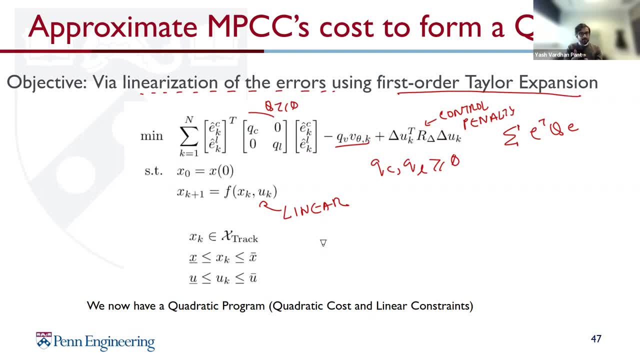 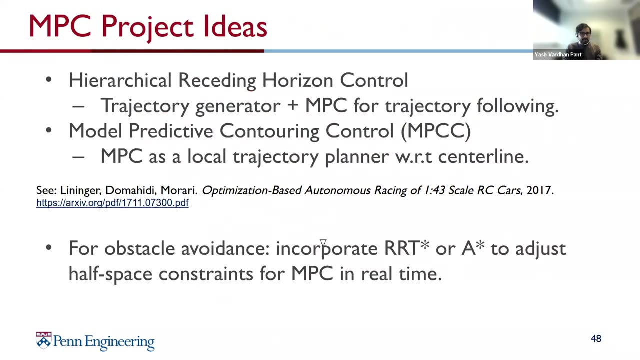 of uh candidate trajectories, you essentially create the best one that's closest to the center line, making progress along it, and you're respecting your constraints as well. and with some approximations and linearizations, you can turn this into a quadratic program to be solved. so that's what model predictive controlling is, contouring control is. 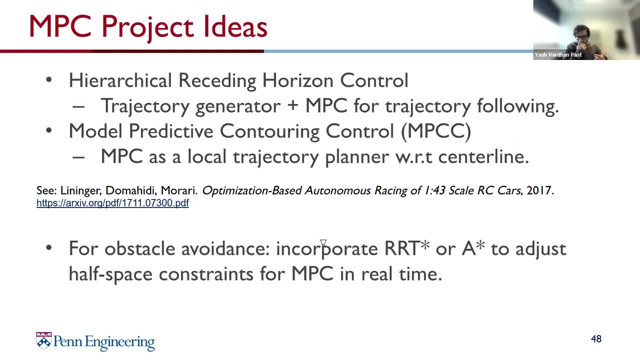 higher level trajectory generator plus mpc that only does trajectory following, plus safety. second is mpcc. that is where the mpc now acts as a local trajectory planner and also does uh control on your own. so look at the reference for more details on both of these methods. i think you might. 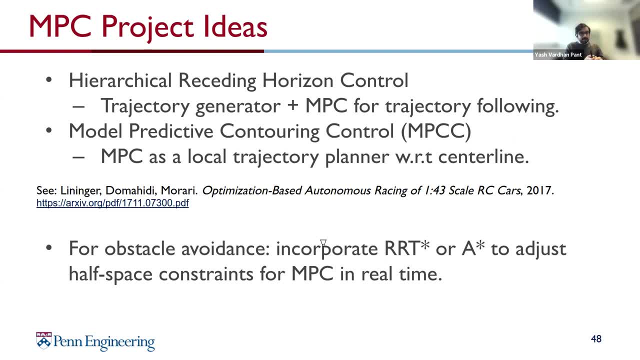 be implementing one of these in the class uma, mpcc, not entirely sure. If you want to take into account things like obstacle avoidance at your high level trajectory generator, you can use RRT star or A star to adjust these half space constraints that you're going to use as X track. 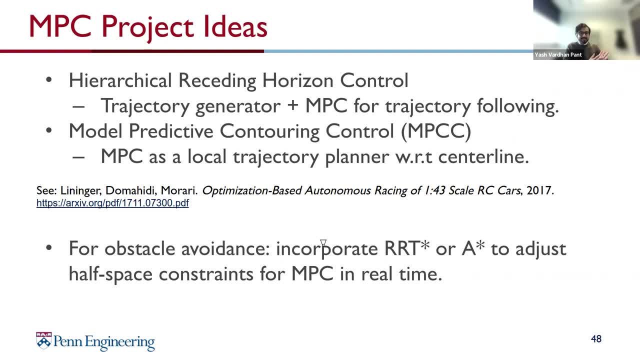 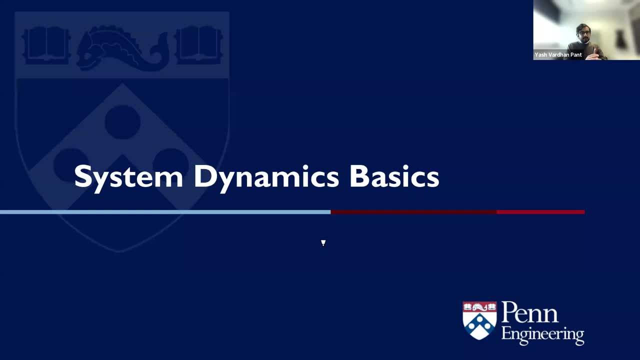 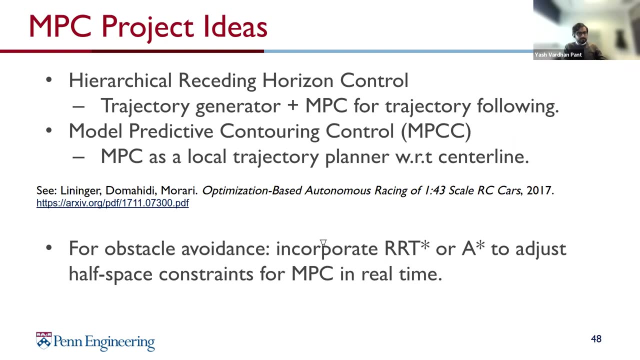 or your constraint set for X in your MPC, So you can use these kind of other approaches to guide your MPC as well. OK, so before we dive into the basics, any questions about that? Yeah, there's a question. In one of the slides you said that the track constraints 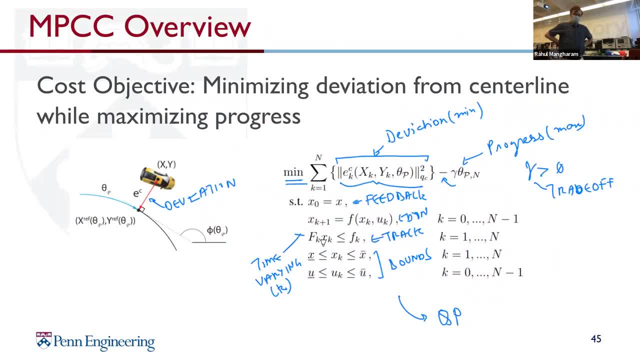 were time-based, And my question is: wouldn't they be more state or space-based? Because if the track doesn't change with time, it changes based on where you are in the track. So I was wondering if there's a way to formulate that properly. 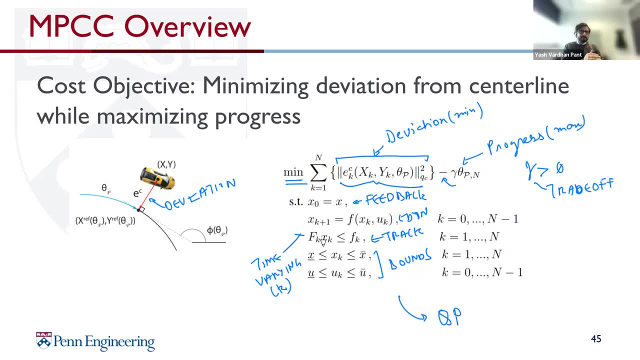 or maybe more intuitively. That's a good point. So they are going to be state-based, like you suggested. If they're a function of the state, then it's usually a nonlinear constraint, which is you want to then approximate it by something simpler. 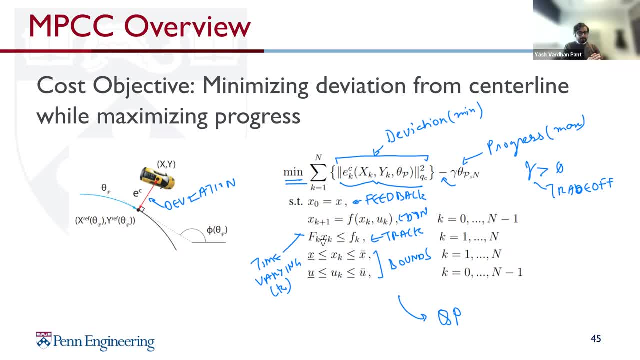 So, which is why you, instead of using a state-based constraint, you'll kind of do some approximation of it, usually an under-approximation of those constraints, such that you can turn it into a time-varying. It doesn't have to be time-varying. 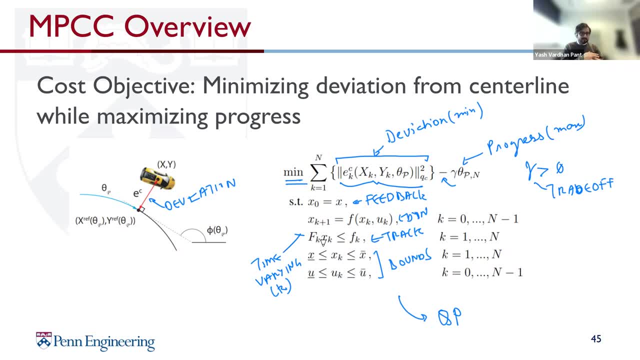 but you'll see, it's usually best given as a time-varying set of constraints to work with. So again, this is all. it may not be all exact, but this is all in the interest of turning it into a quadratic program that you can actually solve. 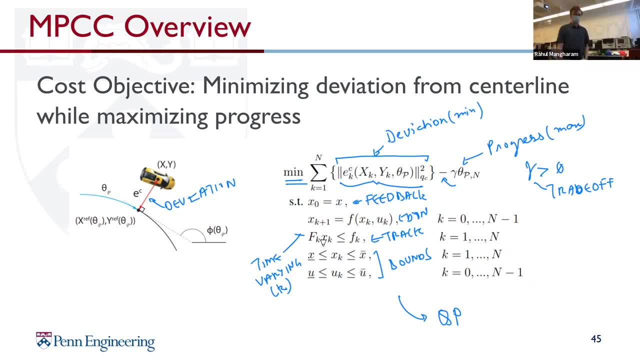 So you want your constraints to be nice and linear. I assume it's explained probably in more detail in the paper. then, Yeah, yeah, The paper will give you some more details on that. Awesome. Thank you Great. Any other questions? 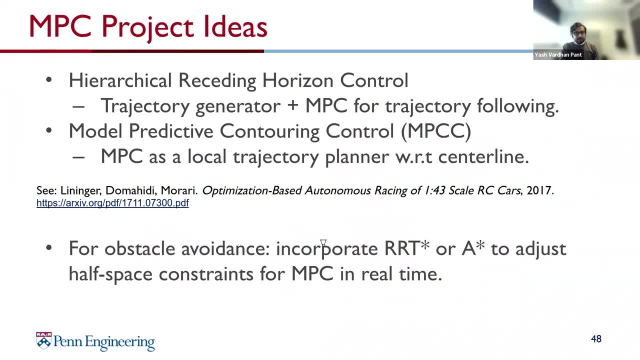 All right, Cool, OK. so yeah, these are two kind of approaches that use MPC for doing racing around the track And again, in the interest of time, we had to speed through this. but more details are in the paper and the paper also has other references. 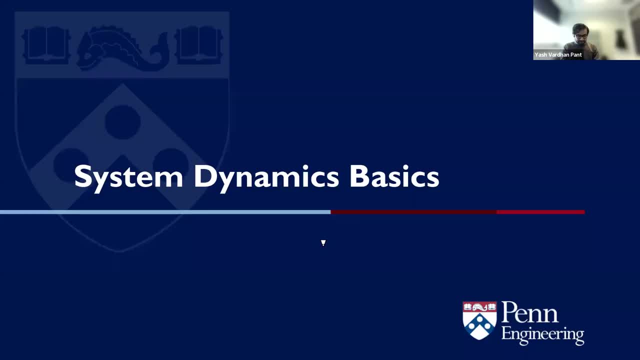 that you can look at. OK, cool. So in the last five minutes let's talk about some of the basics of system dynamics, or why we were using LTI or linear time-invariant dynamics. Again, if you've taken these ESC 500, then 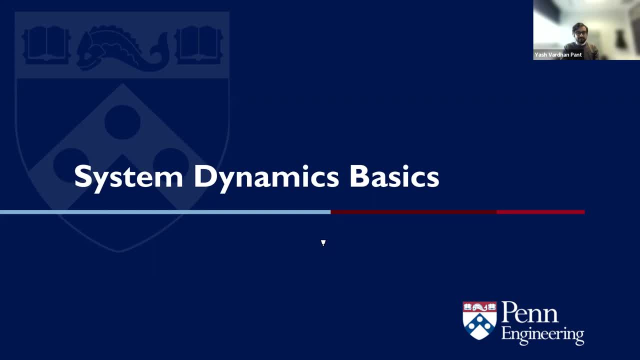 all this will not be news to you, But in case you haven't, it's good to kind of see a little bit about where these system dynamics are, where they come from and how do we represent them in a way that we can throw it to MPC. 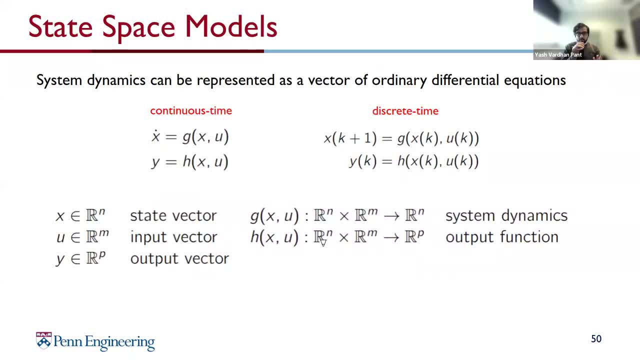 So we use what we call state-space models or where we're talking about the evolution of a state over time. So you have some vector-valued state. The time evolution of that or x dot is given by some function: g of the state, x and the x dot. 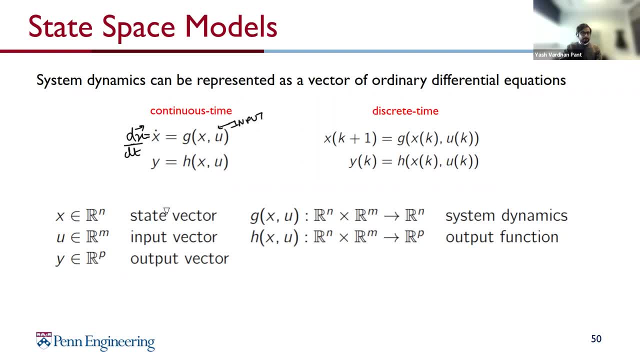 So let's go ahead and see it, OK. input U: The state, for example, for U could represent the position, velocity, acceleration, angular accelerations, orientations of your car. Inputs could be steering throttle or whatever else you're using. 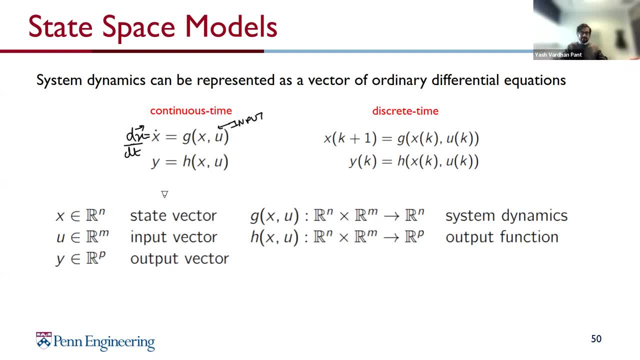 And so the evolution of how the state is going to change over time, as a function of the state right now and the input that you're applying right now. this can be written down as a set of, or a vector of, ordinary differential equations, And we call this a state-space model. 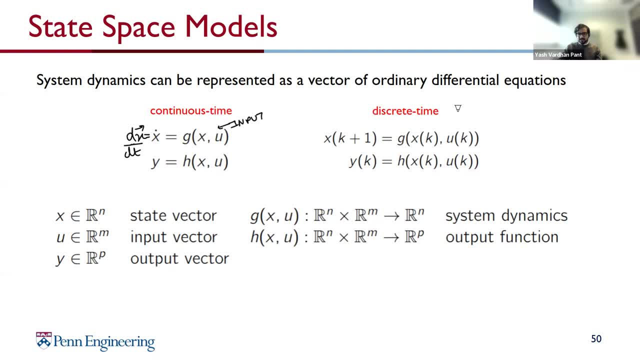 Now, if we're talking about continuous time, then you have differential equations, But we want to again, instead of working with a differential equation, we want to work with a difference equation for discrete time, Because, again, we want to write a finite number. 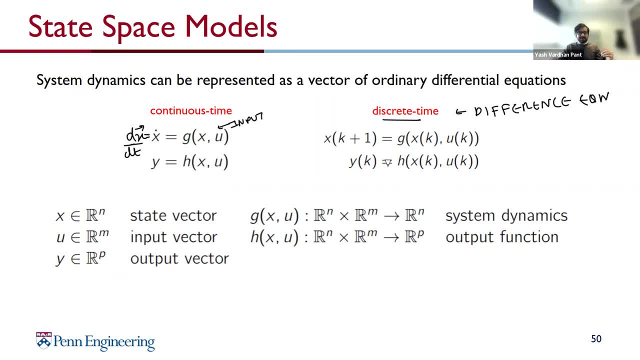 of constraints for our state at time- step 1, time step 2, and so on for our MPC. So we'll work with the discrete time version of it. Again, you have discrete time. You have time-state-space models. They could be nonlinear, as shown over here. 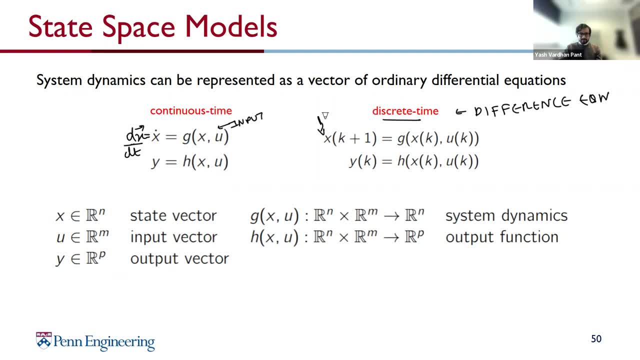 You could have a state evolution model xk plus 1, which is the next state as a function of the current state xk and the current input uk. If you've taken a machine learning class, think of this as a deterministic Markov decision process. 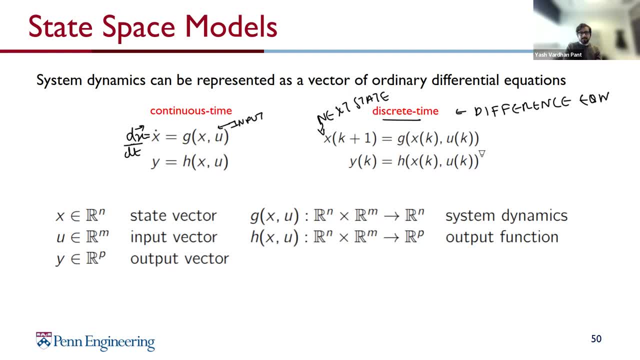 or a continuous valued state and inputs, for example, And so you have this kind of representation of your discrete time system. You could also have an output or a measurement from the state, For example for your car. you won't maybe have access to all your orientation to begin with. 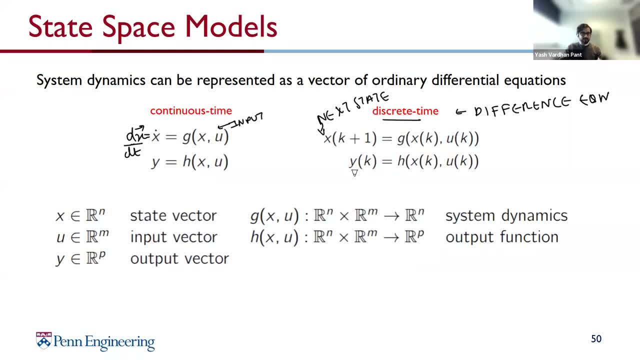 You will only have access to some derivatives of that And then you have to pass that to some state estimator to get the actual orientation or the pose of the car. So y is a measurement which maybe masks some of the inputs or gets a linear combination or whatever, of some of the states. 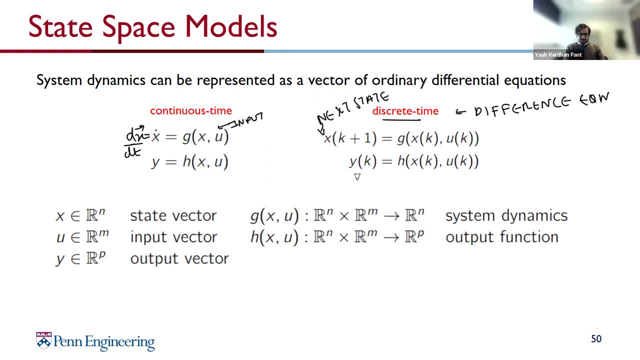 and so on. So we'll care about state-update equation. mostly We won't worry about the output. But yeah, If you wanted to write an output tracking MPC, you could do that as well by using an output function, usually just a matrix that masks the right states. 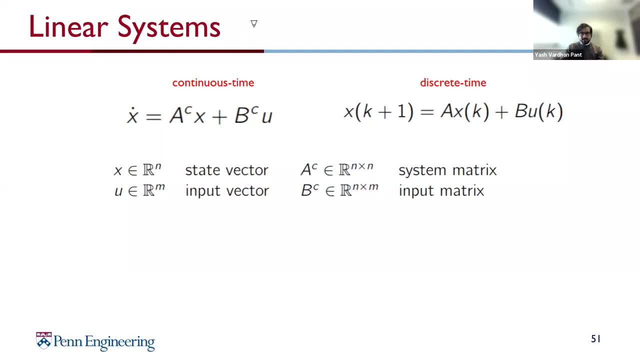 What we'll focus on are linear systems, in particular linear time invariant systems, So LTI or linear time invariant. And what time invariant means is that the A matrix and the B matrix- over here For both discrete time and continuous time, are not changing over time. 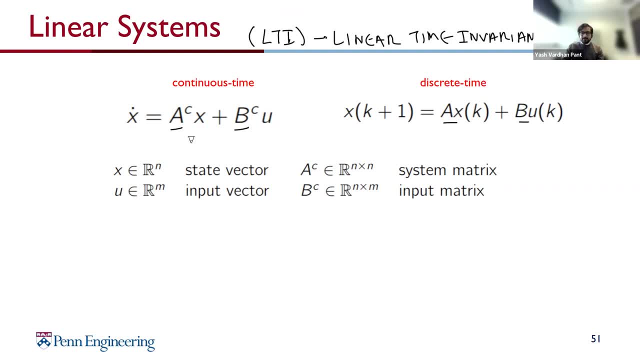 So your dynamics at any point in time is going to be the same. So that's what LTI systems are And again, these are the easiest type of systems you can throw to MPC. You could also use linear time varying systems or LTV systems. 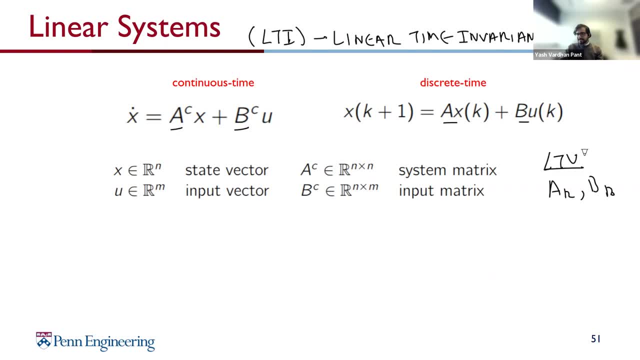 where A and B are indexed by k, for example. So that's another class of linear systems more general Can also be used in MPC, but lose some of the stability and feasibility guarantees. So again, LTI systems are what you want to use more often. 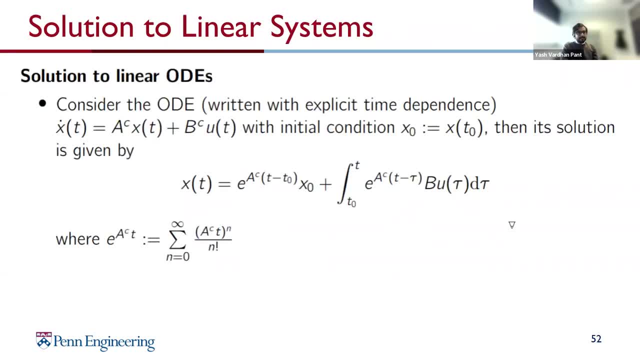 than not. When you talk about the ordinary differential equations, you're talking about the time evolution of states, So you also want to talk about what is the actual state that I have, And we can essentially this following a solution to ordinary differential equations. 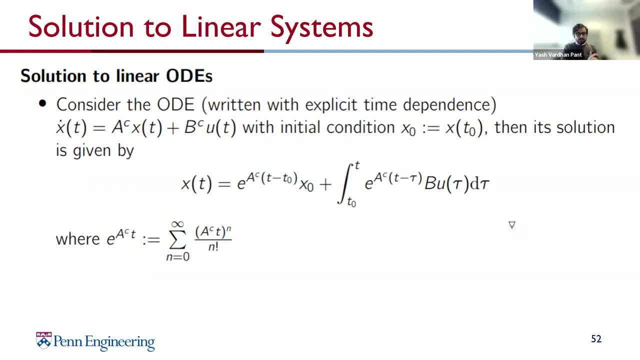 I don't think there's any point getting into it too much, But one thing to note is that this can be used in many ways. For example, for linear systems. we can use the same solution to the linear ODE And if you have a continuous time system, 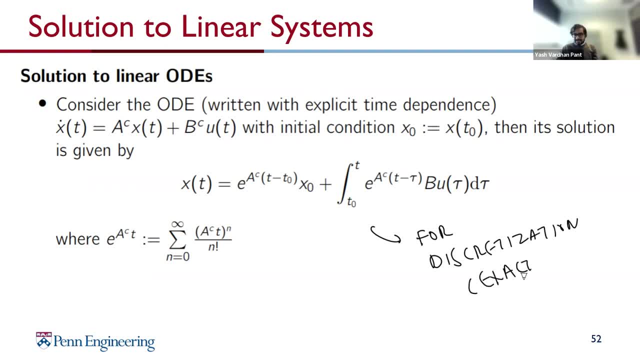 you can use this solution for discretization in time And usually for linear systems. we have this property called exact discretization. That is, if you have a continuous time system and you discretize it using this solution to the linear ODE, you have behavior where at each of the sampling points, 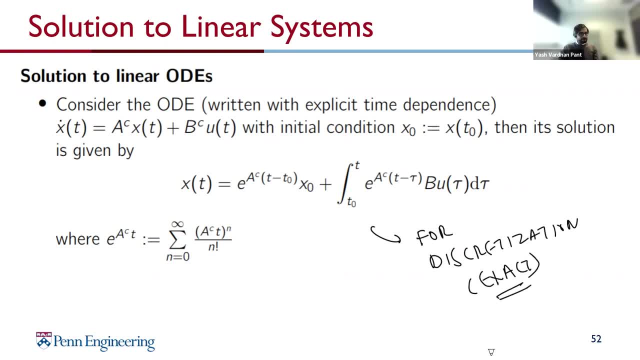 for the discrete system, the state for the discrete system, you have a linearization And you can do that Again. MATLAB can do that for you, for example. So, again, this is the only place where I think the solution to linear ODEs is going to be useful. 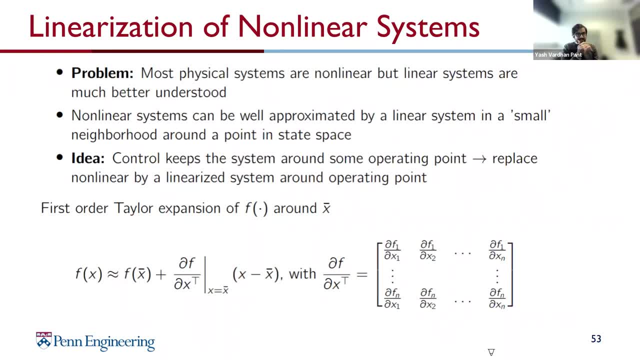 Most systems, of course, are nonlinear. If you try to work out any dynamics from first principles, write down the physics of your car, for example, end up with a bicycle model. it's a nonlinear system, nonlinear in your state and inputs. 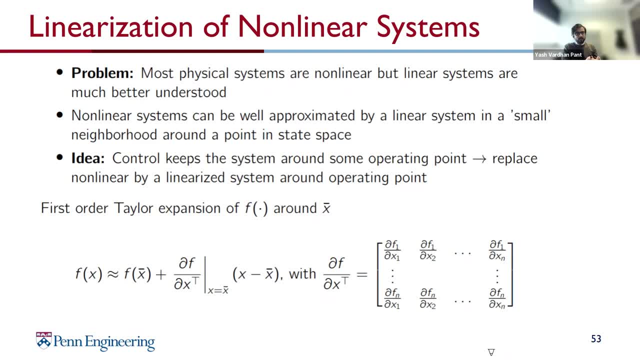 But again, we want to have an MPC that has only linear constraints. So what we'll do is we linearize The system, and usually nonlinear systems can be approximated by linear systems in a small neighborhood, especially if nonlinear systems are not chaotic or unstable. 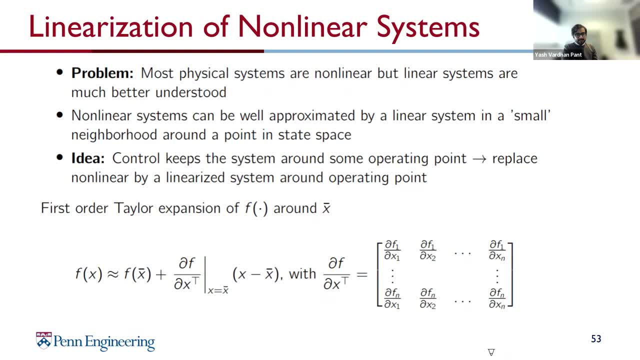 Then you can get away with linearization in more than a small neighborhood. But the idea then is to come up with controls that keep you in a small neighborhood of your operating point And then you can switch your operating point and do successive linearization based on where. 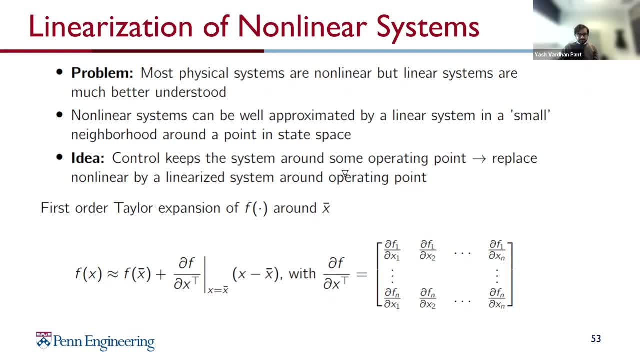 you are in the state space, In order to get our essentially to go from say xk plus 1 is equal to, let's say, some g of xu to our LTI system, which is xk plus 1 is equal to some axk. 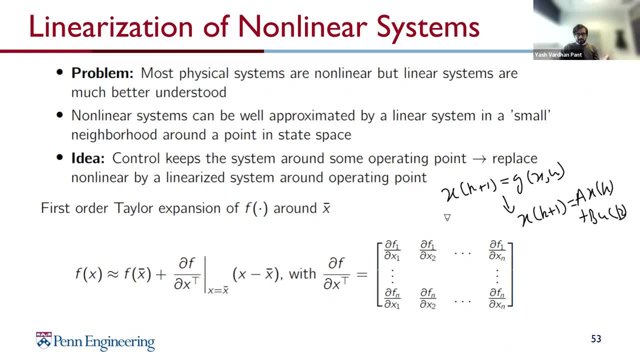 plus buk. what we're going to use is Taylor approximation And again, this is something you might have studied in some other classes, so I won't spend too much time on that, But essentially it's these kind of Jacobians that you'll be computing, which is the partial derivative. 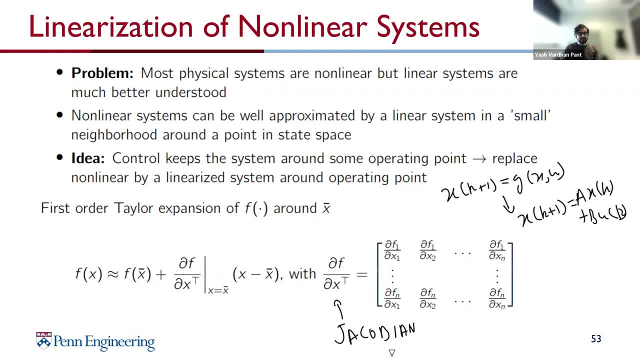 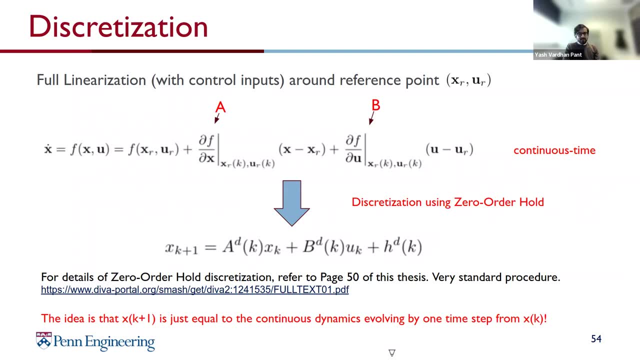 of each element of g or f with respect to each element of the state Or the input, And that's going to give you the A and B matrices. So, essentially, you can get linearization of your system by taking your ODE, applying your first order, Taylor. 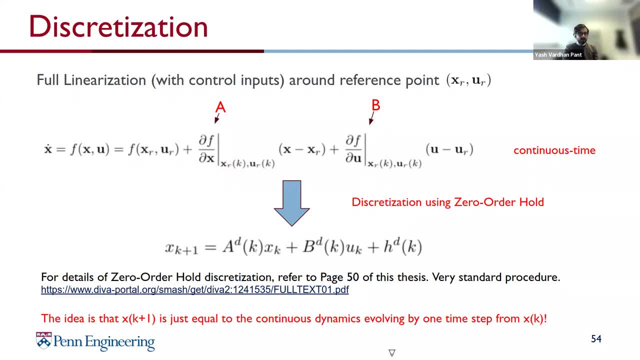 approximation to it, as shown over here, ignoring your higher order terms given to the first order ones, And then you can convert that to, of course. the second step over here would be you would get an x dot as some acx plus bcx. 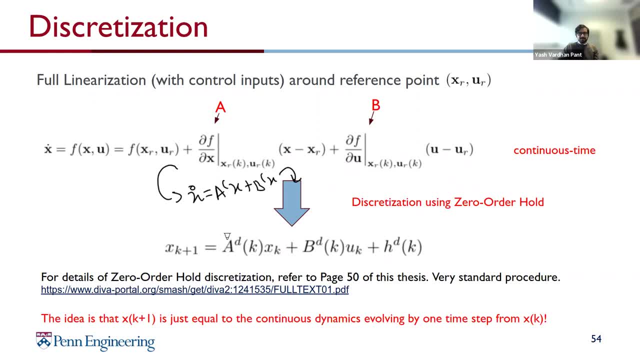 The next step would then be discretize it, Using either zero-order hold or, preferably, using exact linearization, because you're going from linear system to linear system And then what you have is an LTI system that you can throw to most MPC solvers to work with. 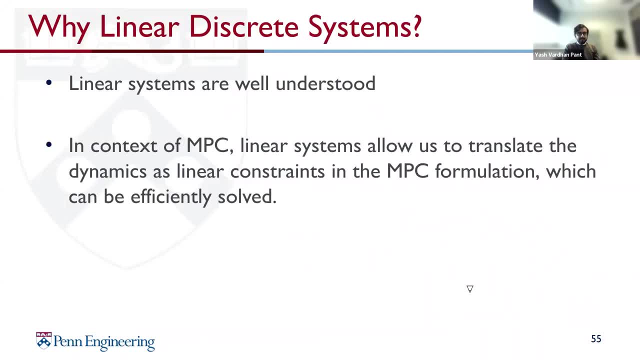 Yeah, so I think that pretty much covers everything about your system dynamics that you should care about, And the reason why we use linear systems is that they are well understood. We have well-known notions of the system: controllable other states observable. 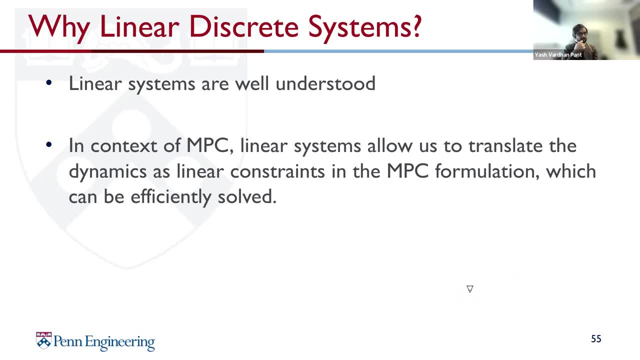 That is, can you estimate the full state given a measurement or can you move your state to wherever you want it, which is just controllability And, in the context of MPC, linear systems give you dynamics and constraints that you can efficiently formulate. 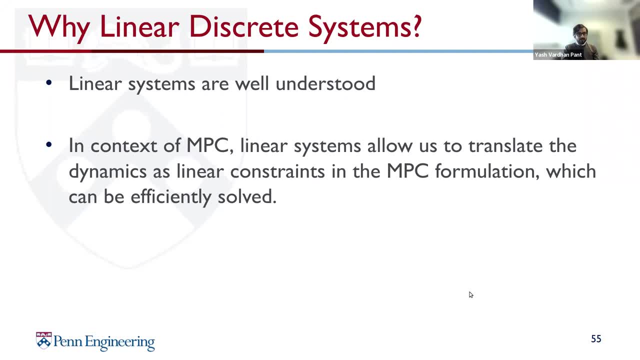 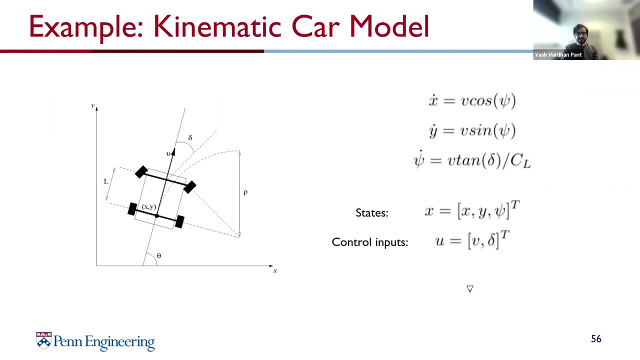 the linear constraints. So it's going to make your life a lot easier when you use MPC. An example is, let's say, non-holonomic car kinematics as shown over here with three states. Again, we'll get too much into that. 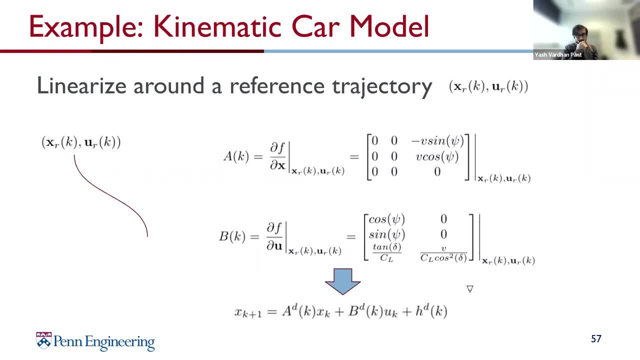 but, given a reference trajectory, you could linearize it By computing the right Jacobians for the A and the B matrix and you'll end up with a linear time invariant system once you discretize this in time. So anyway, these are the kind of things. 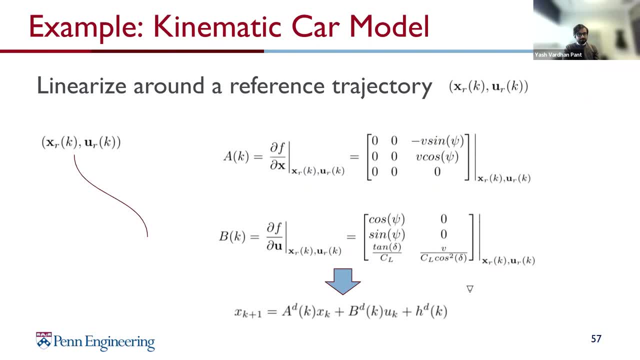 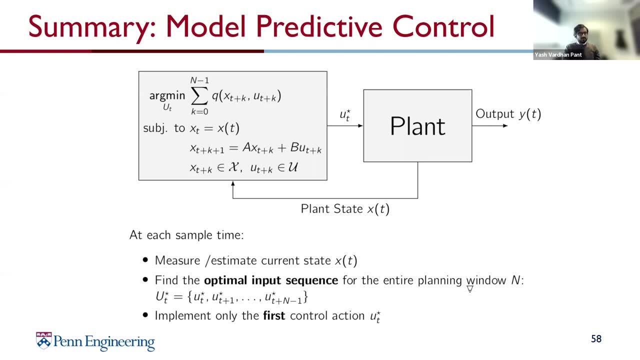 you'll do on the inside when you start to implement MPC. But yeah, long story short. these are kind of things you'll linear models of what you're going to use. So, to summarize, MPC is an optimization that's working in the loop with your dynamical system. 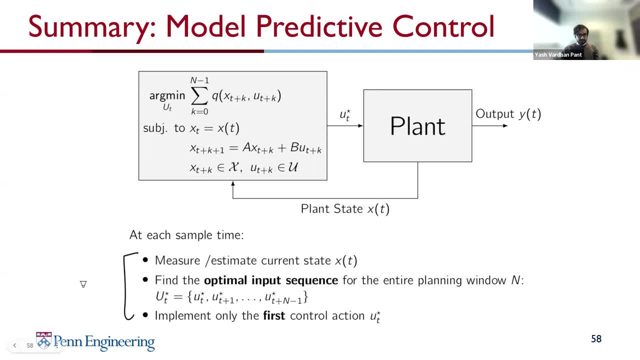 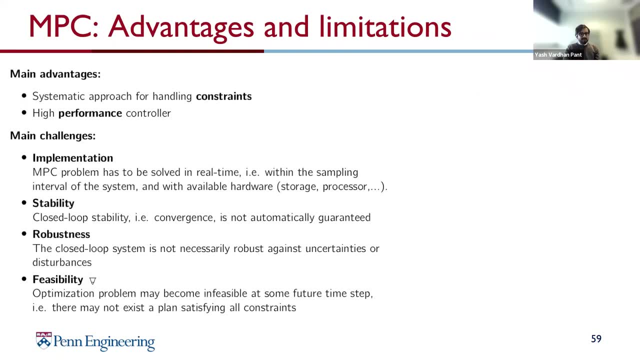 You're going to apply it in a receding horizon manner, which is kind of the same, This whole thing. So that's how you turn your open loop optimization into closed loop control, And MPC gives you a bunch of advantages, That is, it allows you to handle constraints very naturally. 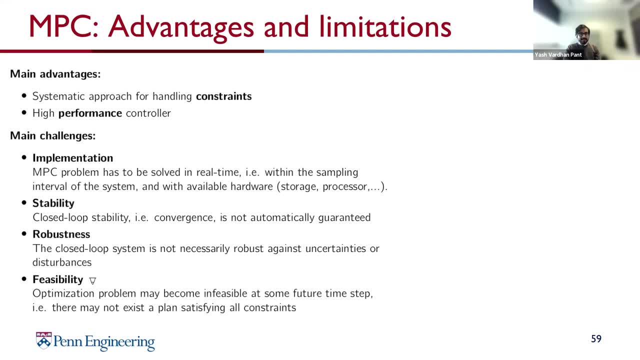 especially if they're linear, Gives you controllers that also have optimality guarantees. You'll have, of course, challenges on implementation, like: how fast can you use this? Someone raised the question in class and that was a good question. You will kind of run into some implementation issues. 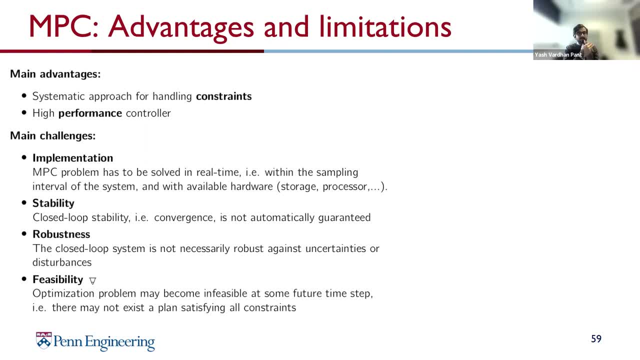 Guarantees on stability, robustness, feasibility. those are usually hard to get from MPC unless you do some special, complex tricks, which again are way beyond the scope of this particular course. But there are methods that allow you to do that as well. 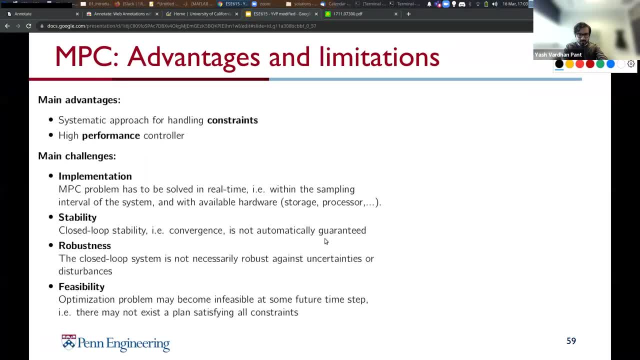 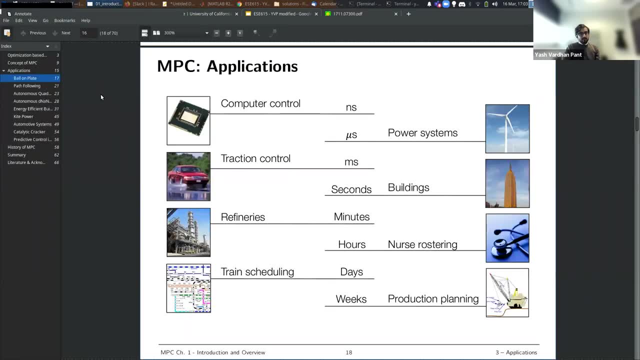 So, yeah, I think that'll summarize MPC. And let me give you one last thing to talk about over here, which is MPC is not just for autonomous racing. It has applications all over, whatever you can imagine from computer control, where you need to have update rates in the order of nanoseconds. 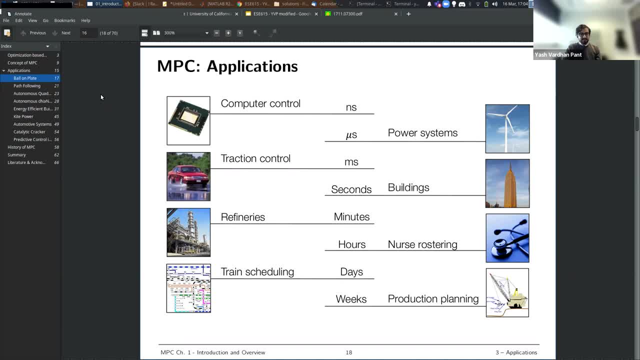 to power systems. So you're trying to do voltage or frequency control with microseconds, or even for things like train scheduling, production planning or smart control of buildings, where your update rates could be of the order of hours, days or even weeks. 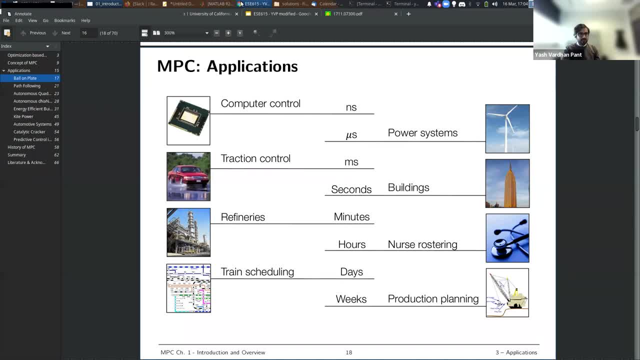 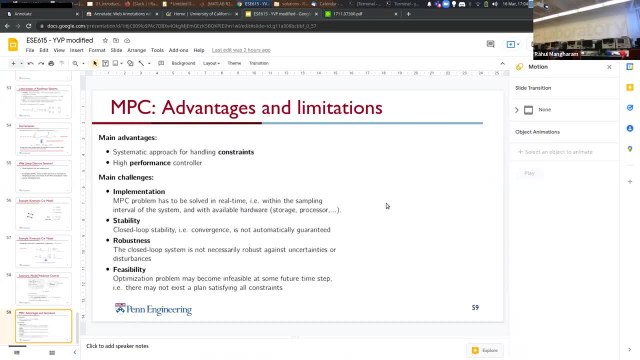 So, yeah, with that I'll end the lecture And let's take any questions if you have, if there's time remaining, Rahul, Sure, any questions. I think that was a lot of material. Yeah, Yeah, We basically passed the MPC course and some. 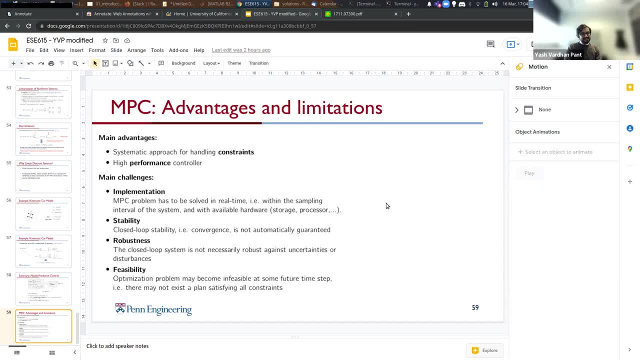 of the linear systems course all in one lecture, But I think this gives you a good start. You basically have a mental framework of how to get started. We'll review the MPCC paper and then get into the details, And we'll also give you a skeleton framework. 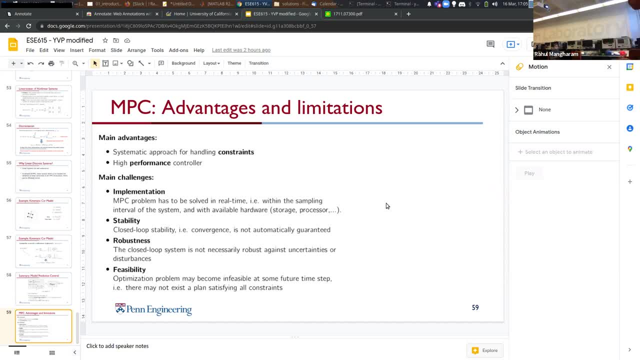 You're not starting from scratch. We don't expect you to have taken the MPC course to solve this right, So we will help you along the way. But thanks so much, Yash. I think this was really great. Thank you everyone. 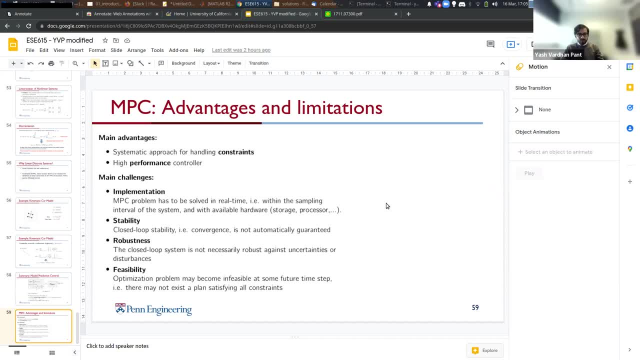 And, yeah, treat this as more of a high-level introduction to what all could have happened. For the details, you'll have to take deeper dives on your own, I suspect. So, yeah, I think the reference for the MPCC paper is going to be useful. 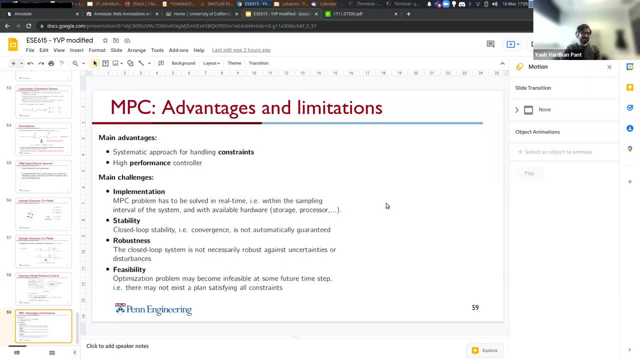 But also, Rahul, if you want, I can send some references on linear systems, But I think that probably won't be required for the class, especially if you tell what the system dynamics are going to be. Yeah, that would be great. 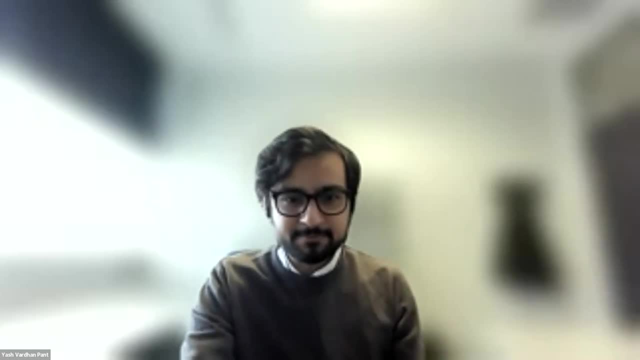 Cool, Thank you. Stop sharing then. Thanks, Rahul, Thanks everyone.